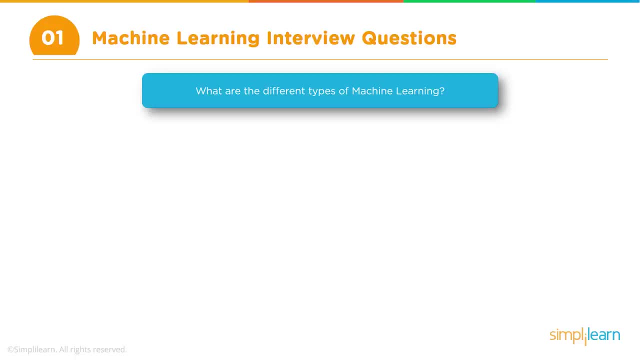 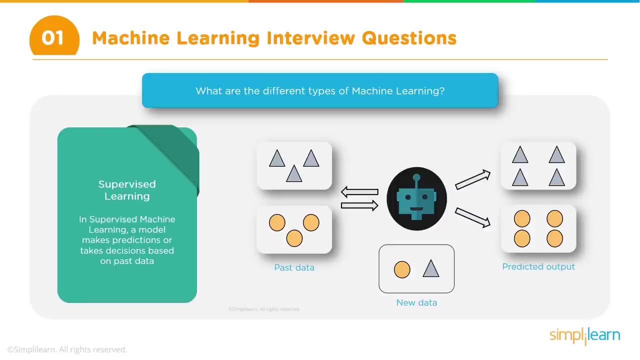 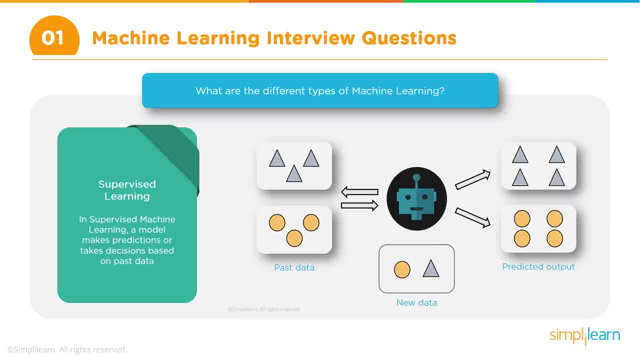 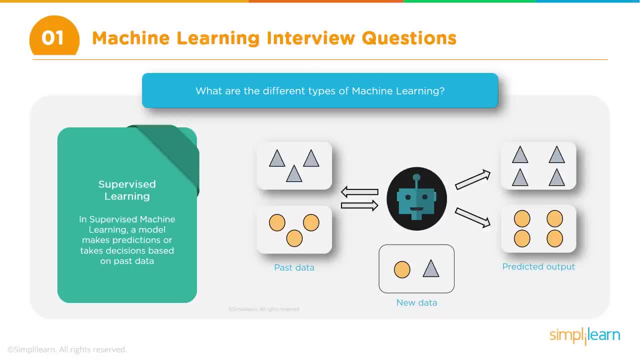 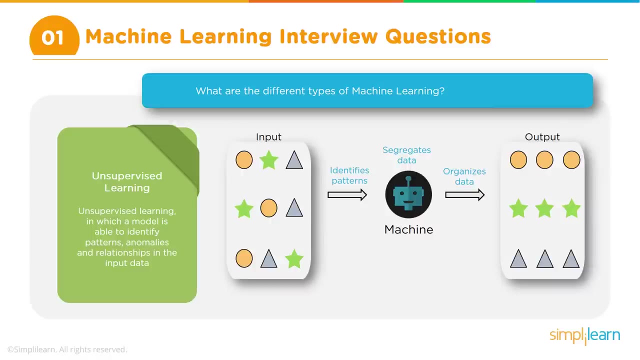 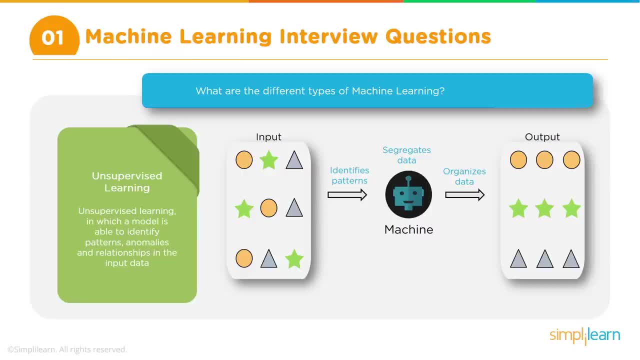 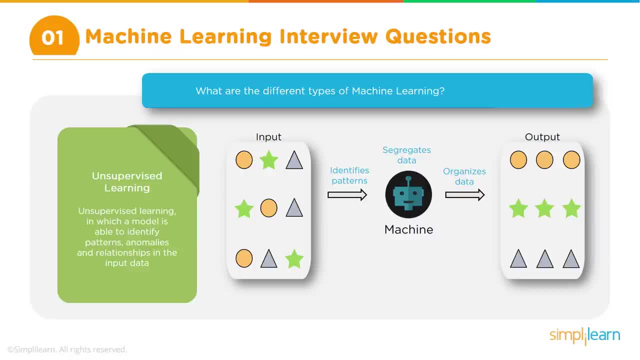 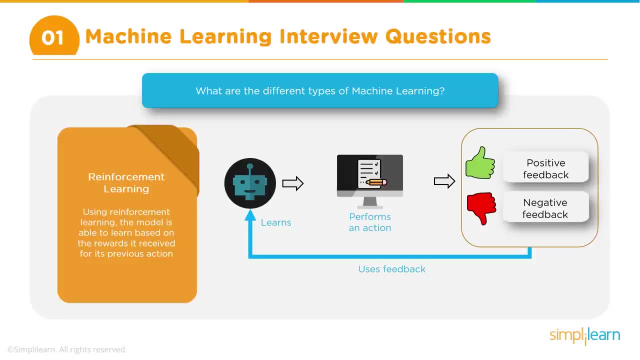 And of course I think there is a different question for that. We will see that later. Then the third: so we have supervised, then we have unsupervised, and then reinforcement. You need to provide a little bit of information around that as well, because it is sometimes. 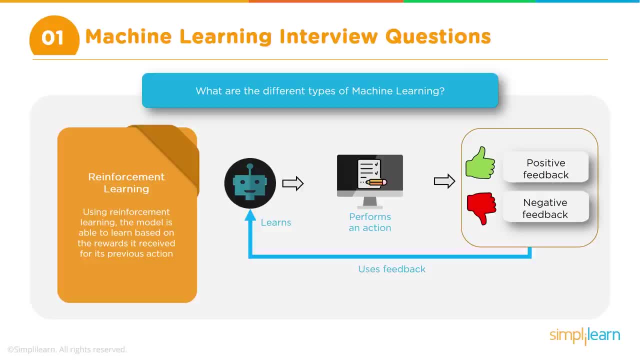 a little difficult to come up with a good definition for reinforcement learning, So you may have to a little bit elaborate on how reinforcement learning works, right? So reinforcement learning works in such a way that it basically has two parts to it. One is the agent and the environment and the agent basically is working inside of this. 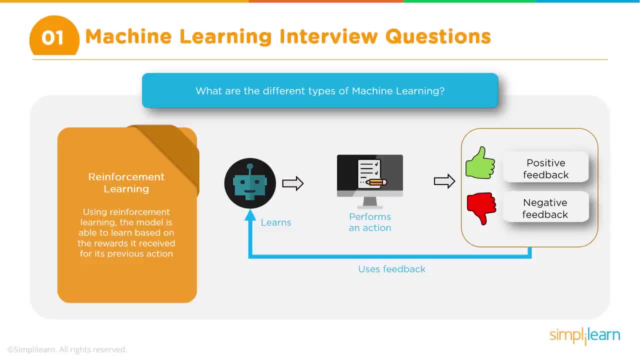 environment and it is given a target that it has to achieve And every time it is moving in the direction of the target. so the agent basically has to take some action And every time it takes an action which is moving the agent towards the target right. 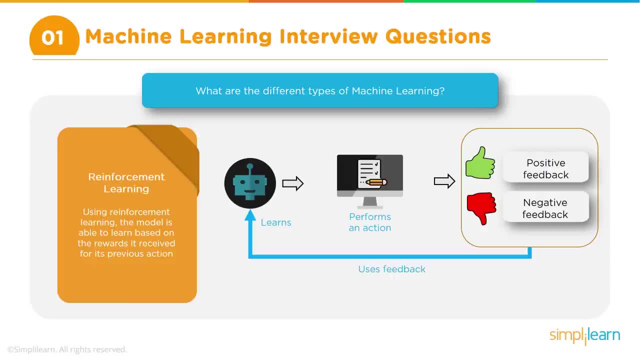 towards a goal. a target is nothing but a goal. okay, Then it is rewarded, And every time it is going in a direction where it is away from the goal, then it is punished. So that is the way you can a little bit explain. 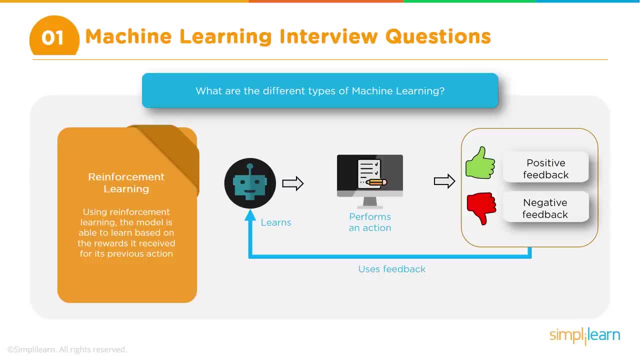 And this is used primarily or very, very impactful for teaching the system, to learn games and so on. Examples of this are basically used in AlphaGo- You can throw that as an example- where AlphaGo used reinforcement learning to actually learn to play the game of Go. 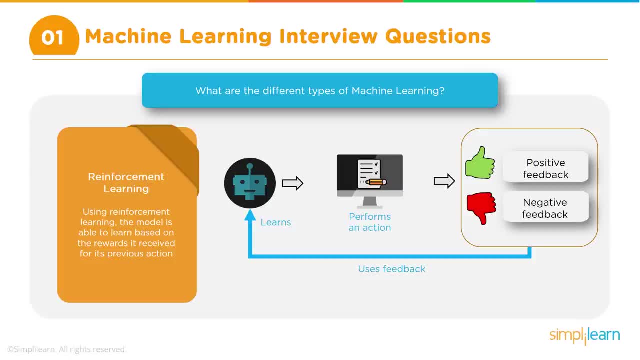 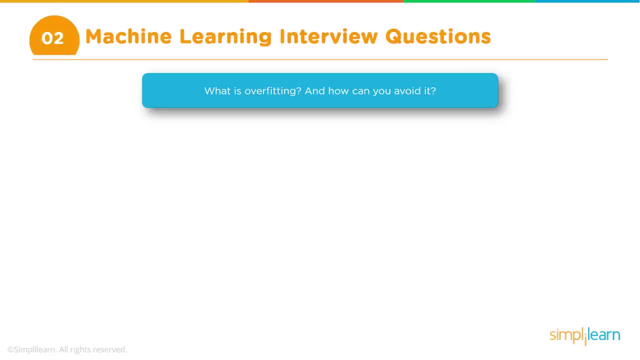 And finally it defeated the Go world champion. right, This much of information. that would be good enough. okay, Then there could be a question on overfitting. So the question could be: what is overfitting And how can you avoid it? 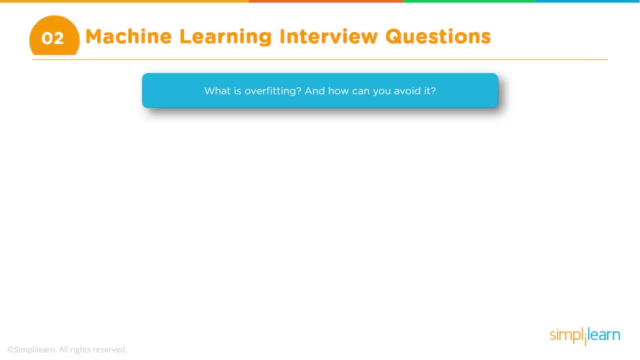 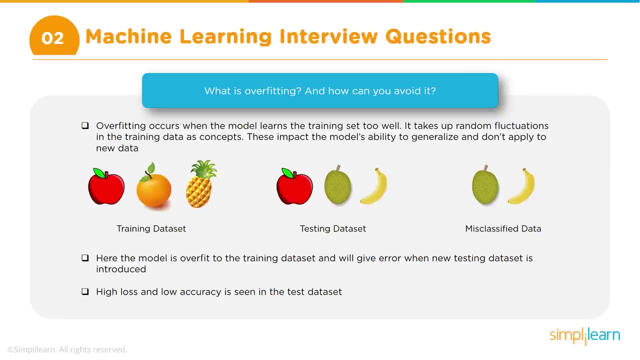 So what is overfitting? Let's first try to understand the concept, because sometimes overfitting may be a little difficult to understand. Overfitting is a situation where the model has kind of memorized the data. So this is an equivalent of memorizing the data. 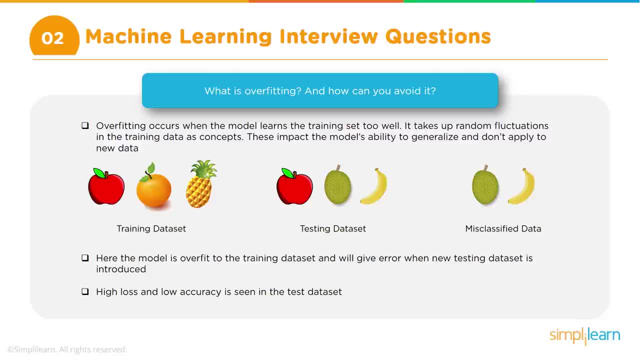 So we can draw an analogy so that it becomes easy to explain this. Now, let's say you're teaching a child about recognizing some fruits or something like that. okay, And you're teaching this child about recognizing, let's say, three fruits: apples, oranges. 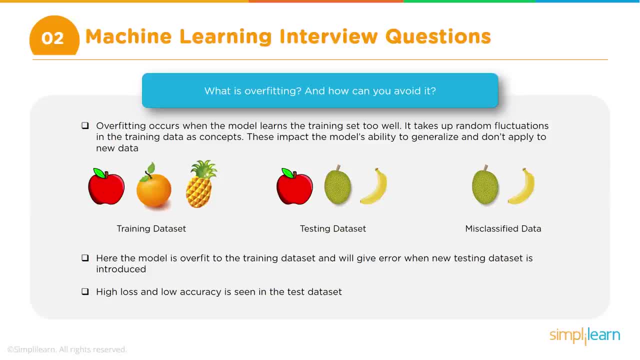 and pineapples. okay, So this is a small child And for the first time, you're teaching the child to recognize fruits Then, so what will happen? So this is very much like that is your training data set. What you will do is you will take a basket of fruits which consists of apples, oranges, 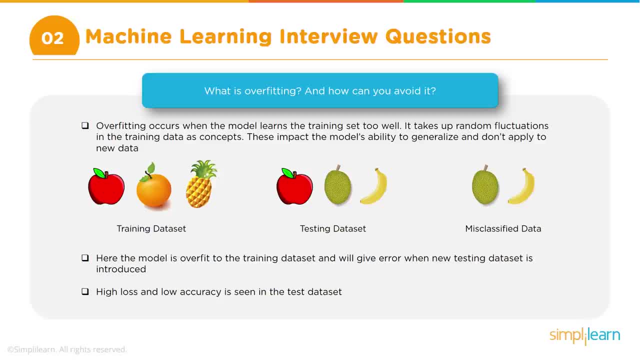 and pineapples, okay, And you take this basket to this child and there may be, let's say, hundreds of these fruits. So you take this basket to this child and keep showing each of this fruit And then, first time, obviously, the child will not know what it is. 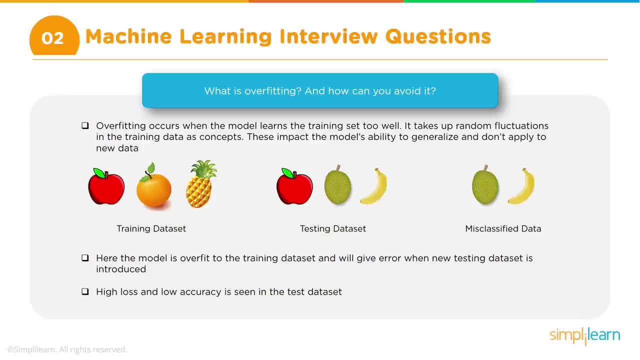 So you show an apple and you say: hey, this is apple. Then you show maybe an orange and say: this is orange, and so on and so forth, And then again you keep repeating that, right So until the That basket is over. 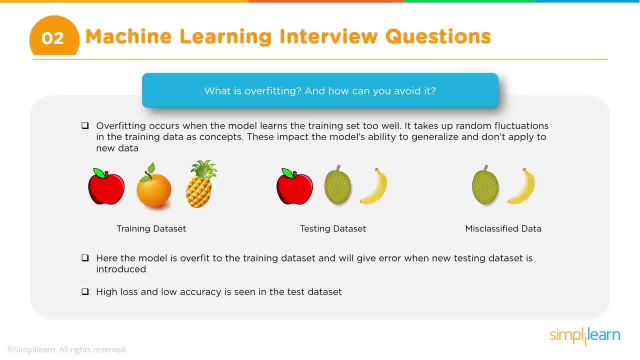 This is basically how training works. in machine learning also. That's how training works. So, till the basket is completed, maybe a hundred fruits. you keep showing this child And then in the process, what has happened? The child has pretty much memorized these. 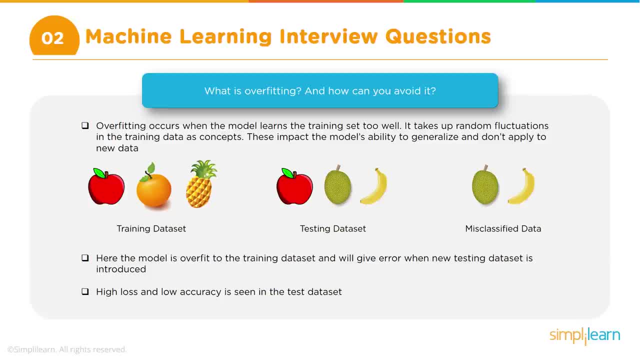 So even before you finish that basket right By the time you are halfway through, the child has learned about recognizing the apple, orange and pineapple. Now what will happen after? halfway through? initially you remember it made mistakes in recognizing, but halfway through now it has learned. 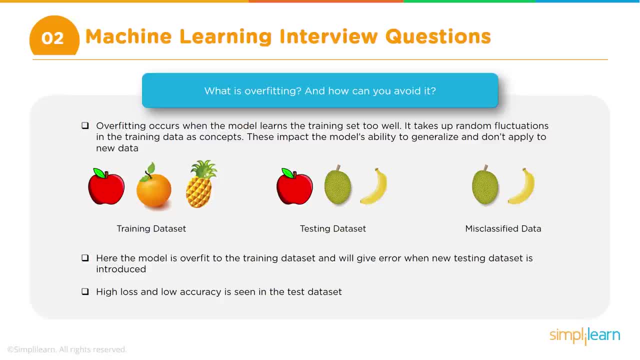 So every time you show a fruit, it will exactly a hundred percent accurately it will identify. It will say the child will say: this is an apple, this is an orange, And if you show a pineapple it will say: this is a pineapple right. 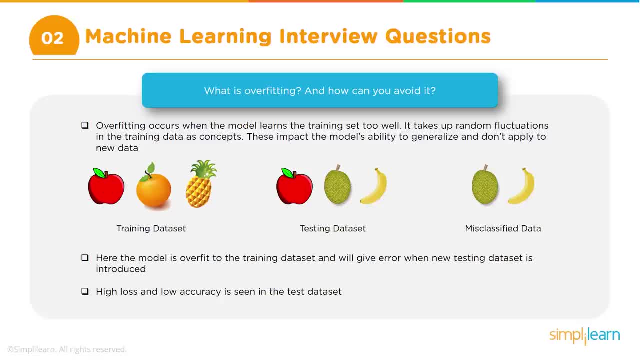 So that means it has kind of memorized this data. Now, let's say you bring another basket of fruits and it will have a mix of maybe apples, which were already there in the previous set, but it will also have in addition to apple, it will. 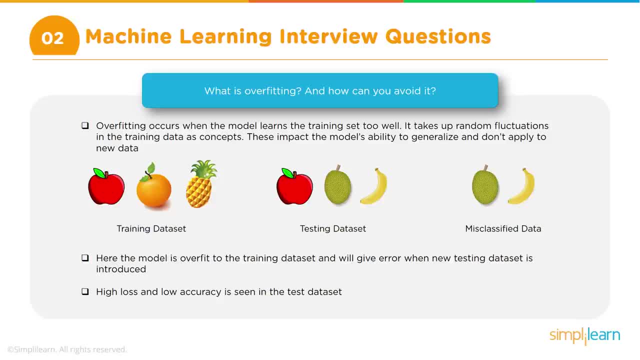 probably have a banana or maybe another fruit like a jackfruit, right? So this is an equivalent of your test data set, which the child has not seen before. Some parts of it it probably has seen, like the apples it has seen, but this banana and 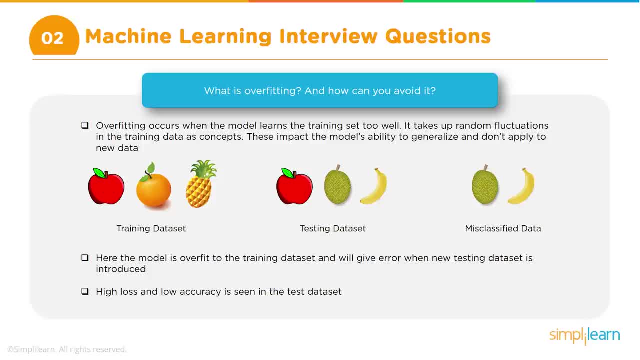 jackfruit it has not seen. So then what will happen in the first round, which is an equivalent of your training data set towards the end? it has a hundred percent. it was telling you what the fruits are right. Apple was accurately recognized. orange was accurately recognized. 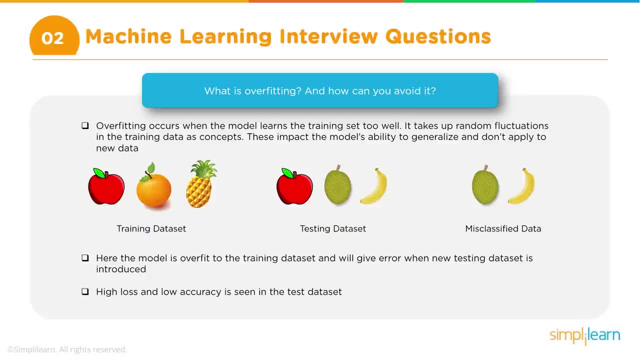 And pineapples were accurately recognized right. So that is like a hundred percent accuracy. But now, when you get another, a fresh set, which were not a part of the original one, what will happen? all the apples maybe it will be able to recognize correctly, but all the others, like the 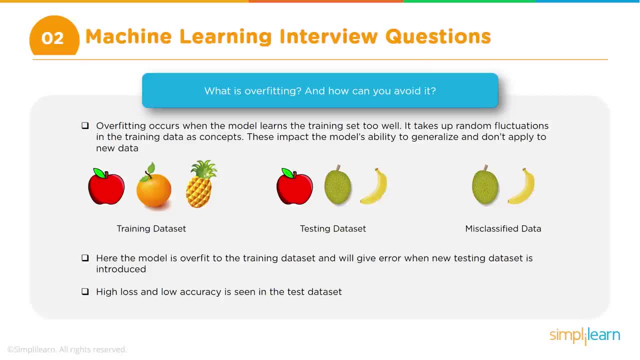 jackfruit or the banana will not be recognized by the child right? So this is an analogy. this is an equivalent of overfitting. So what has happened during the training process? it is able to recognize or reach a hundred percent accuracy, maybe very high accuracy. 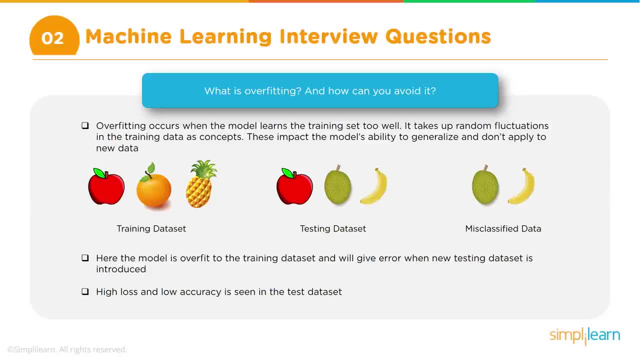 Okay, And we call that as very low loss, right? So that is the technical term. So the loss is pretty much zero and accuracy is pretty much a hundred percent, Whereas when you use testing there will be a huge error, which means the loss will be pretty high. 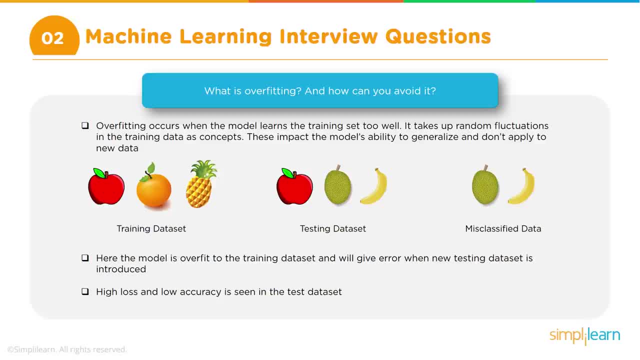 And therefore the accuracy will be also low. Okay, This is known as overfitting. This is basically a process where training is done. Training processes: it goes very well, almost reaching a hundred percent accuracy, but while testing it really drops down. 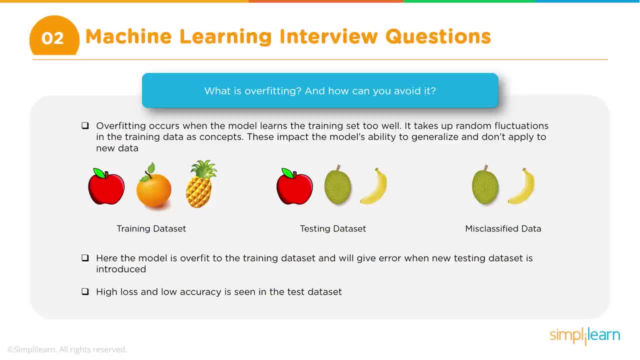 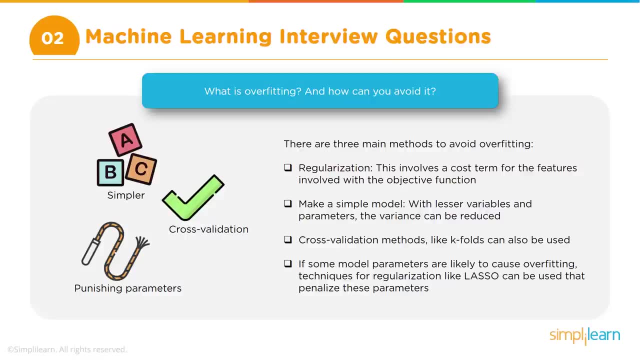 Now, how can you? So? that is the extension of this question. there are multiple ways of avoiding overfitting. There are techniques like what do you call regularization- That is the most common technique that is used for avoiding overfitting- and, within regularization, 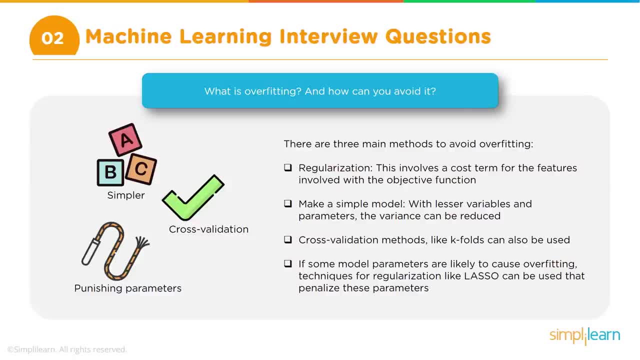 there can be a few other subtypes, like dropout in case of neural networks and a few other examples, But I think if you give example or if you give regularization as the technique, probably you will be able to avoid it. So there will be some questions where the interviewer will try to test your fundamentals and your knowledge and depth of knowledge and so on and so forth. 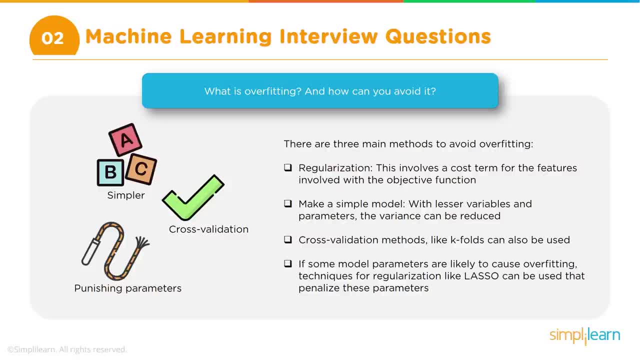 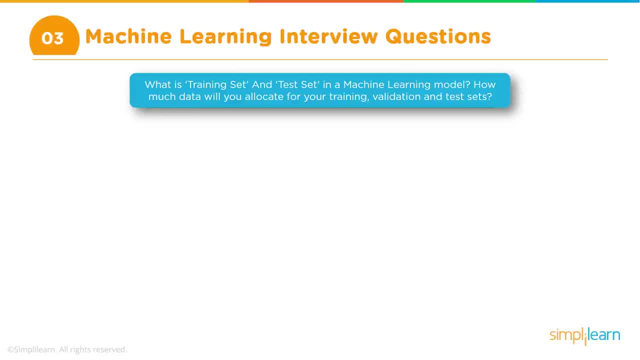 And then there will be some questions which are more like quick questions. that will be more to stump you. Okay, Then the next question is around the methodology. So when we are performing machine learning training, we split the data into training and tests, right? 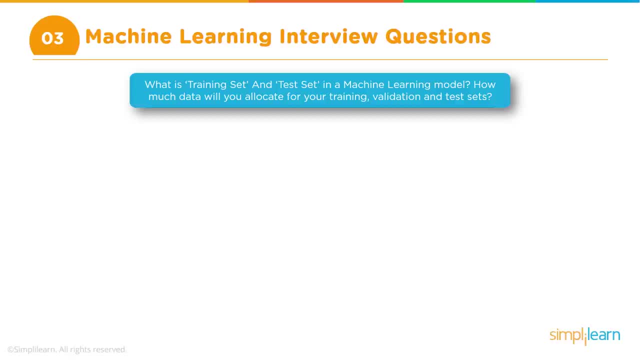 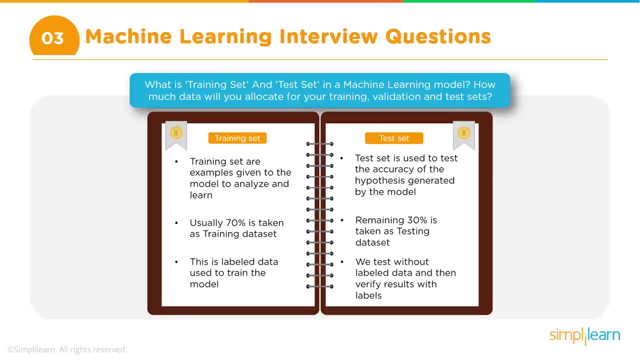 So this question is around. So the question is: what is training set and test set in machine learning model and how is the split done? So the question can be like that: So in machine learning, when we are trying to train the model, so we have a three step process. 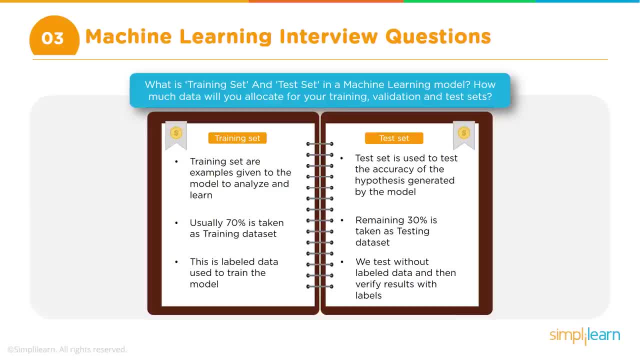 We train the model and then we test the model And then, once we are satisfied with the test, only then we deploy the model. So what happens in the train and test is that you remember the labeled data. So let's say you have a thousand records with labeling information. 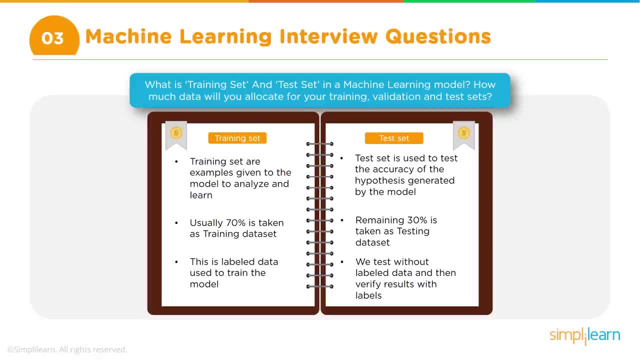 Now one way of doing it is you use all the thousand records for training and then maybe right, which means that you have exposed all this thousand records during the training process, And then you take a small set of the same data and then you say, okay, I will test it with this. 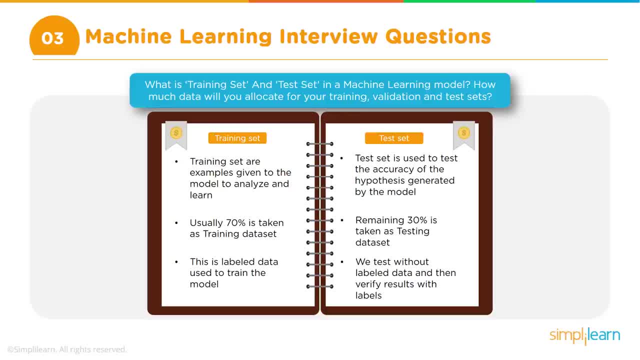 Okay, And then you probably what will happen? You may get some good results right, But there is a flaw there. What is the flaw? This is very similar to Human beings. It is like you are showing this model, the entire data, as a part of training. 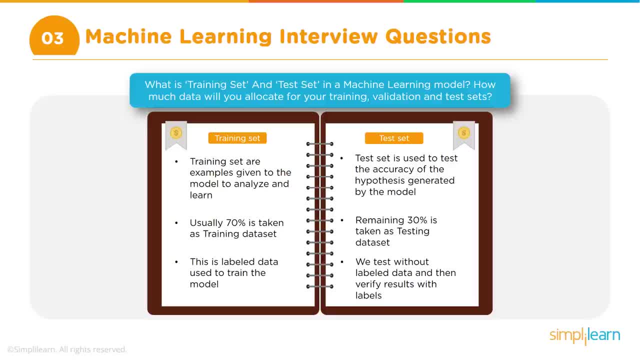 Okay, So obviously it has become familiar with the entire data. So when you're taking a part of that again and you're saying that I want to test it, obviously you will get good results. So that is not a very accurate way of testing. 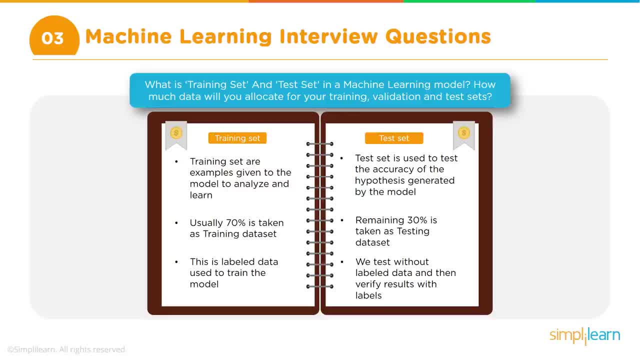 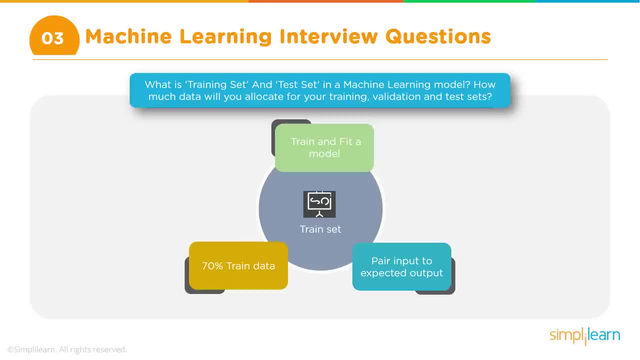 So that is the reason. what we do is we have the label data of this thousand records or whatever we set aside before starting the training process. We set aside a portion Of that data and we call that test set and the remaining we call as training set and we use only this for training our model. 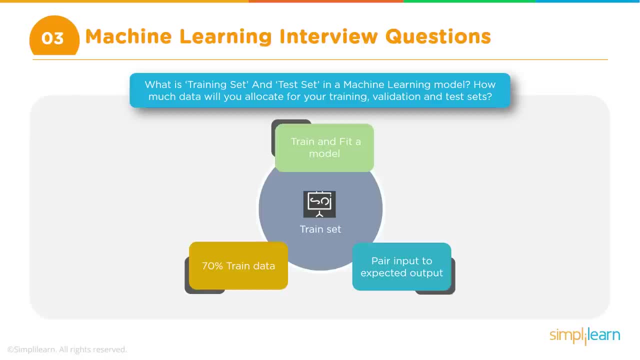 Now the training process, remember, is not just about passing one round of this data set. So let's say, now your training set has 800 records. It is not just one time you pass this 800 records. What you normally do is you actually, as a part of the training, you may ask this data through the model multiple times. 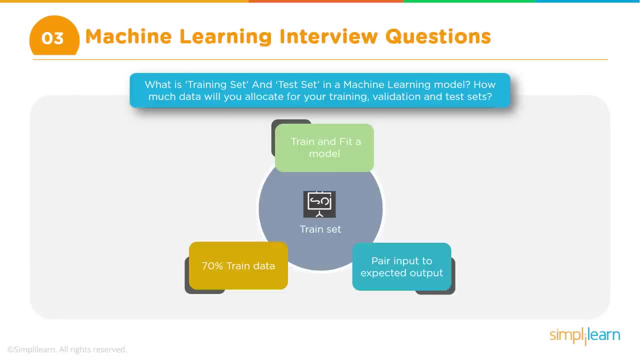 So this thousand records may go Through the model, maybe 10,, 15,, 20 times. till the training is perfect, till the accuracy is high, till the errors are minimized. Okay Now so, which is fine, which means that you are. that is what is known as the model has seen your data and gets familiar with your data. 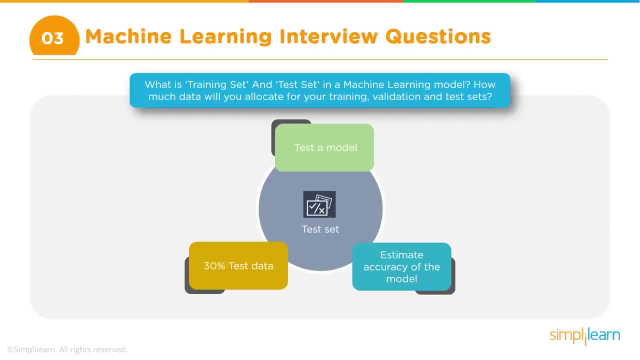 And now, when you bring your test data, what will happen is: this is like some new data, because that is where the real test is. Now you're trained the model and now you are testing the model with some data which is kind of new. 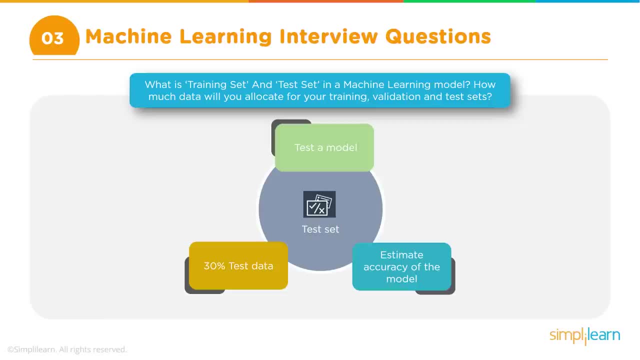 That is like A situation, like like a realistic situation, because when the model is deployed, that is what will happen: It will receive some new data, not the data that it has already seen. Right, So this is a realistic test. 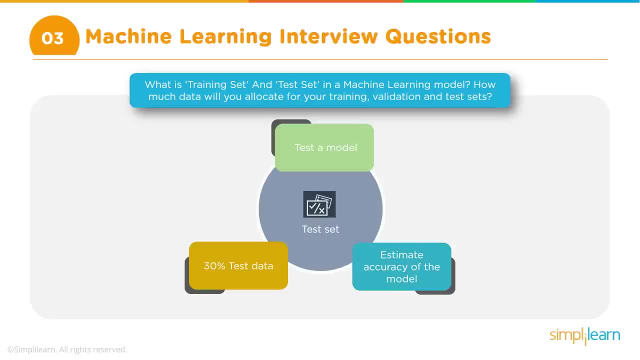 So you put some new data. So this data which you have set aside is for the model. It is new And if it is able to accurately predict the values, that means your training has worked. Okay, The model got trained properly. But, let's say, while you're testing this, with this test data, you're getting a lot of errors. 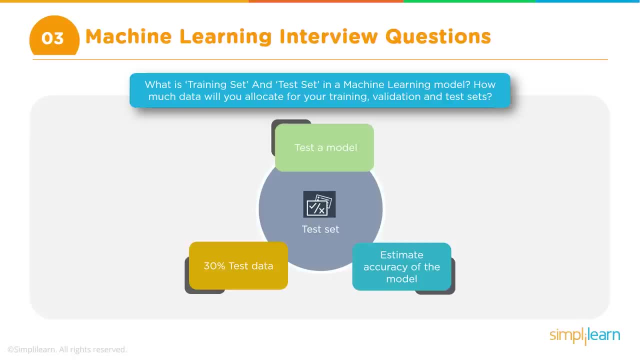 That means you need to probably Either Change your model or retrain with more data and things like that. Now coming back to the question of how do you split this? What should be the ratio? There is no fixed number. Again, this is like individual preferences. 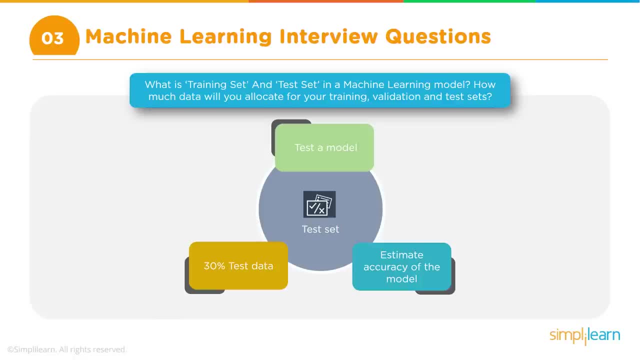 Some people split it into 50, 50, 50% test and 50% training. Some people prefer to have a larger amount for training and a smaller amount for test, So they can go by either 60, 40 or 70, 30, or some people even go with some odd numbers. 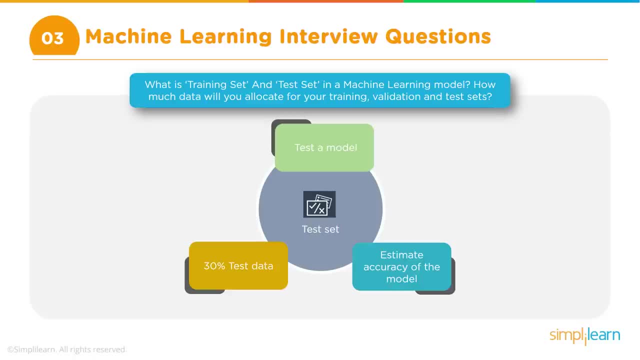 Like 65, 35 or 63.33 and 33, which is like one third and two thirds. So there is no fixed rule, that it has to be something. The ratio has to be this: You can go by your individual preferences. 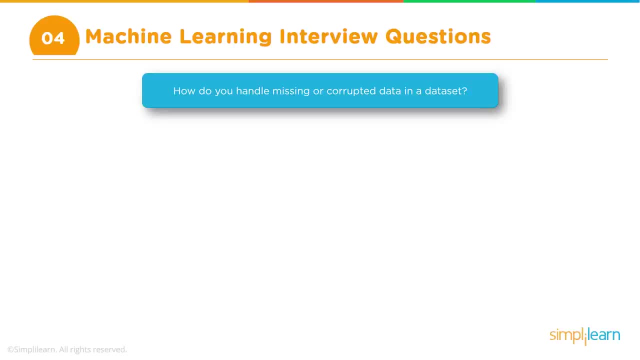 All right. Then you may have questions around data handling, data manipulation or what do you call data management or preparation. So these are all some questions around that area. There is, again, no one answer, one single good answer to this. It really varies. 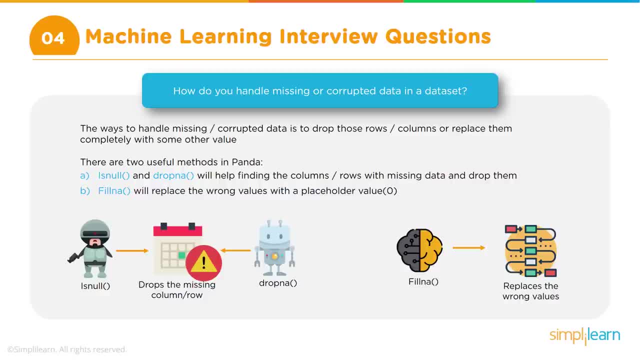 From situation to situation and depending on what exactly is the problem, what kind of data it is, how critical it is, what kind of data is missing and what is the type of corruption. So there are a whole lot of things which is a very generic question. 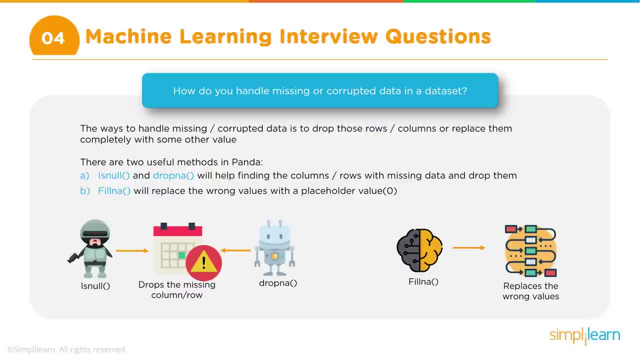 And therefore you need to be a little careful about responding to this as well. So probably have to illustrate this again. If you have experience in doing this kind of work in handling data, you can illustrate with examples. saying that I was on one project where I received this: 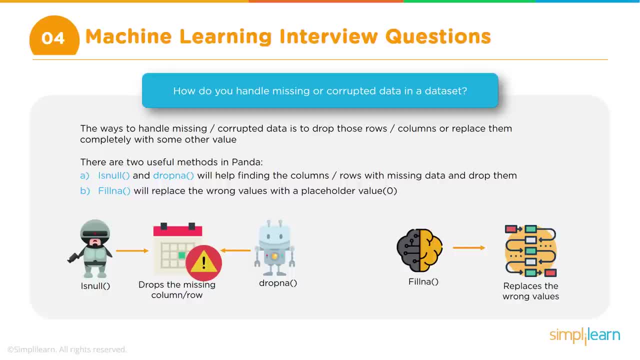 Kind of data. These were the columns where data was not filled, or these were the this many rows where the data was missing. That would be, in fact, a perfect way to respond to this question, But if you don't have that, obviously you have to provide some good answer. 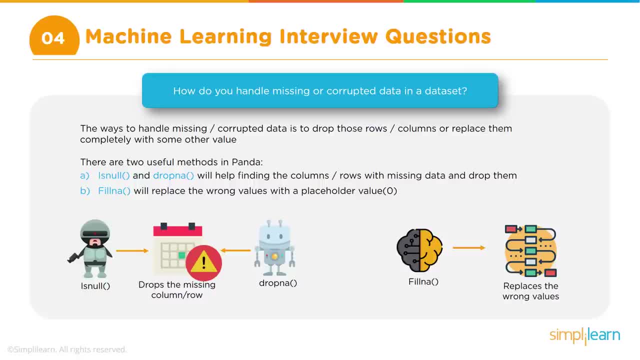 I think it really depends on what exactly the situation is, And there are multiple ways of handling the missing data or corrupt data. Now let's take a few examples. Now let's say you have data where some values in Some of the columns are missing and you have pretty much half of your data having these. 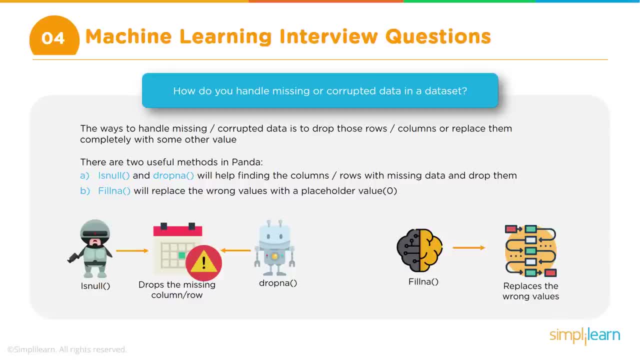 missing values in terms of number of rows. Okay, That could be one situation. Another situation could be that you have records or data missing, but when you do some initial calculation- how many records are corrupt, or how many rows, or observations as we call? 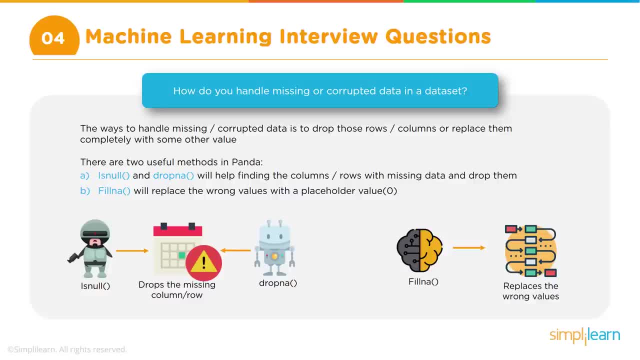 it has this missing data. Let's assume it is very minimal, like 10%. Okay. Now between these two cases, Okay, So let's assume that this is not a mission critical situation And in order to fix this 10% of the data, the effort that is required is much higher. 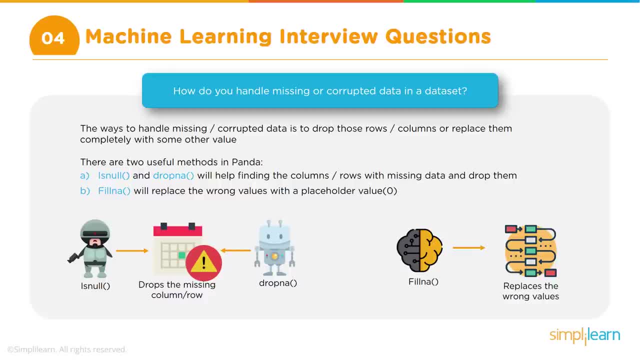 And obviously effort means also time and money, right? So it is not so mission critical and it is okay to, let's say, get rid of these records. So obviously one of the easiest ways of handling the data part or missing data is remove those. 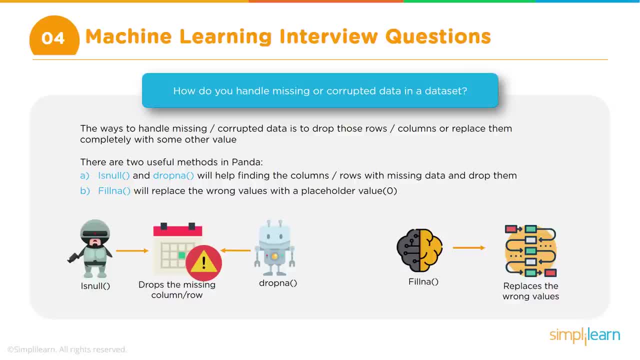 records or remove those observations from your analysis. So that is the easiest way to do. But then the downside is, as I said in, as in the first case, if, let's say, 50% of your data is like that because some column or the other is missing, 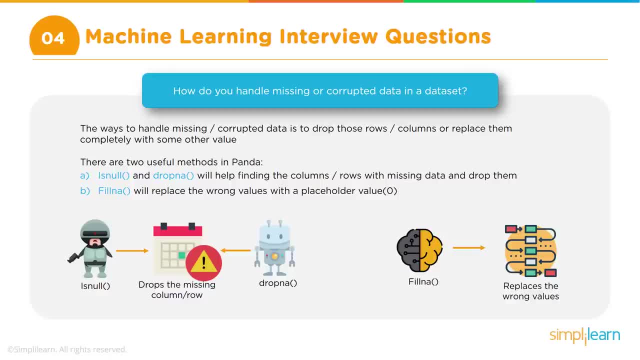 So it is not like every in every place, in every row, the same column is missing. but you have in maybe 10% of the records: column one is missing and another 10%. column two is missing, Another 10%. column three is missing, and so on and so forth. 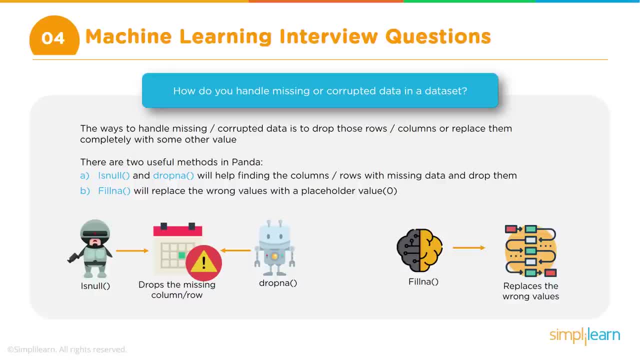 So it adds up to maybe half of your data set. So you cannot completely remove half of your data set. Then the whole purpose is lost. Okay, So then how do you handle it? Then you need to come up with ways of filling up this data with some meaningful value, right? 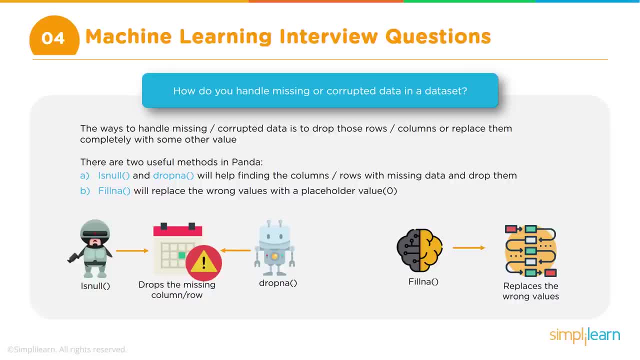 That is one way of handling. So when we say meaningful value, what is that meaningful value? Let's say, for a particular column. you might want to take a mean value for that column and fill wherever the data is missing. fill up with that mean value. 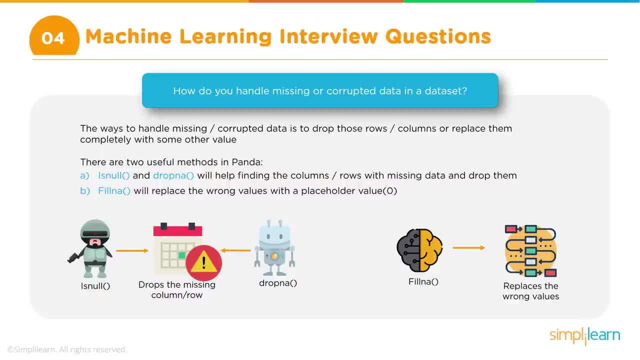 So that when you're doing the calculations, your analysis is not completely way off. So you have values which are not missing, First of all, so your system will work. Number two: these values Are not so completely out of whack that your whole analysis goes for a toss right. 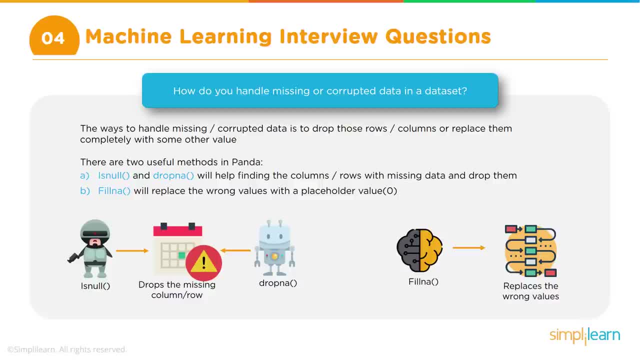 There may be situations where, if the missing values, instead of putting mean, maybe a good idea to fill it up with the minimum value, or with a zero, So, or with the maximum value again. as I said, there are so many possibilities. 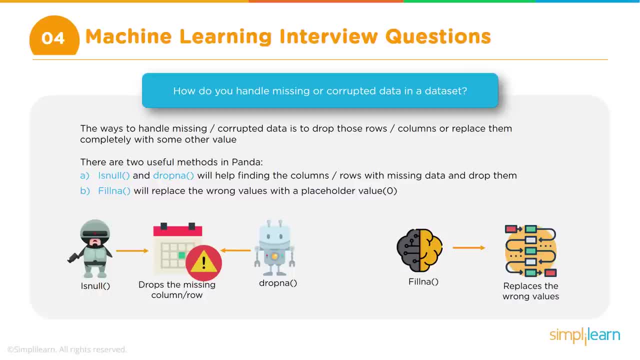 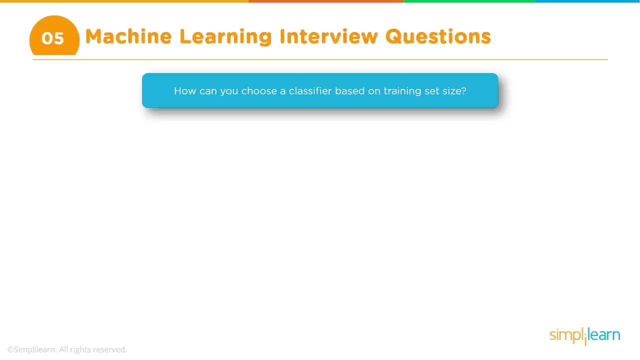 So there is no like one correct answer for this. You need to basically talk around this and illustrate with your experience, As I said, that would be the best. Otherwise, this is how you need to handle this question. Okay, So then the next question can be: how can you choose a classifier based on a training? 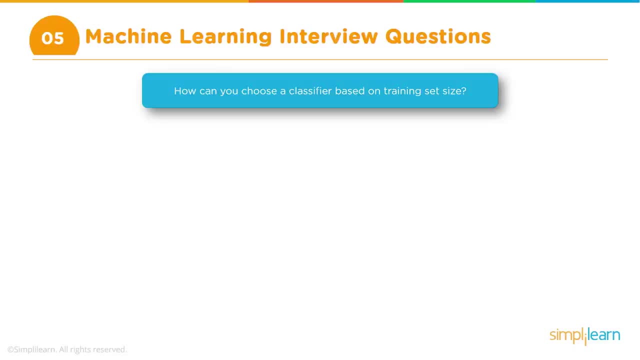 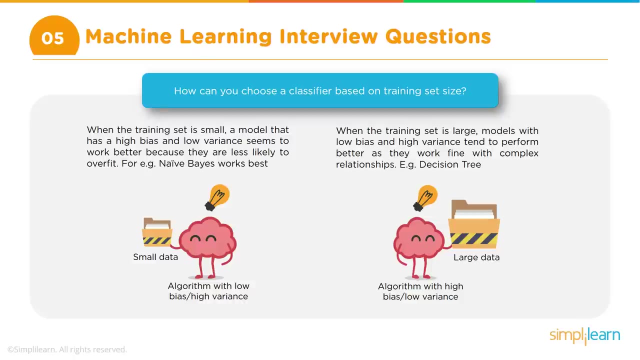 set data size. So, again, this is one of those questions where you probably do not have like a one size fits all answer. First of all, you may not, let's say, decide your classifier based on the training set size. Maybe not the best way to decide the type of the classifier. 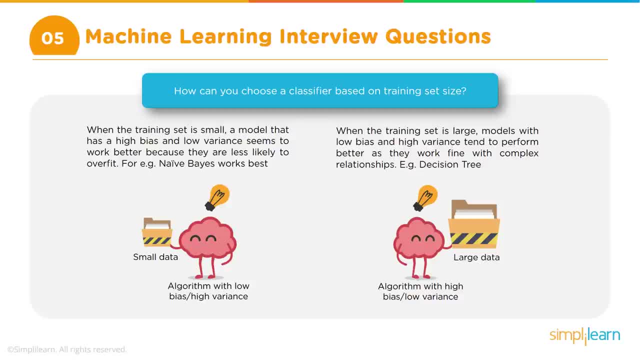 And even if you have to, there are probably Some thumb rules which we can use, but then again every time. So, in my opinion, the best way to respond to this question is: you need to try out few classifiers, irrespective of the size of the data, and you need to then decide on your. 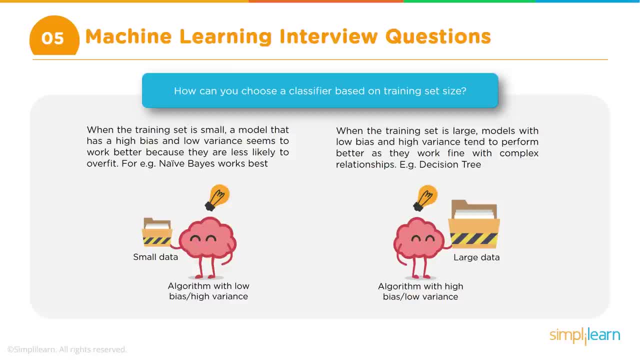 particular situation, which of these classifiers are the right ones? This is a very generic issue, So you will never be able to just by if somebody defines a problem to you and somebody even if it's if they show the data to you or tell you what is the data. 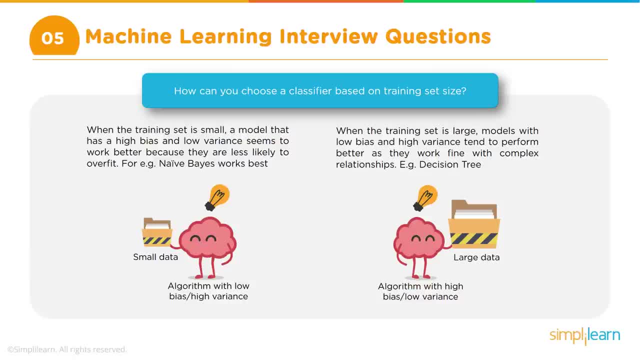 Okay, Or even the size of the data. I don't think there is a way to really say that, yes, this is the classifier that will work here. No, that's not the right way, So you need to still, you know, test it out, get the data, try out a couple of classifiers. 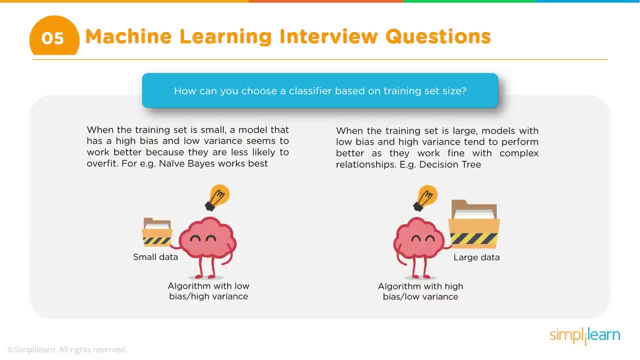 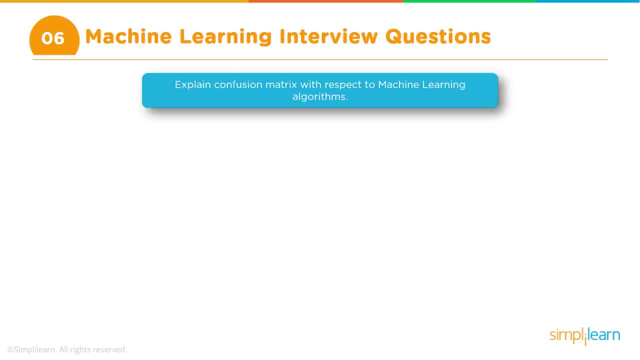 and then only you will be in a position to decide which classifier to use. You try out multiple classifiers, see which one gives the best accuracy, And only then you can decide. Then you can have a question around confusion matrix. So the question can: 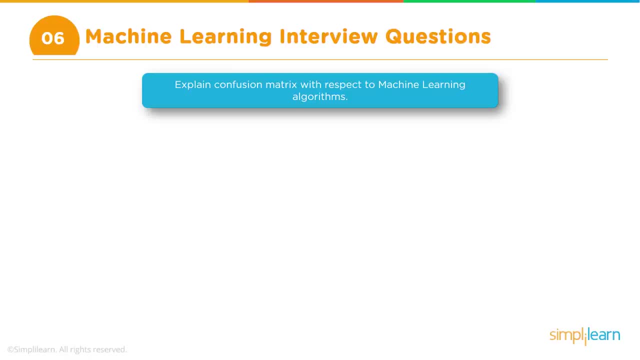 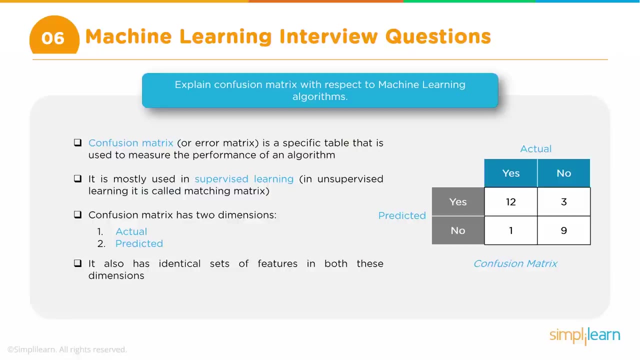 Be explained. confusion matrix, right, So confusion matrix. I think the best way to explain it is by taking an example and drawing like a small diagram. Otherwise it can really become tricky. So my suggestion is to take a piece of pen and paper and explain it by drawing a small. 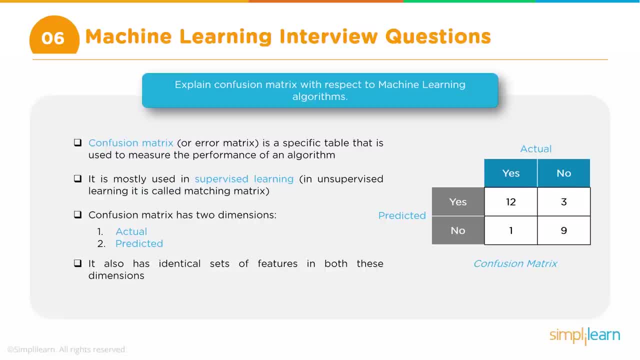 matrix and confusion. matrix is about to find out. this is used especially in classification learning process And when you get the results- and the our Model predicts the results- you compare it with the actual value and try to find out what is the accuracy. 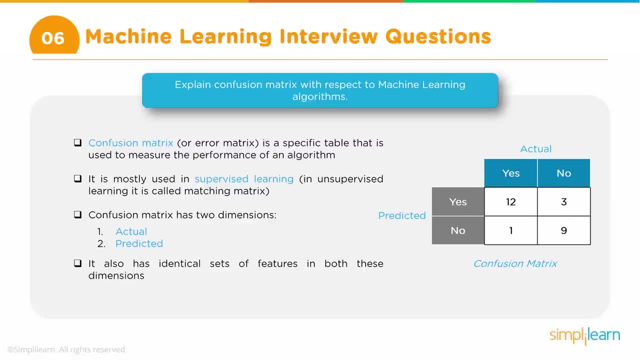 Okay, So in this case, let's say this is an example of a confusion matrix and it is a binary matrix, So you have the actual values, which is the labeled data right, And which is so you have how many yes and how many no. 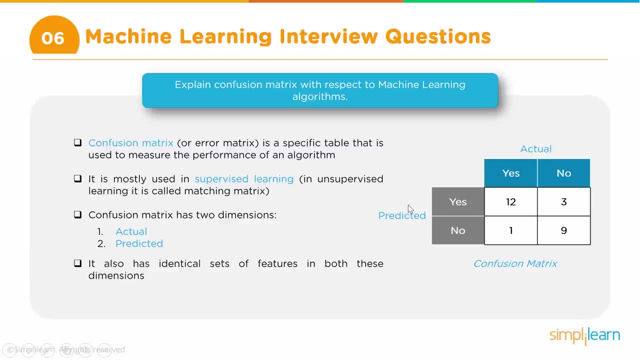 So you have that information and you have the predicted values- How many yes and how many no, right? So The total actual values, the total yes is 12 plus 1,, 13,, and they are shown here. And the actual value no's are 9 plus 3, 12.. 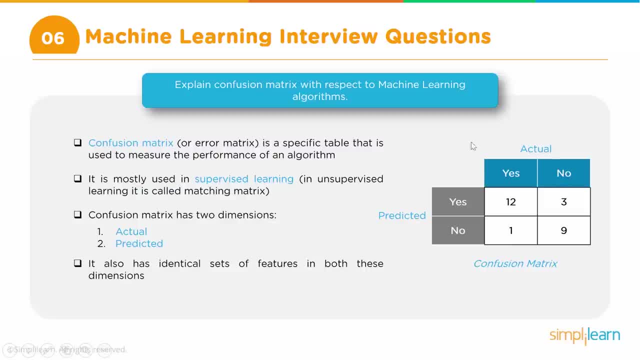 Okay, So that is what this information here is. So this is about the actual and this is about the predicted. Similarly, the predicted values there are: yes are 12 plus 3, 15 yeses and no are 1 plus. 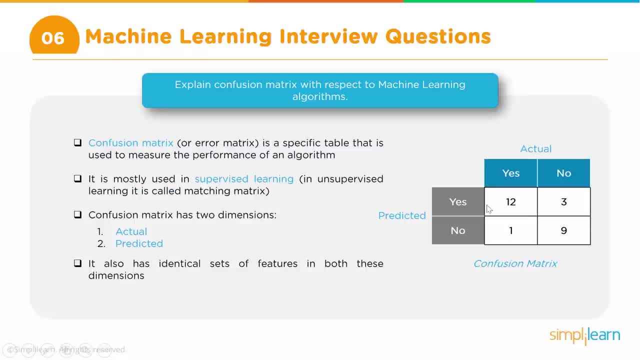 9,, 10 no's. Okay, So this is the way to look at this. confusion: matrix, Okay, And out of this, what is the meaning? Conversion matrix? So there are two or three things that needs to be explained outright. 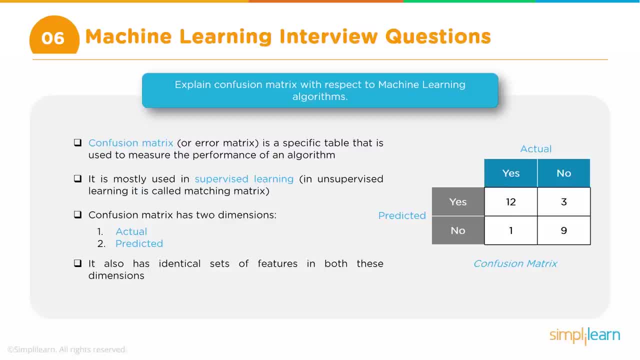 The first thing is for a model to be accurate. the values across the diagonal should be high, like in this case. right, That is one Number two. the total sum of these values is equal to the total observations in the test data set. 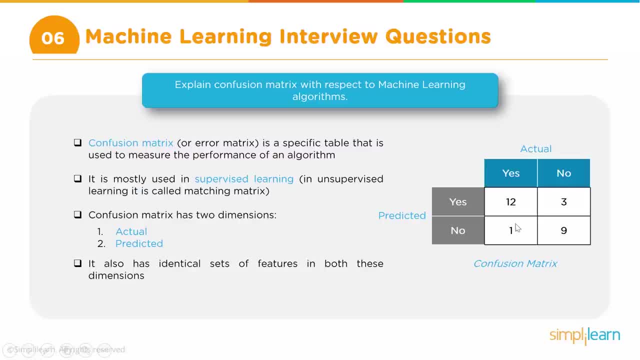 So in this case, for example, you have 12 plus 3, 15 plus 10, 25.. So that means we have 25 observations in our test data set. Okay, So these are the two things you need to find. 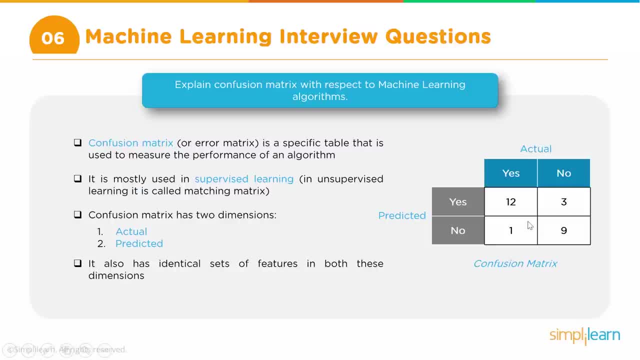 First explain that the total sum in this matrix the numbers is equal to the size of the test data set and the diagonal values indicate the accuracy. So by just by looking at it, you can probably have an idea about: is this an accurate model? 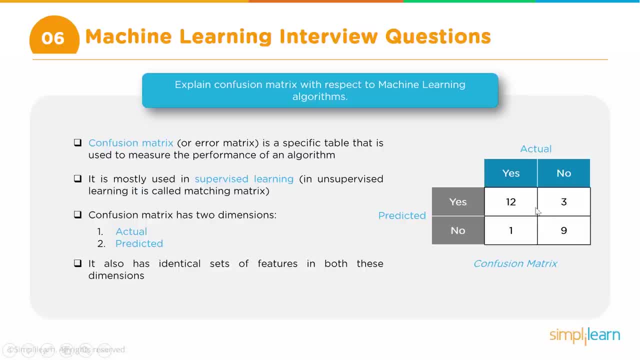 Is the model being accurate If they're all spread out equally in all these four boxes, that means probably the accuracy is not very good. Okay, Now how do you calculate the accuracy itself? Right, How do you calculate accuracy? Okay. 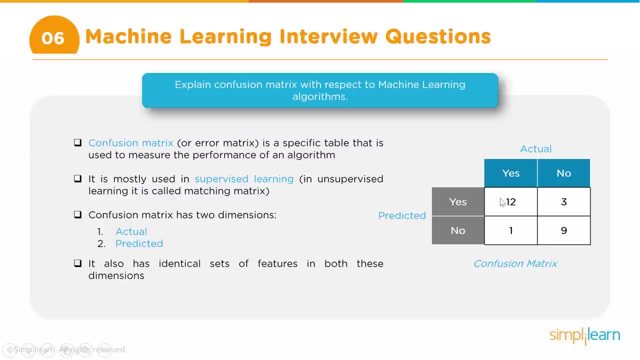 So it is a very simple mathematical calculation. You take some of the diagonals right, So in this case it is nine plus 12, 21 and divide it by the total. So in this case, what will it be? Let's me take a pen. 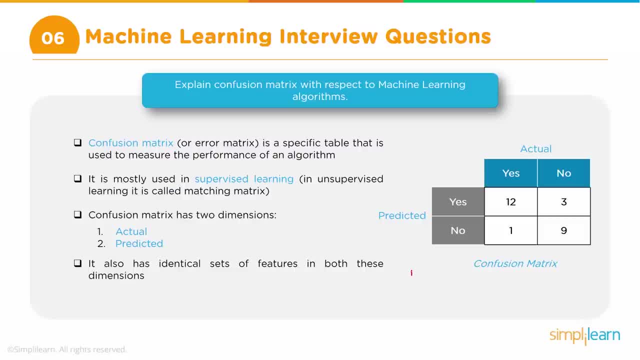 So your, your diagonal values is equal to. if I say D is equal to 12 plus nine, So that is 21,. right, And the total data set is equal to right. We just calculated it is 25.. So what is your accuracy? 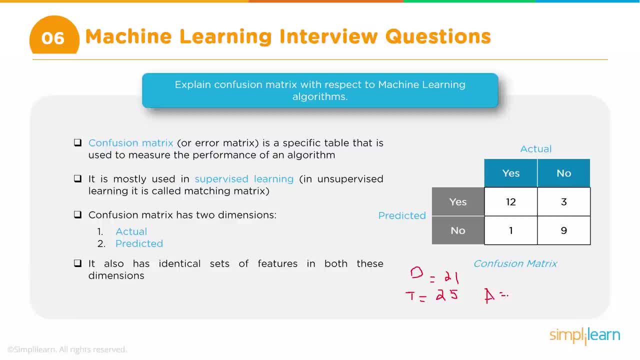 It is 21 by your accuracy is equal to 21 by 25.. And this turns out to be about 85%, right? So this is 85%. So that is our accuracy. Okay, So this is the way you need to explain draw diagram. 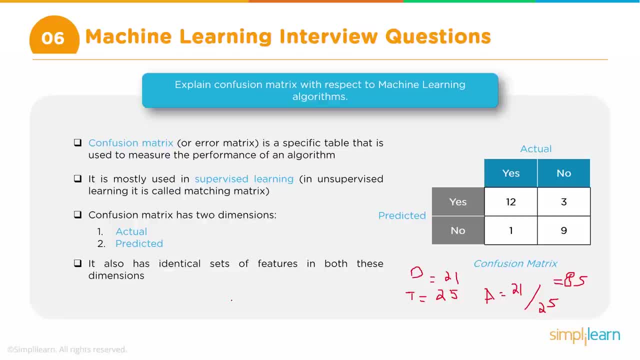 Give an example. Maybe it may be a good idea to be prepared with an example so that it becomes easy for you. You don't have to calculate those numbers on the fly, Right. So a couple of hints are that you take some numbers which are with, which add up. 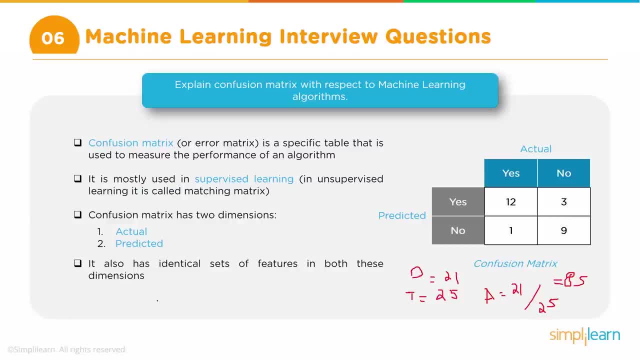 That is always a good idea, So you don't have to really do this complex calculations. So the total value will be a hundred and then diagonal values. you divide. Once you find the diagonal values, that is equal to your percentage. Okay, All right. 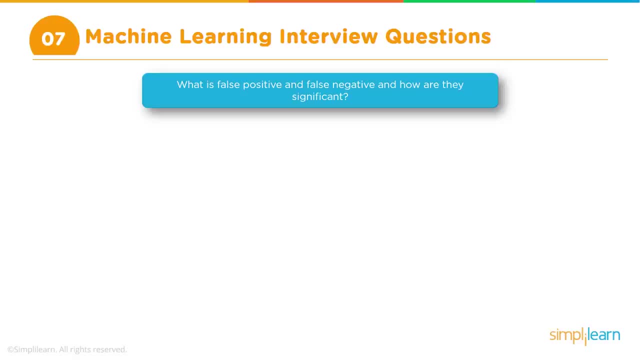 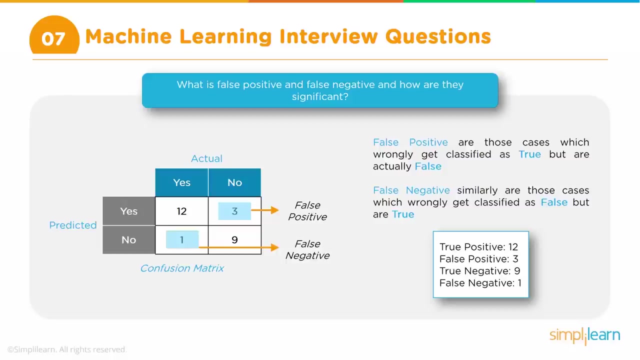 So the next question can be a related question about false positive and false negative. So what is false positive and what is false negative? Now, once again, the best way to explain this is using a piece of paper and pen. Otherwise, it will be pretty difficult to explain this. 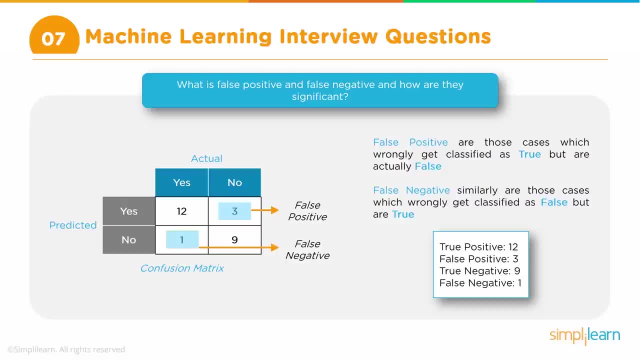 So we use the same example of the confusion matrix and, uh, we can explain that. So a confusion matrix looks somewhat like this And, um, when we just take, yeah, it looks somewhat like this, and we continue with the previous example, where this is the actual value. 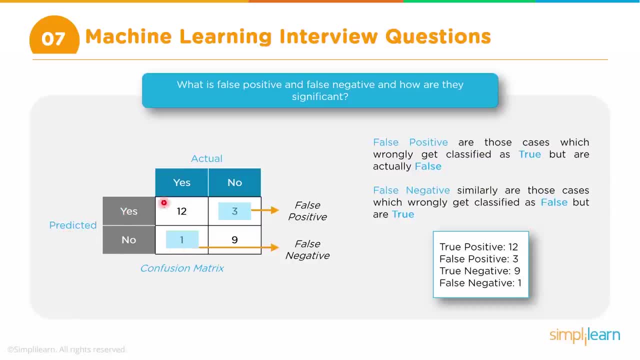 This is the predicted value And uh, in the actual value we have 12 plus 1, 13 yeses and 3 plus 9, 12 nos. and the predicted values There are 12 plus 3, 15 yeses and uh, 1 plus 9, 10 nos. 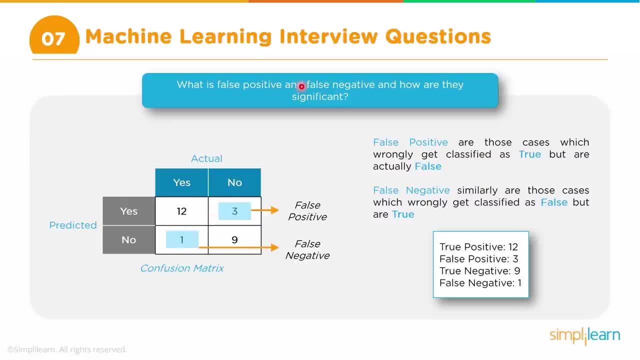 Okay, Now this particular case, which is the false positive. What is a false positive? First of all, the second word which is positive- Okay- Is referring to the predicted value, So that means the system has predicted it as a positive, but the real value? 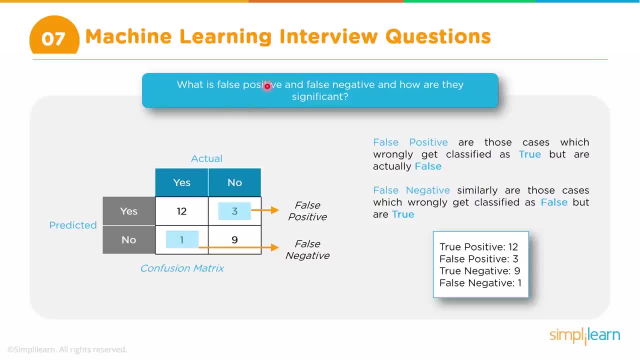 So this is what the false comes from, but the real value is not positive. Okay, That is the way you should understand This term: false positive or even false negative. So false positive, So positive is what your system has predicted. So where is that system predicted? 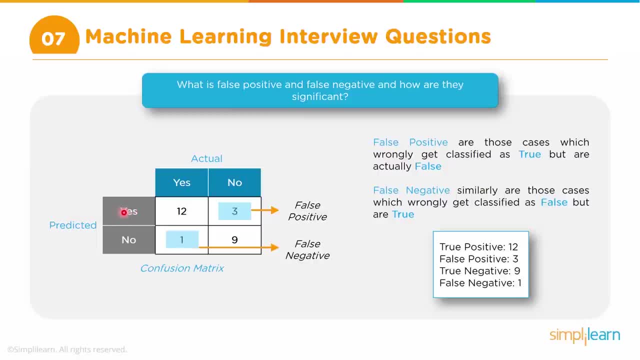 This is the one positive is what? Yes, So you basically consider this row. Okay, Now, if you consider this row, so this is, this is all positive values, This entire row is positive values. Okay, Now, the false positive is the one with where the value- actual value- is negative. 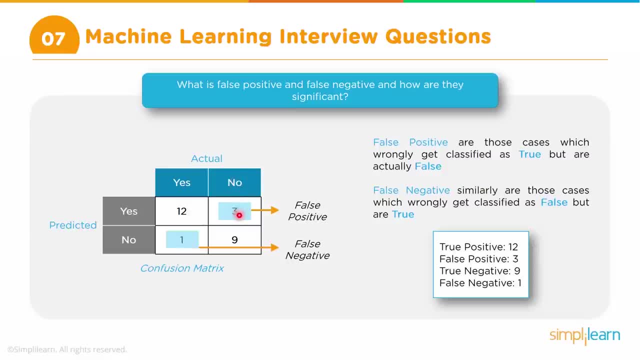 Predicted value is positive, but the actual value is negative. Okay, This is a false positive right, And here is a true positive. So the predicted value is positive and the actual value is also positive. Okay, I hope this is making sense. 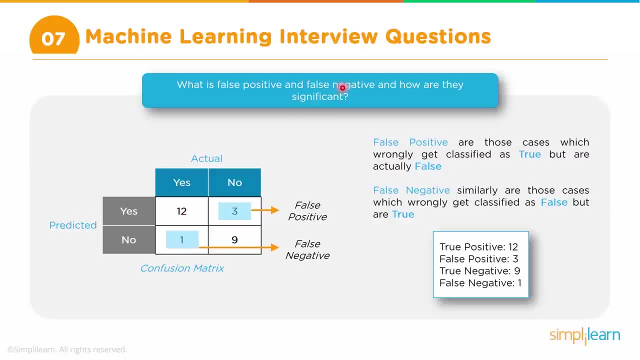 Now let's take a look at what is false negative, false negative, So negative is the second term. That means that is the predicted value that we need to look for. So which are the predicted negative values? This row corresponds to predicted negative values. 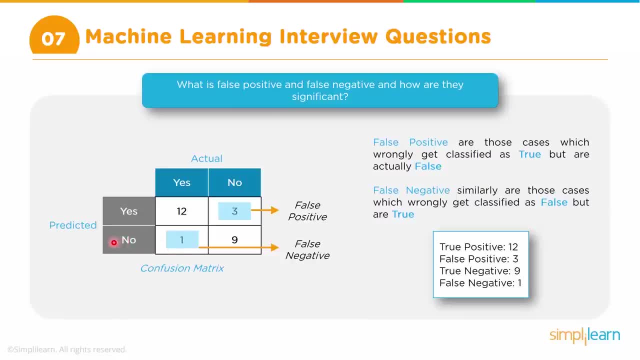 All right, So this row corresponds to predicted negative values And what they are asking for False. So this is the row for predicted negative values And the actual value is this one. right? This is predicted negative and the actual value is also negative. 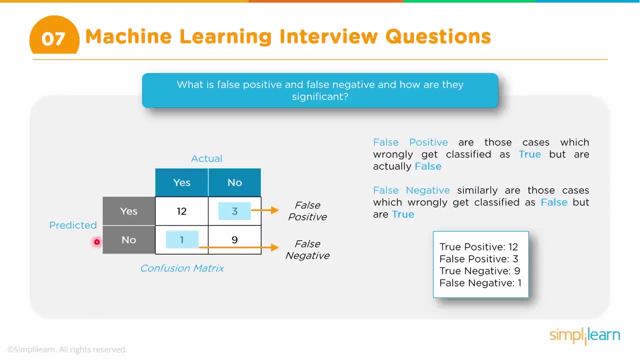 Therefore, this is a true negative. So the false negative is this: one: Predicted is negative, but actual is positive, right? So this is the false negative. So this is the way to explain and this is the way to look at false, positive and false. 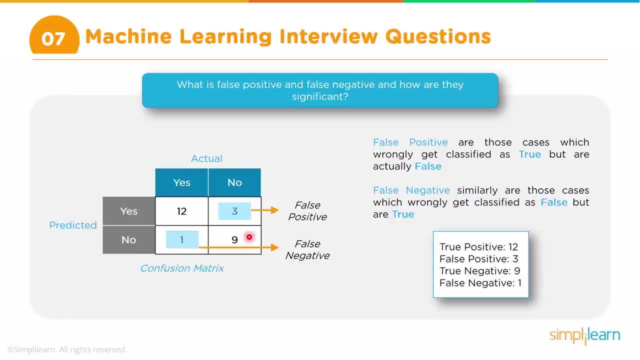 negative. Same way there can be true positive and true negative And true negative as well. So, again, positive, the second term you need to use to identify the predicted row right. So if we say true, positive, positive we need to take for the predicted part. 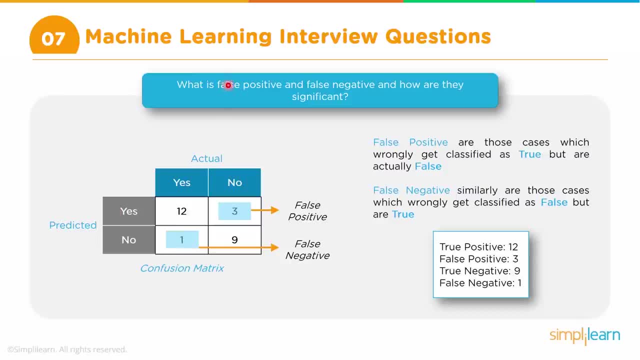 So predicted positive is here Okay. And then the first term is for the actual: So true, positive. So true, in case of actual, is yes, right. So true, positive, is this one, Okay. And then, in case of actual, the negative. 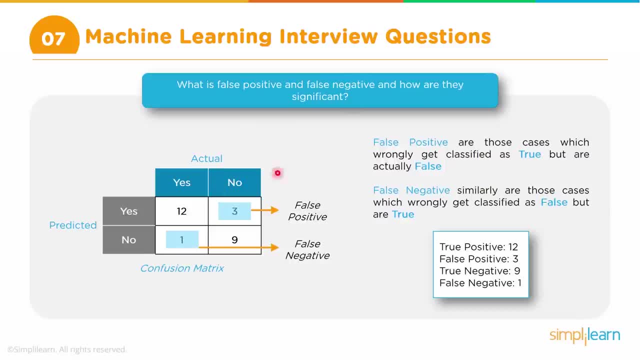 Now we are talking about- let's say True, negative, True, negative, Negative is this one, and the true comes from here. So this is true, negative, right Nine is true negative. The actual value is also negative and the predicted value is also negative. 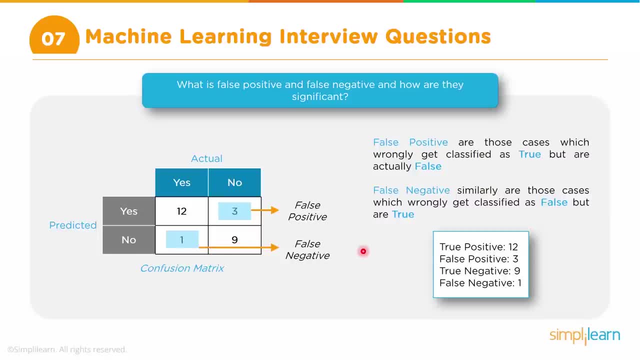 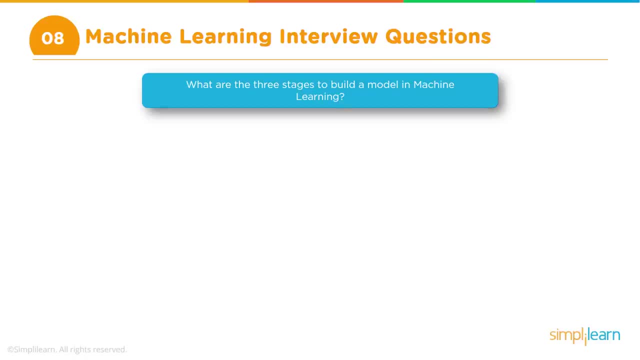 Okay, So that is the way you need to explain this: the terms false positive, false negative and true positive, true negative. Then you might have a question like: what are the steps involved in the machine learning process, Or what are the three steps in the process? 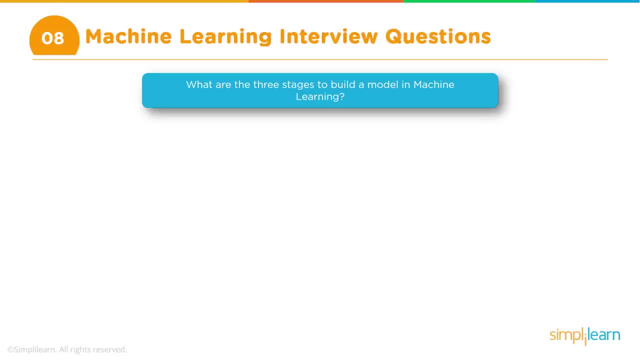 What are the steps involved in the process of developing a machine learning model? right, So it is around the methodology that is applied. So basically, the way you can probably answer in your own words, but the way the model development of the machine learning model happens is like this. 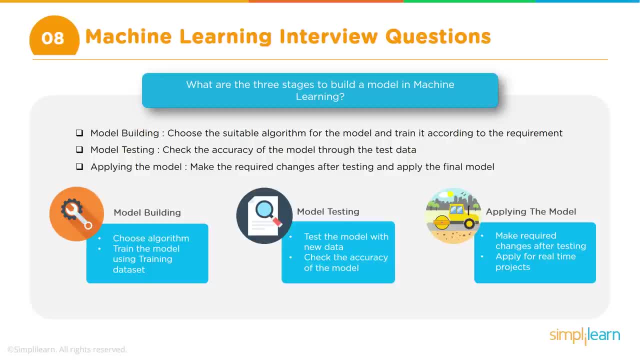 So first of all, you try to understand the problem and try to figure out whether it is a classification problem or a regression problem. Based on that, you select a few algorithms and then you start the process of training these models. So you can either do that or you can. after due diligence, you can probably decide that. 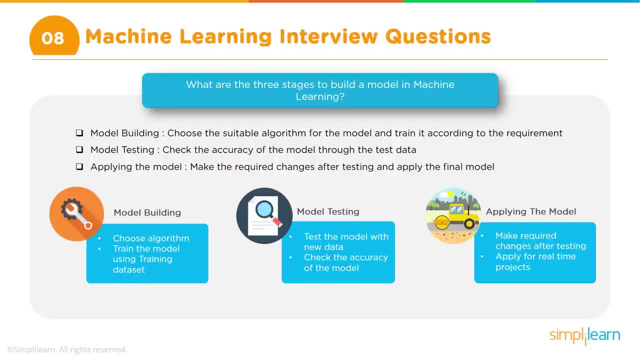 there is one particular algorithm, that which is most suitable. Usually it happens through trial and error process, but at some point you will decide that, okay, this is the model we are going to use. Okay, So in that case we have the model algorithm and the model decided, and then you need to. 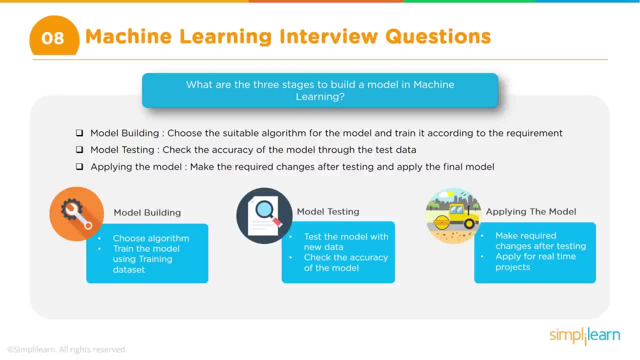 do the process of training the model and testing the model, And this is where, if it is supervised learning, you split your data Label data into training data set and test data set and you use the training data set to train your model And then you use the test data set to check the accuracy, whether it is working fine or 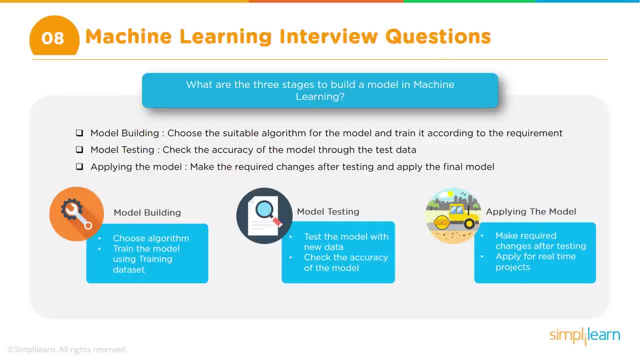 not. So you test the model before you actually put it into production, right. So once you test the model, you're satisfied it's working fine. Then you go to the next level, which is putting it for production. And then in production, obviously new data will come and the inference happens. 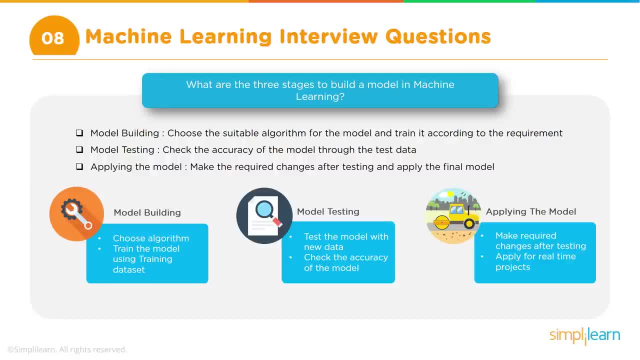 So the model is readily available And And only thing that happens is new data comes and the model predicts the values, whether it is regression or classification. Now, so this can be an iterative process, So it is not a straightforward process where you do the training for the testing and then 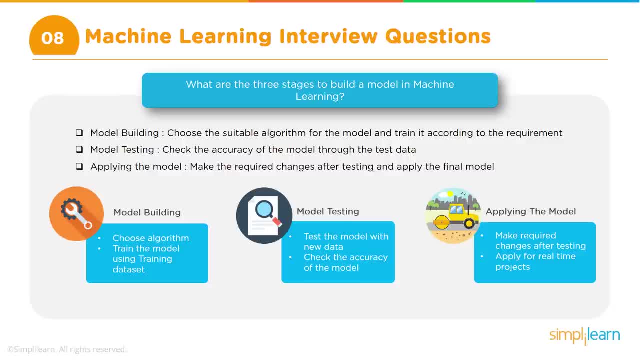 you move it to production. No, So during the training and test process, there may be a situation where, because of either overfitting or things like that, the test doesn't go through, which means that you need to put that back into the training process. 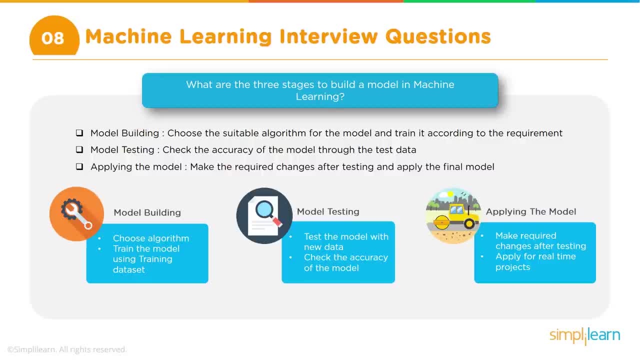 So that can be a an iterative process. Not only that: Even if the training and test goes through properly and you deploy the model in production, there can be a situation that the data that actually comes, the real data that comes with that, this model is failing. 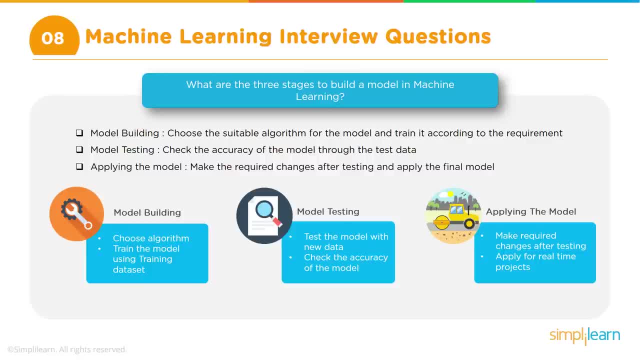 So, in which case you may have to once again go back to the drawing board, or initially it will be working fine, but over a period of time, maybe due to the change in the nature of the data- once again the accuracy will deteriorate. 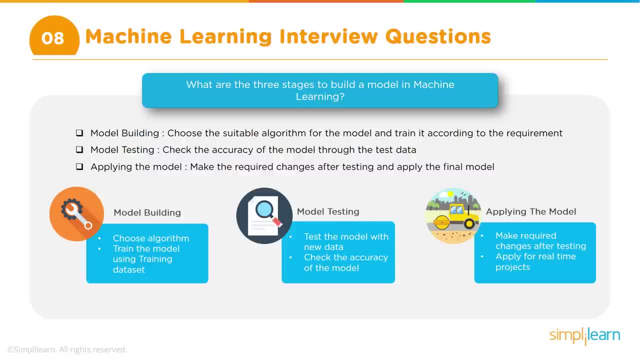 So that is again a recursive process. So once in a while you need to keep checking whether the model is working fine Or not And, if required, you need to tweak it and modify it, and so on and so forth. So let let. this is a continuous process of um tweaking the model and testing it. 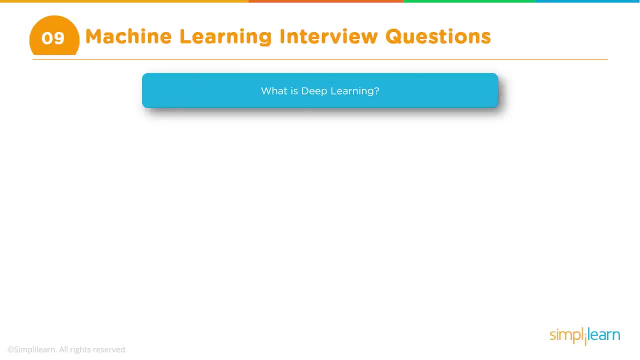 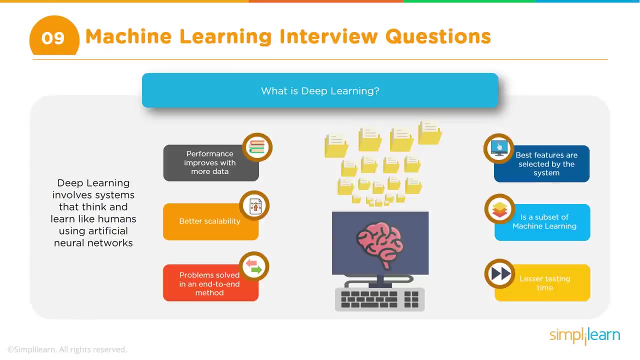 and making sure it is up to date. Then you might have question around deep learning. So, because deep learning is now associated with AI, artificial intelligence and so on, So can be as simple as what is deep learning? So I think the best way to respond to this could be: deep learning is a part of machine. 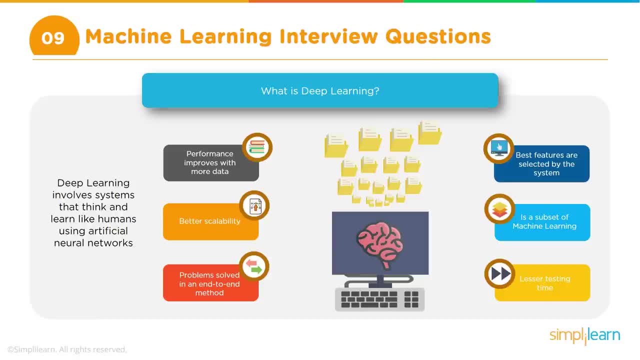 learning, And Then obviously, the question would be: then what is the difference? right? So deep learning, you need to mention there are two key parts that interviewer will be looking for when you are defining deep learning. So first is, of course, deep learning is a subset of machine learning. 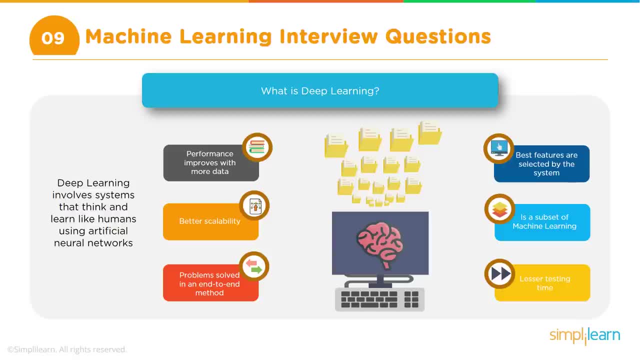 So machine learning is still the bigger let's say, uh, scope, and deep learning is one part of it. So then, what exactly is the difference? Deep learning is primarily when we are implementing these, uh, our algorithms, or when we are using 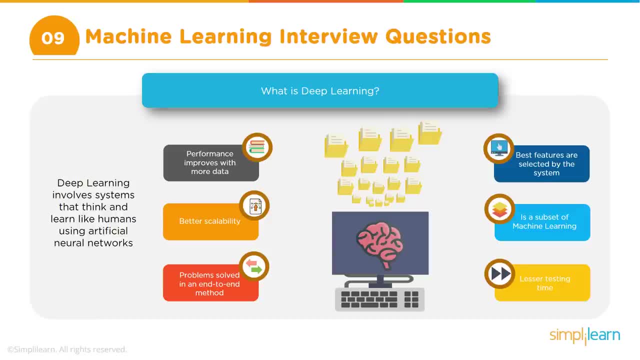 neural networks For doing our training and classification and regression and all that right. So when we use neural network then it is considered as deep learning And the term deep comes from the fact that you can have several layers of neural networks and these are called deep neural networks. 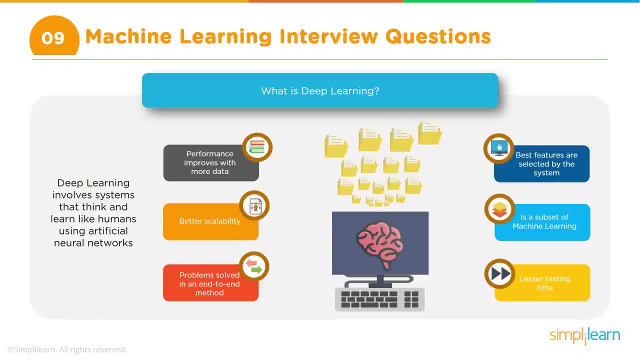 And therefore the term deep, deep learning. uh, the other difference between machine learning and deep learning, which they do, or maybe wanting to hear, is that in case of machine learning, the feature Engineering is done manually. What do we mean by feature engineering? 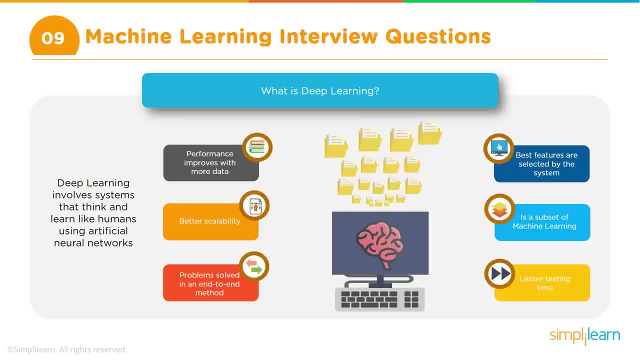 Basically, when we are trying to train our model, we have our training data, right. So we have our training label data and, uh, this data has several. let's say, if it is a regular table, it has several columns. Now, each of these columns actually has information about a feature, right? 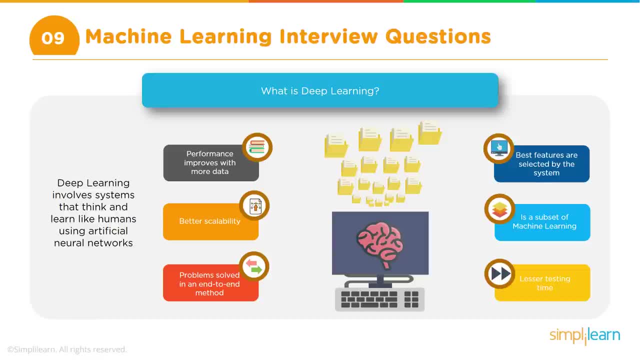 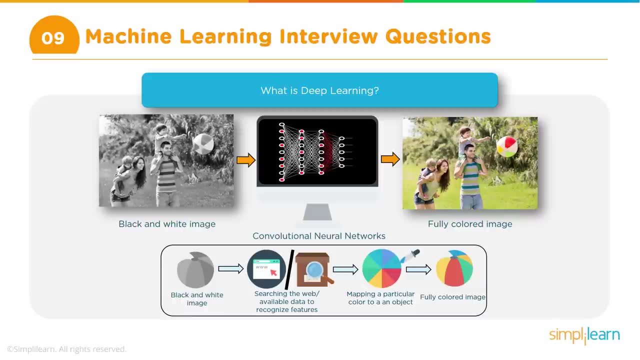 So if we are trying to predict, uh, height, weight and so on and so forth, So these are all features of human beings- Let's see, We have census data and we have all this. So those are the features Now there may be probably 50 or a hundred. in some cases there may be a hundred such 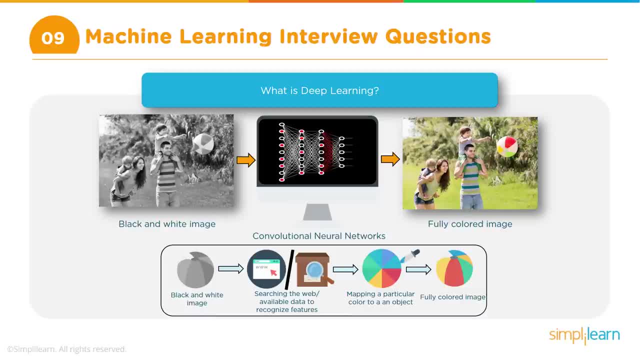 features. Now, all of them do not contribute to our model, right. So we, as a data scientist, we have to decide whether we should take all of them, all the features, or we should throw away some of them. Because, again, if we take all of them, number one of course, your accuracy will probably. 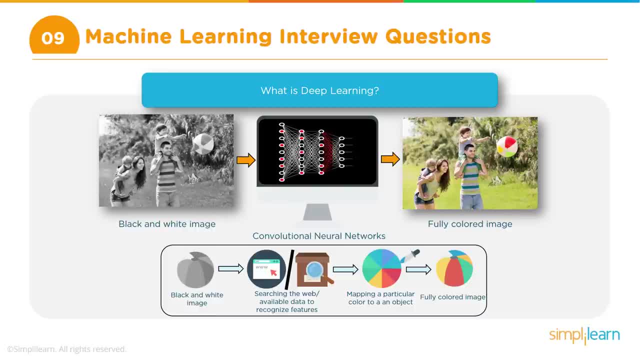 get affected. but also there is a computational part. So if you have so Features and then we have so much data, it becomes very tricky. So in case of machine learning, we manually take care of identifying the features that do not contribute to the learning process, and thereby we eliminate those features and 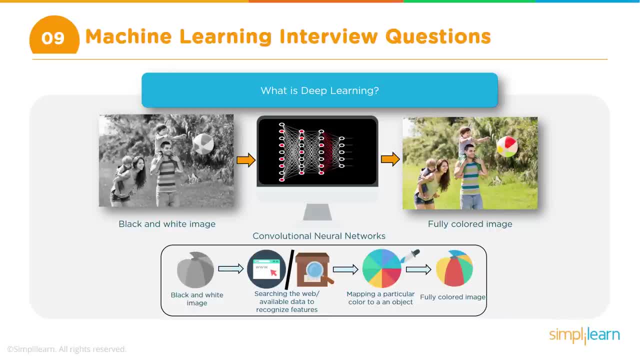 so on. right, So this is known as feature engineering, and in machine learning we do that manually, Whereas in deep learning, where we use neural networks, the model will automatically determine which features to use and which to not use, And therefore feature engineering is. 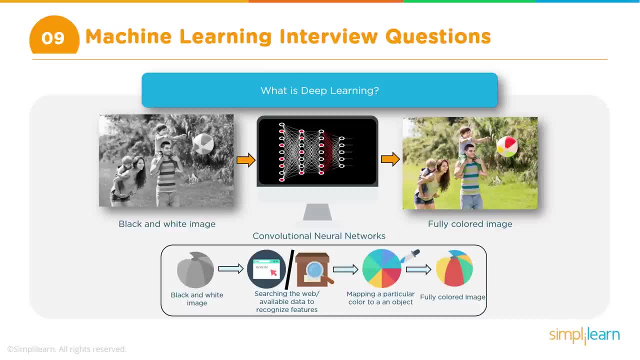 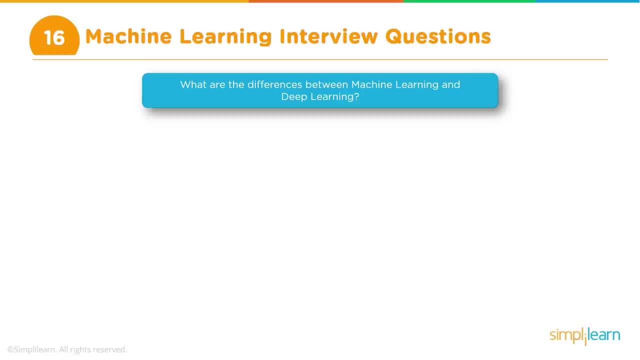 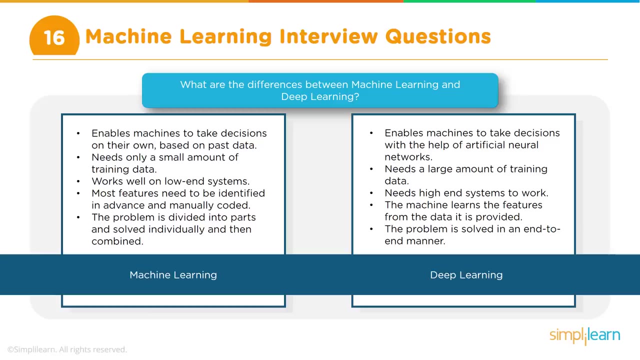 Is also done automatically. So this is a explanation. These are two key things probably will add value to your response. All right, So the next question is: what is the difference between, or what are the differences between, machine learning and deep learning? So here this is a quick comparison table between machine learning and deep learning. 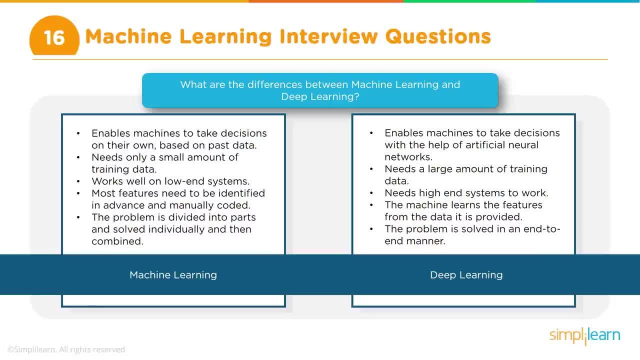 and in machine learning. learning enables machines to take decisions on their own based on past data. So here we are talking primarily of supervised learning, and It needs only a small amount of data for training and then works well on low end systems. So you don't need large machines and most features need to be identified in advance. 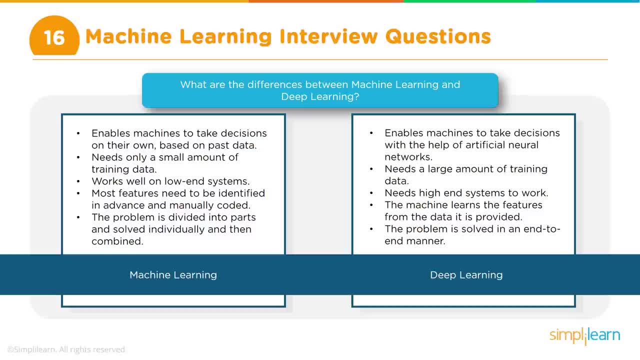 and manually coded. So basically the feature engineering part is done manually and the problem is divided into parts and solved individually and then combined. So that is about the machine learning part in deep learning. Deep learning basically enables machines to take decisions with the help of artificial 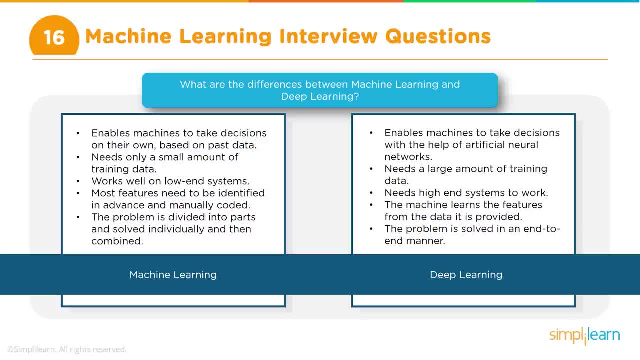 neural networks. So here in deep learning We use neural networks. So that is the key differentiator between machine learning and deep learning. And usually deep learning involves a large amount of data And therefore the training also requires- usually the training process requires- high 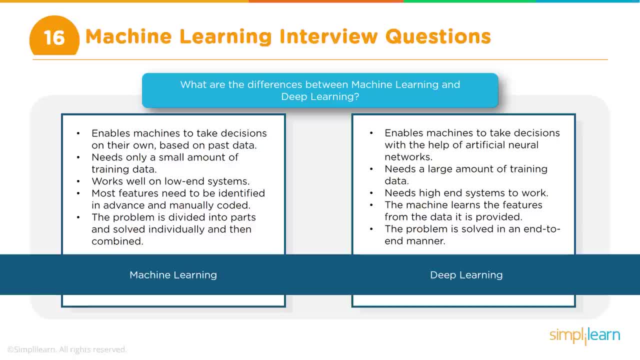 end machines because it needs a lot of computing power And the machine learning features are the or the feature engineering is done automatically, So the neural networks takes care of doing the feature engineering as well, And in case of deep learning, therefore, it is said that the problem is handled end to end. 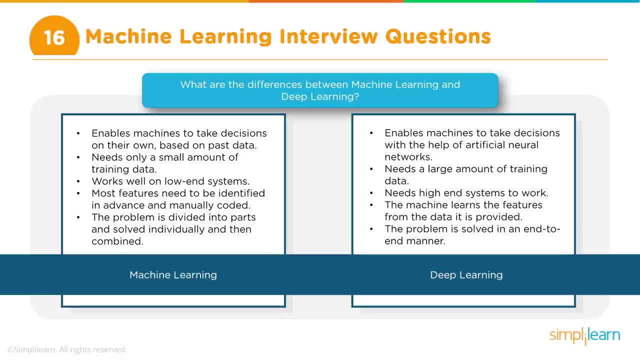 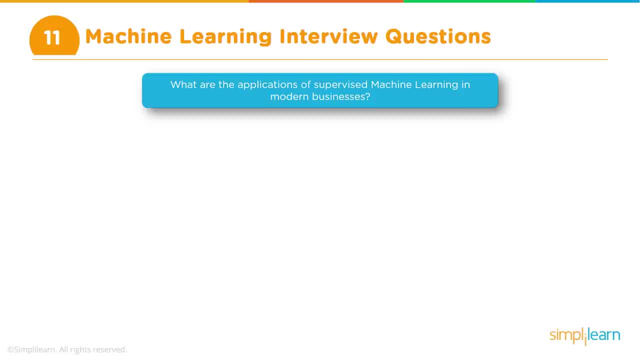 So this is a quick comparison between machine learning and deep learning. in case you have that kind of a question, Then you might get a question around the uses of machine learning or some real life applications of machine learning in modern business. The question may be worded in different ways, but the meaning is: how exactly is machine 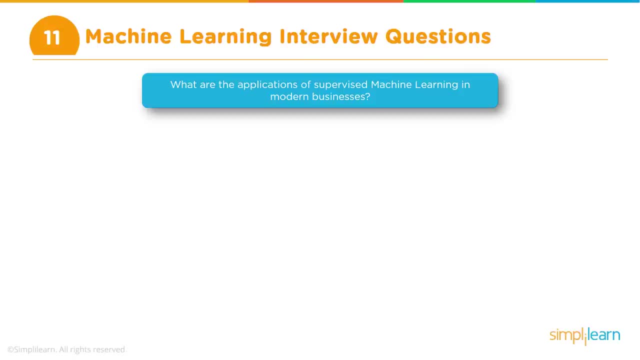 learning used or actually supervised machine learning. It could be a very specific question around supervised machine learning. So this is like give example Skills of supervised machine learning, use of supervised machine learning in modern business. So that could be the next question. So there are quite a few examples or quite a few use cases, if you will, for supervised 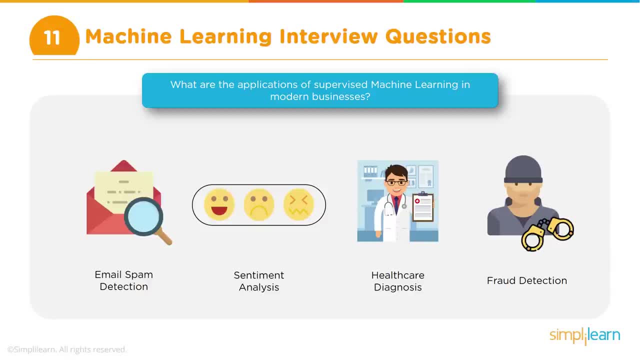 machine learning. The very common one is email spam detection, So you want to train your application or your system to detect between spam and non-spam. So this is a very common business application of supervised machine learning. So how does this work? The way it works is that you obviously have historical data of all of your emails and 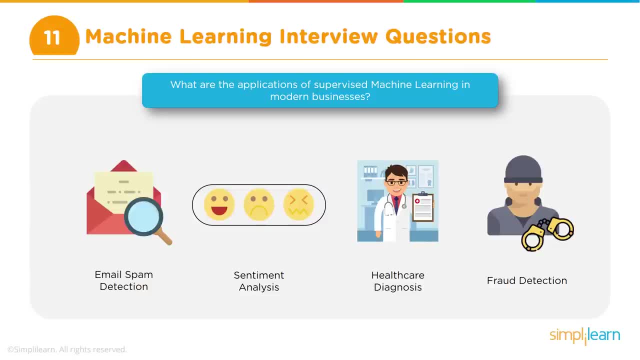 they are categorized as spam and not spam. So that is what is the labeled information, And then you feed this information or all these emails as an input to your model right And the model will then get trained to detect which of the emails are, to detect which is. 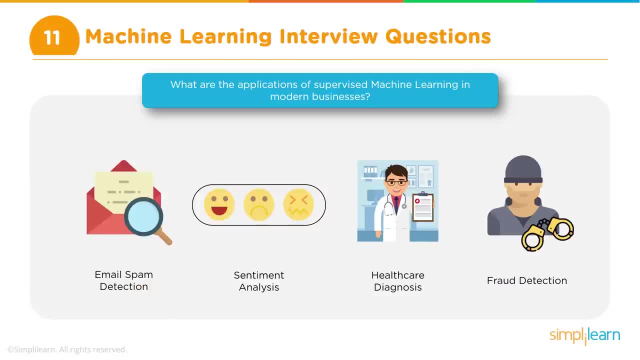 spam and which is not spam. So that is the training process. This is supervised machine learning, because you have labeled data. You already have emails which are tagged as spam or not spam, And then you use that to train your model right. So this is one example. 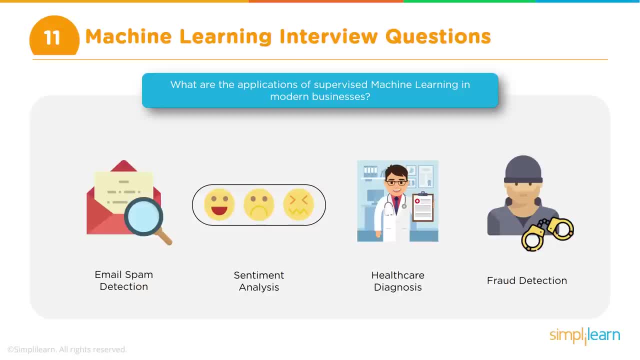 Now there are a few industry specific applications for supervised machine learning. One of the very common ones is in healthcare diagnostics. In healthcare diagnostics you have these images and you want to train models to detect whether from a particular image, whether it can find out if the person is sick or not. 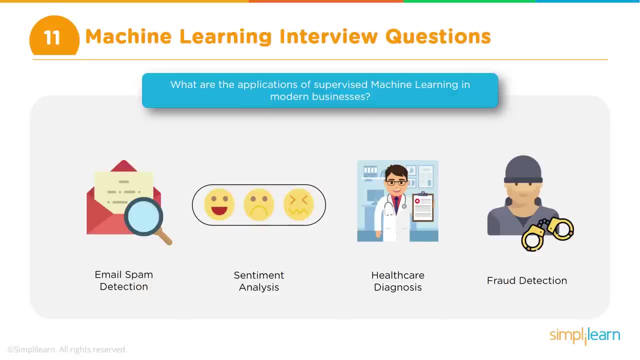 whether a person has cancer or not, right? So this is a very good example of supervised machine learning. Here. the way it works is that existing images- it could be X-ray images, it could be MRI or any of these images- are available and they are tagged saying that, okay, this X-ray image. 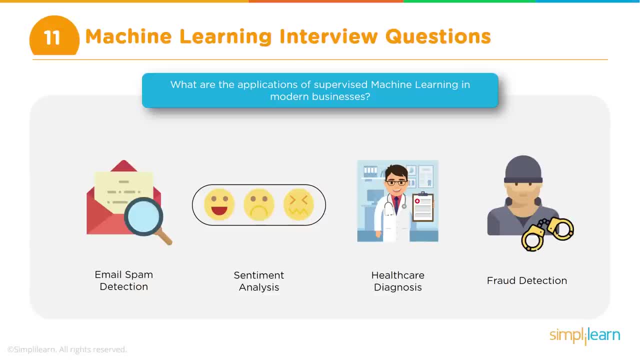 is defective, or the person has an illness, or it could be cancer, whichever illness, right, This person has defective or clear or good image and defective image, something like that. So we come up with a binary- or it could be multiclass as well- saying that this is defective. 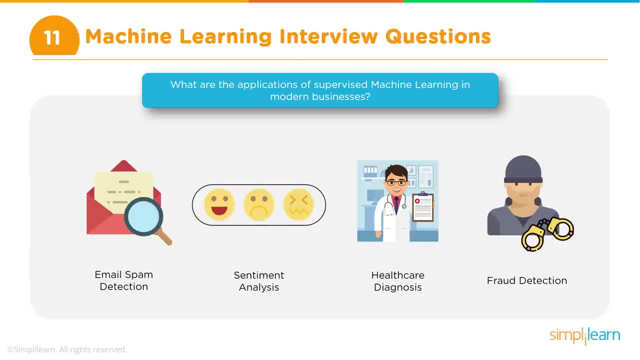 to 10%, this is 25% and so on. But let's keep it simple. You can give an example of just a binary classification. that would be good enough. So you can say that in healthcare diagnostics using image, we need to detect whether a person 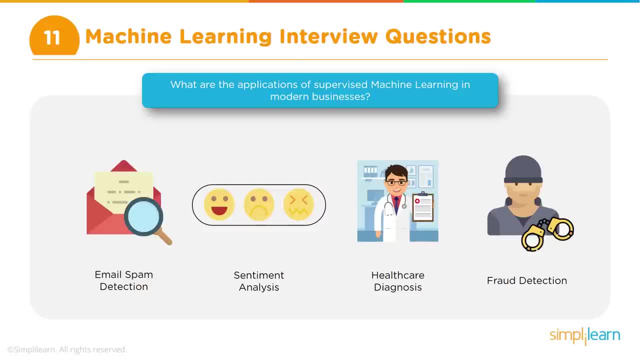 is ill or whether a person is having cancer or not. So here the way it works is you feed labeled images and you allow the model to learn from that so that when new image is fed it will be able to predict whether this person is having that illness or not having. 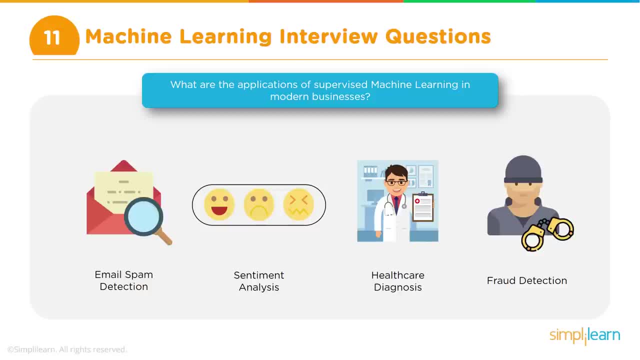 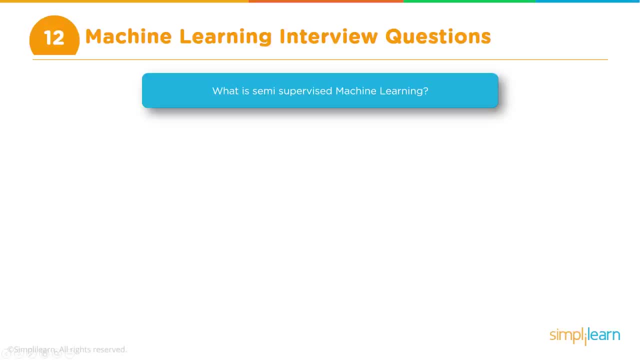 cancer or not, right? So I think this would be a very good example for supervised machine learning in modern business. All right, Then we can have a question like: so we've been talking about supervised and unsupervised, and so there can be a question around semi-supervised machine learning. 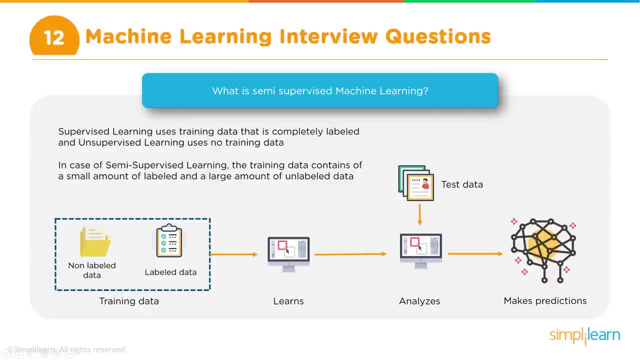 So What is semi-supervised machine learning Now? semi-supervised learning, as the name suggests, it falls between supervised learning and unsupervised learning, But for all practical purposes it is considered as a part of supervised learning, And the reason this has come into existence is that in supervised learning you need labeled. 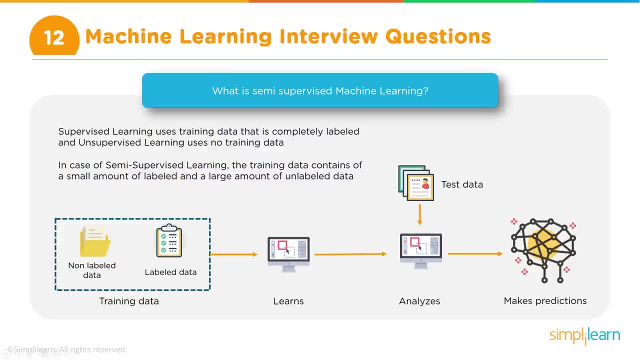 data. So all your data for training, your model has to be labeled. Now this is a big problem In many industries or under many situations. getting the labeled data is not that easy because there's a lot of effort in labeling this data. 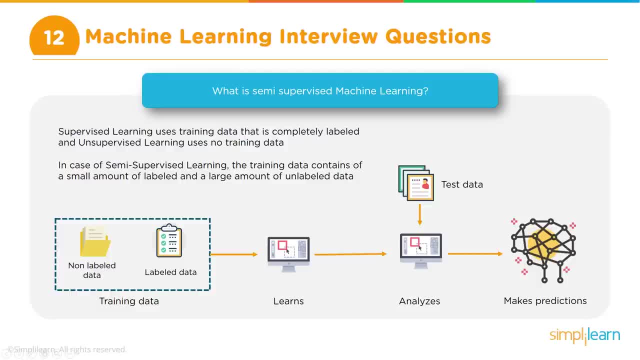 Let's take an example of diagnostic images. We can just, let's say, take X-ray images. Now, there are actually millions of X-ray images available all over the world, but the problem is they are not labeled. So the images are there, but whether it is effective or whether it is good, that information 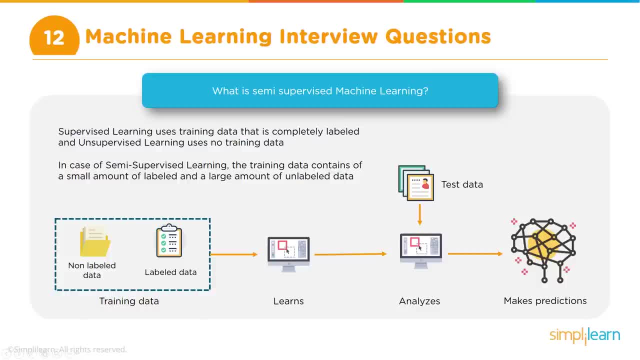 is not available along with it Right In a form that it can be used by a machine, which means that somebody has to take a look at these images- and usually it should be like a doctor- and then say that, okay, yes, 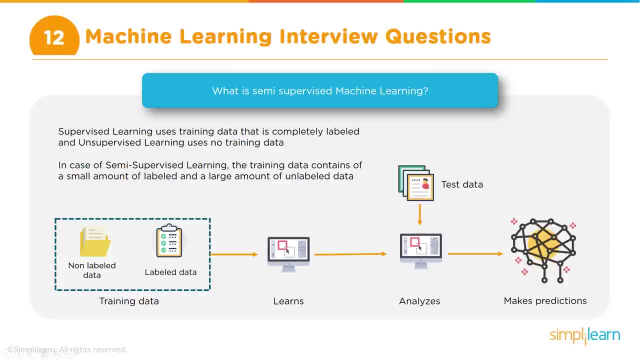 this image is clean, and this image is cancerous, and so on and so forth. Now, that is a huge effort by itself. So this is where semi-supervised learning comes into play. So what happens is there is a large amount of data. maybe a part of it is labeled. then 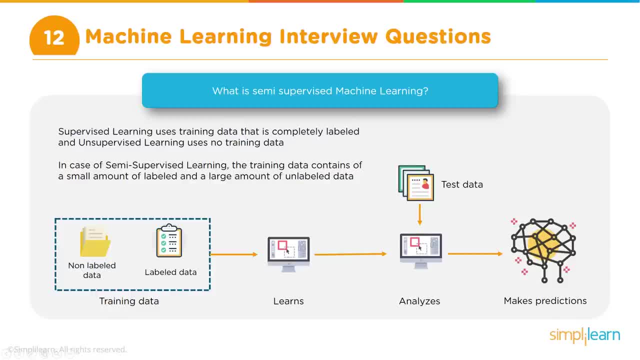 we try some techniques To label the remaining part of the data so that we get completely labeled data and then we train our model. So I know this is a little long winding explanation, but unfortunately there is no quick and easy definition for semi-supervised machine learning. 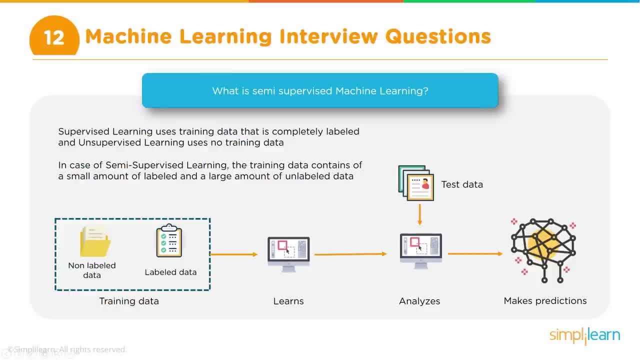 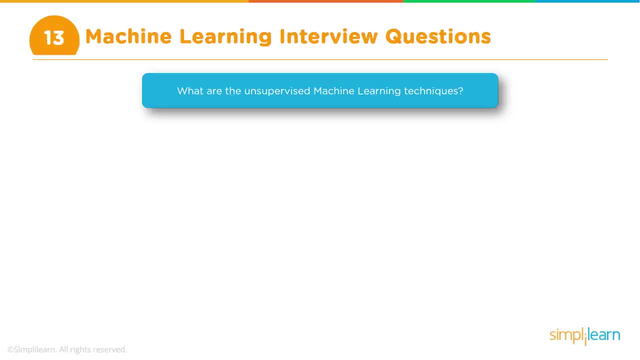 This is the only way, probably, to explain this concept. We may have another question, as what are unsupervised machine learning techniques or what are some of the techniques used? So how do we answer this question? So, unsupervised learning, you can say that there are two types: clustering and association. 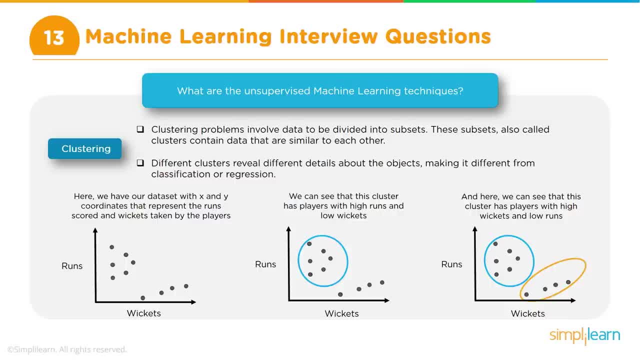 And clustering is a technique where similar objects are put together. There are different ways of finding similar objects, So their characteristics can be measured and if they have most of the characteristics, if they are similar, then they can be put together. This is clustering. 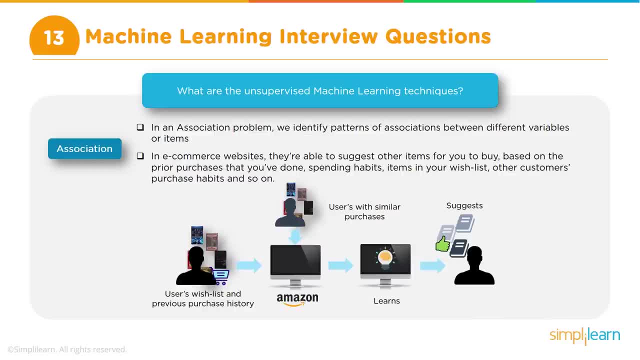 Then association you can. I think the best way to explain association is with an example. In case of association, you try to find out how the items are linked to each other. So, for example, if somebody bought maybe a laptop, the person has also purchased a mouse. 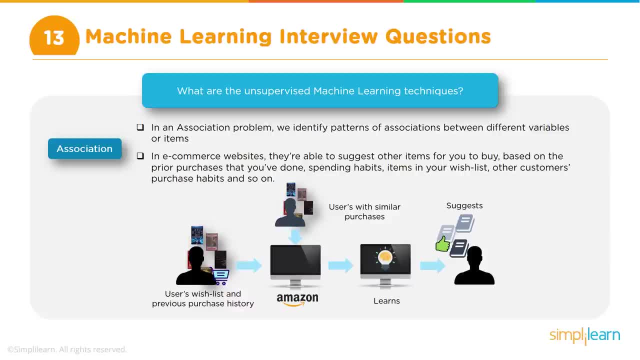 So this is more in an e-commerce scenario, for example, So you can give this as an example. So people who are buying laptops are also buying a mouse, So that means there is an association between laptops and mouse. Or maybe people who are buying bread are also buying butter. 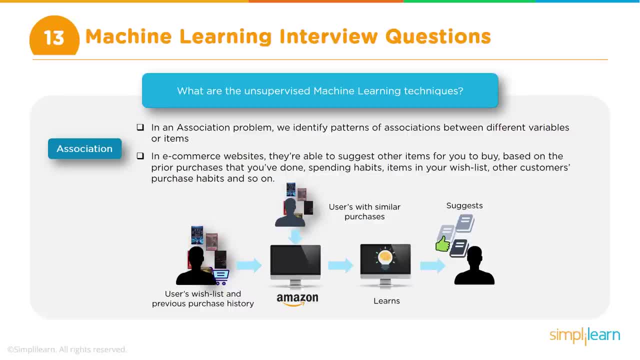 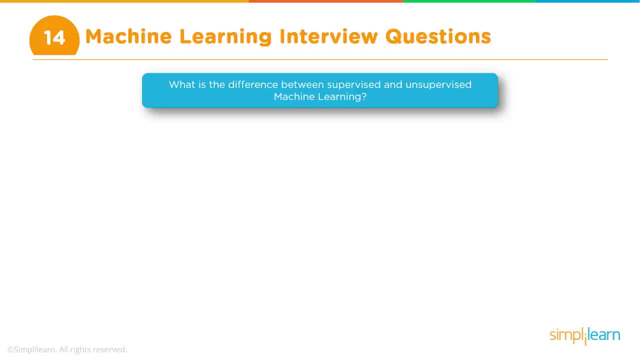 So that is an association that can be created. So this is unsupervised learning, one of the techniques. Okay, All right, then we have a fundamental question: What is the difference between supervised and unsupervised machine learning? So machine learning, these are the two main types of machine learning: supervised and unsupervised. 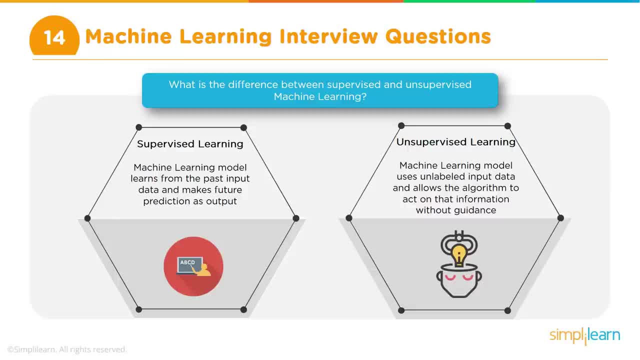 And in case of supervised- and again here, probably the keyword that the person may be wanting to hear is labeled data. Now, very often people say we have historical data and if we run it, it is supervised, And if we don't have historical data, yes, but you may have historical data. 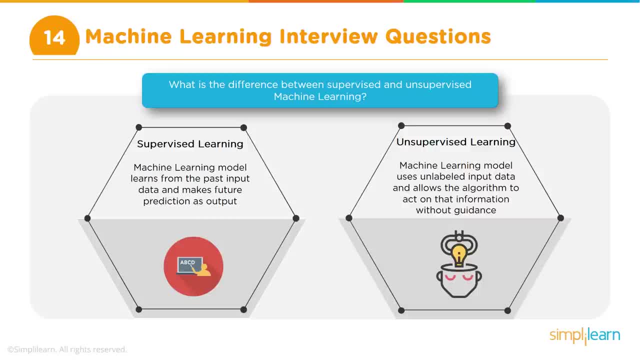 but if it is not labeled then you cannot use it for supervised learning. So it is it's very key to understand that we put in that keyword labeled Okay. So when we have labeled data for training, our model, then we can use supervised learning. 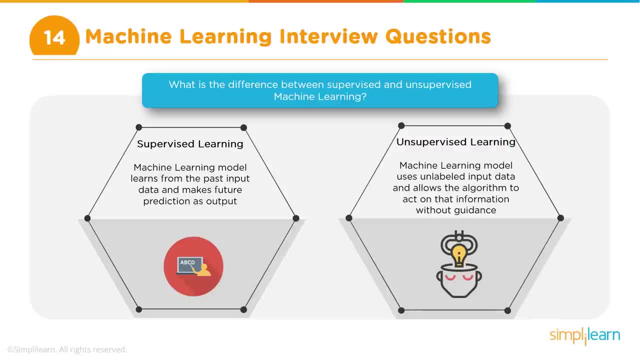 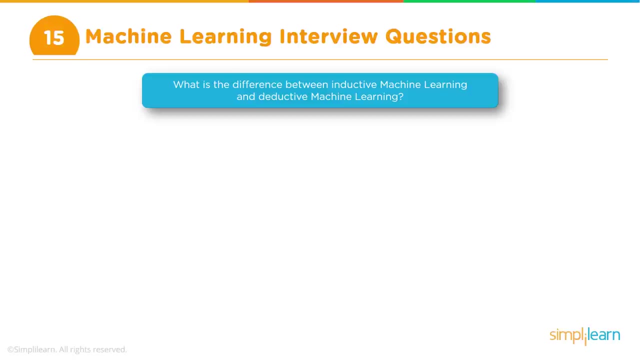 And if we do not have labeled data, then we use unsupervised learning And there are different algorithms available to perform both of these types of trainings. So there can be another question a little bit more theoretical and conceptual in nature. This is about inductive machine learning and deductive machine learning. 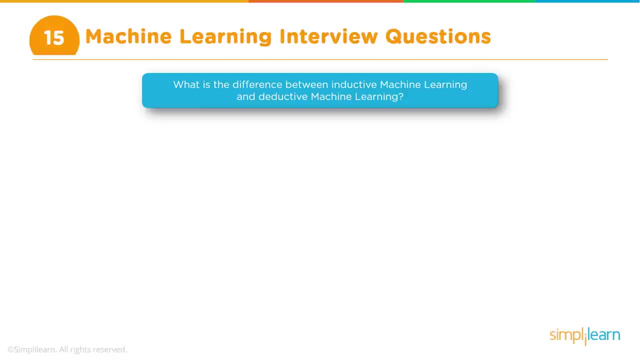 So the question can be: what is the difference between inductive machine learning and deductive machine learning, or somewhat the opposite? Okay, So the exact phrase or exact question can vary. They can ask for examples and things like that, but that could be the question. 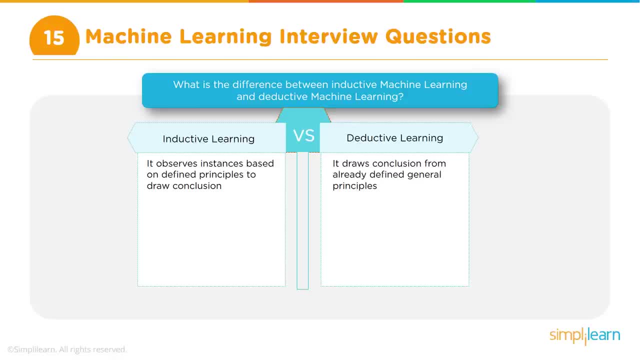 So let's first understand what is inductive and deductive training. Inductive training is induced by somebody And you can illustrate that with a small example. I think that always helps. So whenever you're doing some explanation, try as much as possible, as I said, 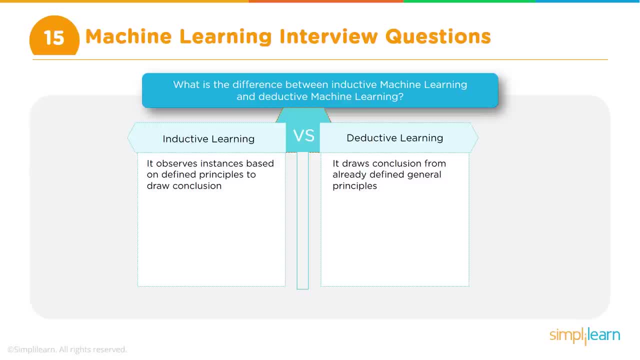 to give examples from your work experience or give some analogies, And that will also help a lot in explaining as well And for the interviewer also to understand. So here we'll take an example, or rather we will use an analogy. So inductive training is when we induce some knowledge or the learning process into a person. 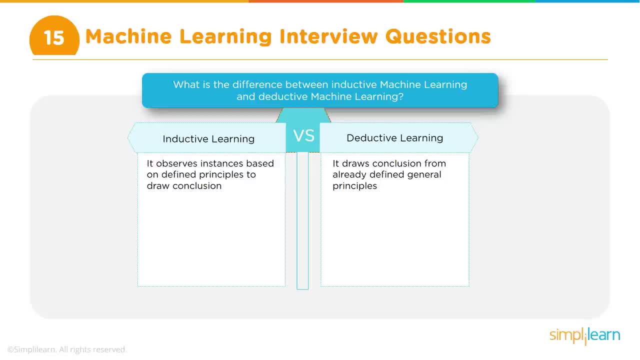 without the person actually experiencing it. Okay, What can be an example? So we can probably tell the person, or show a person a video- that fire can burn the thing, burn his finger, or fire can cause damage. So what is happening here? This person has never, probably seen a fire or never seen anything getting damaged by fire. 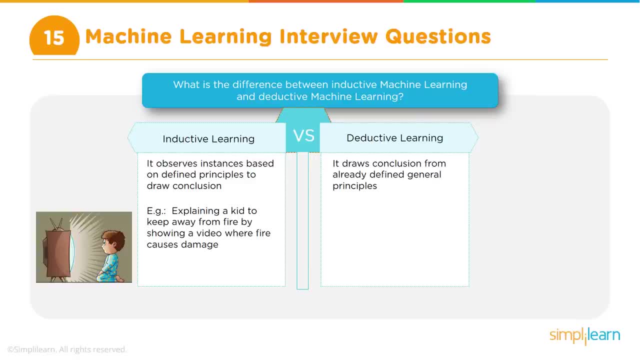 But just because he has seen this video, he knows that, okay, fire is dangerous, And if a fire can cause damage, right. So this is inductive learning compared to that, What is deductive learning? So here you draw conclusion, or the person draws conclusion out of experience. 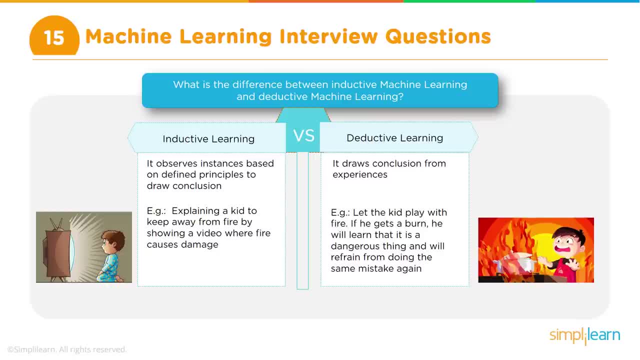 So we will stick to the analogy. So, compared to the showing of video, let's us: A person is allowed to play with fire, right? And then he figures out that if he puts his finger, it's burning, or if throw something into the fire, it burns. 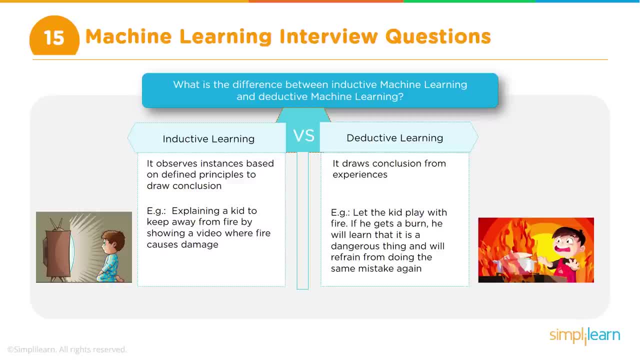 So he is learning through experience, So this is known as deductive learning. Okay, So you can have applications or models that can be trained using inductive learning or deductive learning. All right, I think probably that explanation will be sufficient. The next question is: are KNN and K-means? 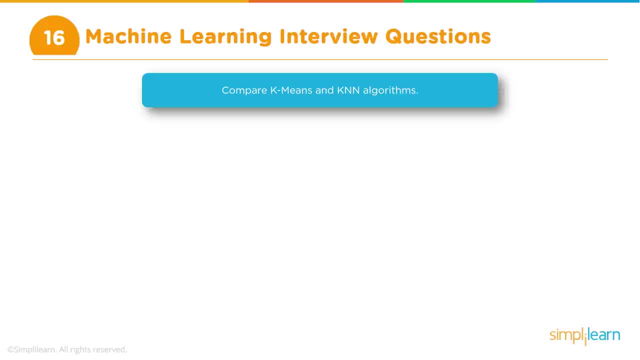 Clustering similar to one another, or are they same, right? Because the letter K is kind of common between them. Okay, So let us take a little while to understand what these two are. One is KNN and another is K-means. 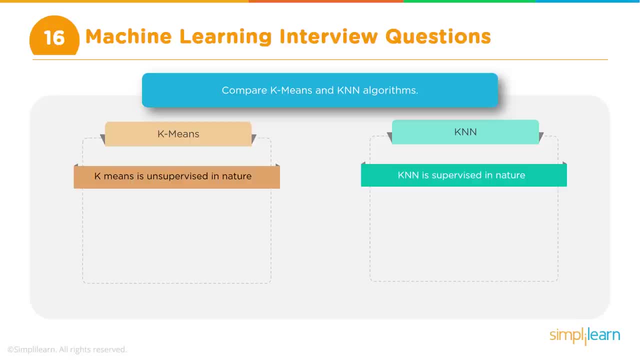 KNN stands for K- nearest neighbors- and K-means, of course, is the clustering mechanism. Now, these two are completely different, except for the letter K being common between them. KNN is completely different, K-means clustering is completely different, KNN. 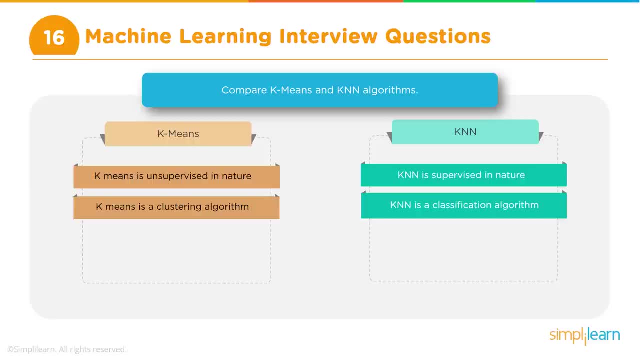 Is a classification process and therefore it comes under supervised learning, Whereas K-means clustering, is actually unsupervised. Okay, When you have KNN, when you want to implement KNN, which is basically K- nearest neighbors- the value of K is a number. 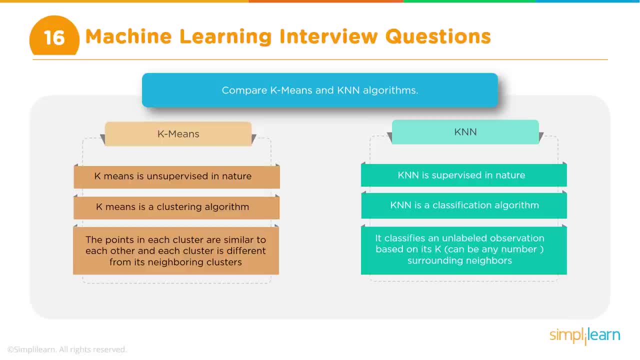 So you can say: K is equal to three. You want to implement KNN with K is equal to three, So, which means that it performs the classification in such a way that how does it perform the classification? So It will take three nearest objects and that's why it's called nearest neighbor. 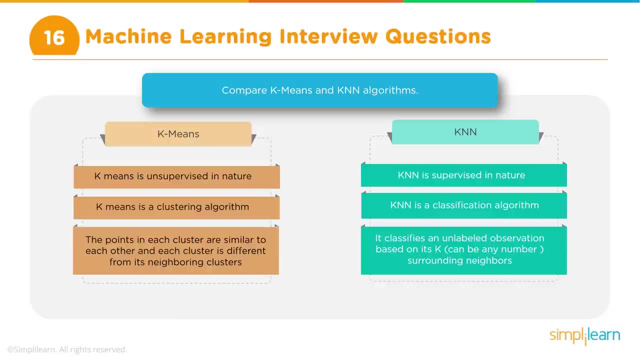 So basically, based on the distance, it will try to find out its nearest objects. that are three of the nearest objects, And then it will check whether the class they belong to which class. right. So if all three belong to one particular class, obviously this new object is also classified. 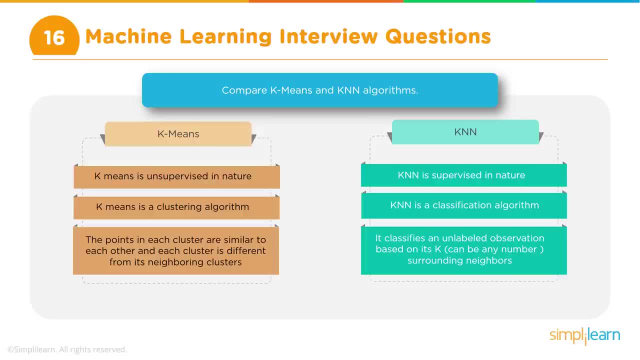 as that particular class, but it is possible that they may be from two or three different classes. Okay, So let's say they are from two classes And then, If they are from two classes, Now, usually you take a odd number, you assign odd number two. 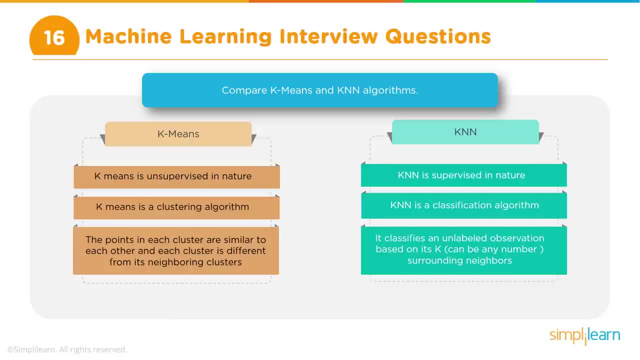 So if there are three of them and two of them belong to one class and then one belongs to another class, So this new object is assigned to the class to which the two of them belong. Now the value of K is sometimes tricky. whether should you use three? 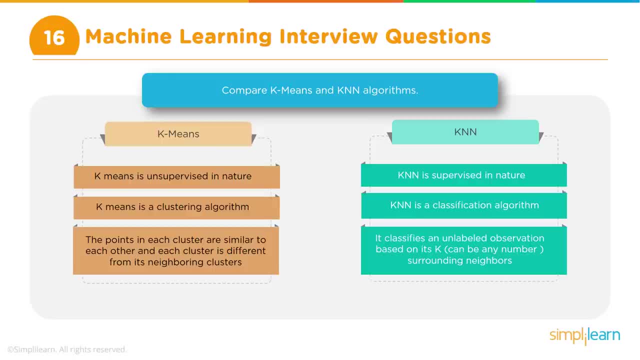 Should you use five? Should you use seven? That can be tricky because the ultimate classification can also vary. So it's possible that if you're taking K as three, the object is going to be three. The object is probably in one particular class. 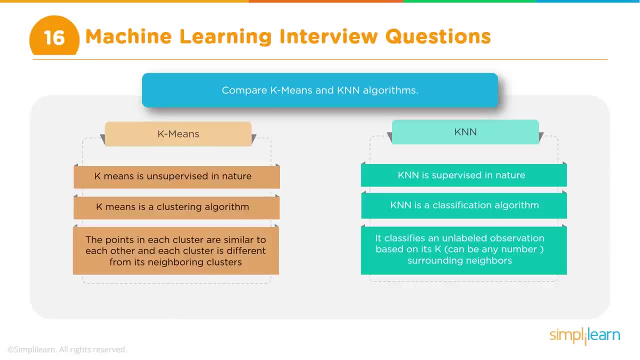 But if you take K is equal to five, maybe the object will belong to a different class, because when you're taking three of them, probably two of them belong to a class one and one belong to class two, Whereas when you take five of them, it is possible that only two of them belong to class. 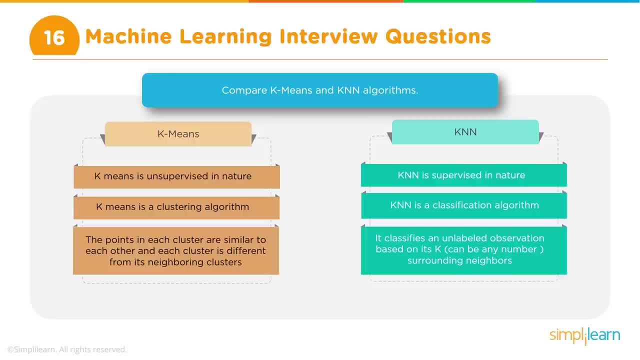 one and three of them belong to class two, So, which means that this object will belong to class two, right? So you see that. So it is. the class allocation can vary Depending on the value of K. now, K means, on the other hand, is a clustering process, and 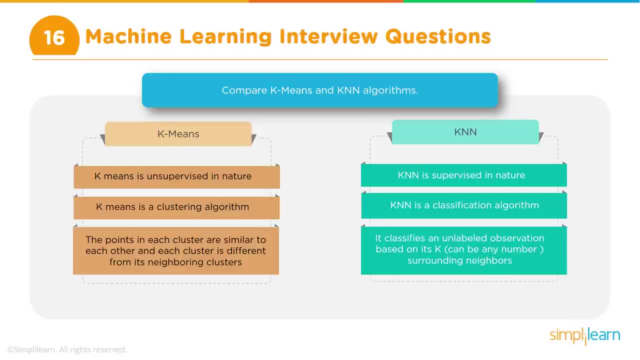 it is unsupervised, where what it does is the system will basically identify how the objects are, how close the objects are with respect to some of their features. Okay, And, but the similarity, of course, is the, the letter K, and in case of K, means also we. 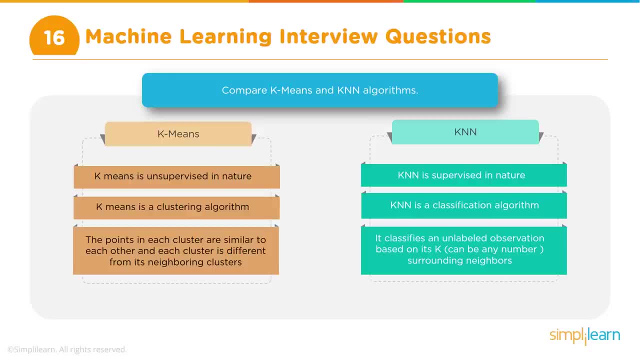 specify its value, and it could be three or five or seven. There is no technical limit as such, but it can be any number of clusters that you can create. Okay, So, based on the value that you provide, the system will create that many clusters of similar. 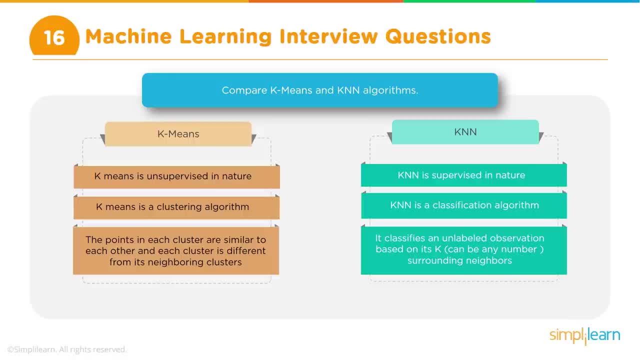 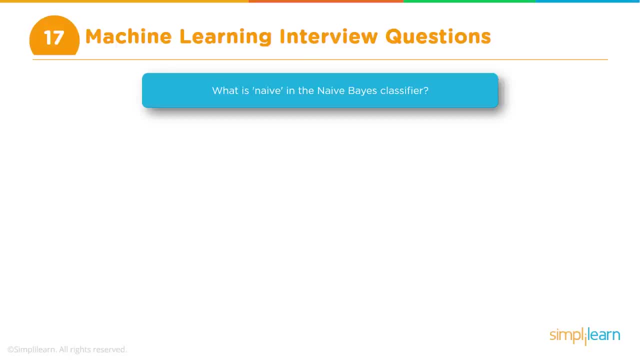 objects. So there is a similarity to that extent that K is a number in both the cases, but actually these two are completely different processes. We have what is known as naive base classifier, and people often get confused, thinking that naive base is the name of the person who found this classifier or who developed this classifier. 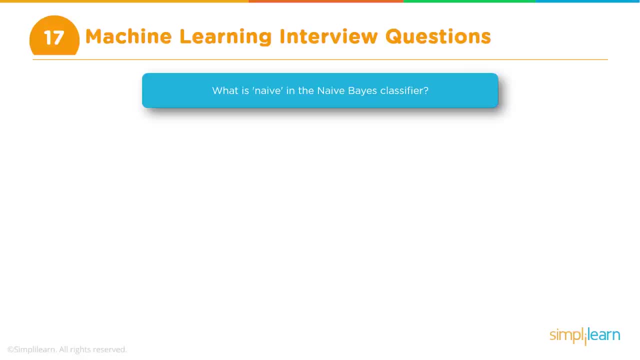 which is not a hundred percent true. Base is the name of the person, B A Y S is the name of the person, but naive is not the name of the person, right? So naive is basically an English word And that has been added here because of the nature of this particular classifier. 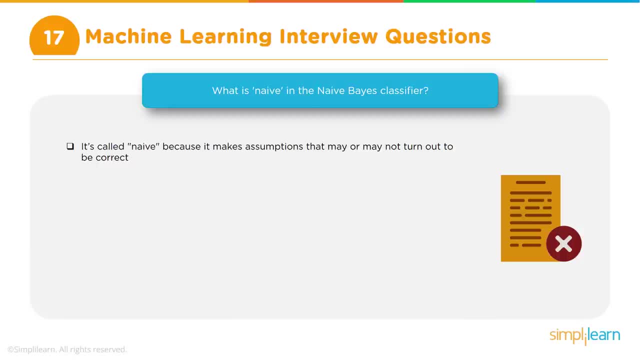 Naive base classifier is a probability based classifier And it makes some assumptions that presence of one feature of a class is not related to the presence of any other feature of maybe other classes, right, So, which is not a very, very strong or not a very, what do you say, accurate assumption, because these features 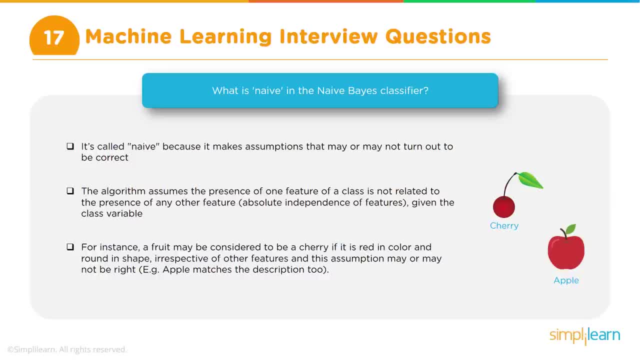 can be related and so on. But even if we go with this assumption, this whole algorithm works very well, even with this assumption, And that is the good side of it. But the term comes from that, So that is the explanation that you can. 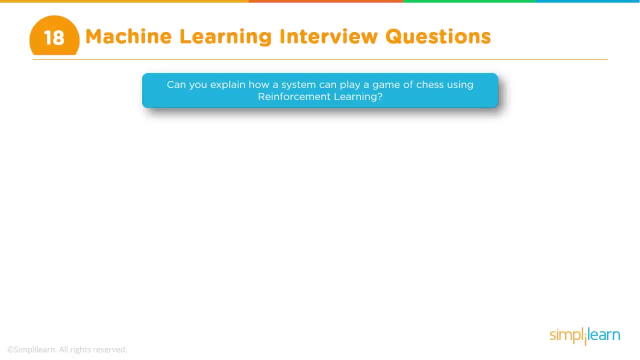 Then there can be question around reinforcement learning. It can be paraphrased in multiple ways. One could be: can you explain how a system can play a game of chess Using reinforcement learning, or it can be any game. So the best way to explain this is again to talk a little bit about what reinforcement 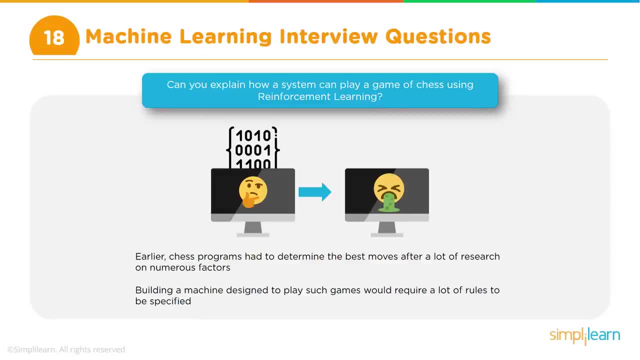 learning is about, and then elaborate on that to explain the process. So, first of all, reinforcement learning has an environment and an agent, and the agent is basically performing some actions in order to achieve a certain goal, And these goals can be anything either. if it is related to game, then the goal could. 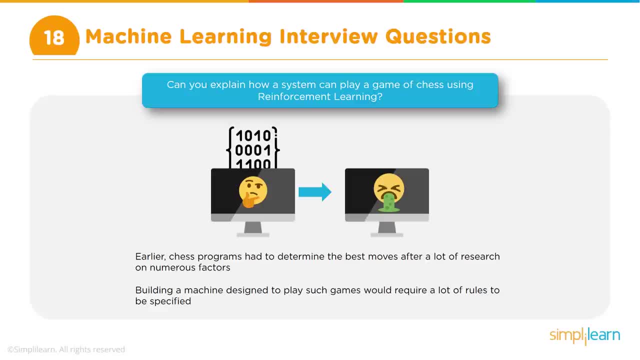 be that you have to score Very high. score high value, high number. or it could be that your number of lives should be as high as possible. Don't lose life. So these could be some of them. More advanced examples could be for driving the automotive industry, self-driving cars. 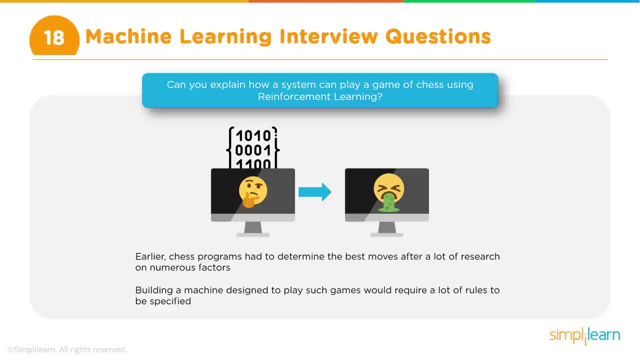 They actually also make use of reinforcement learning to teach the car how to navigate through the roads, and so on and so forth. That is also another example. Now, how does it work? So if the system is basically there is an agent And every time the agent takes a step or performs a task which is taking it towards the goal? 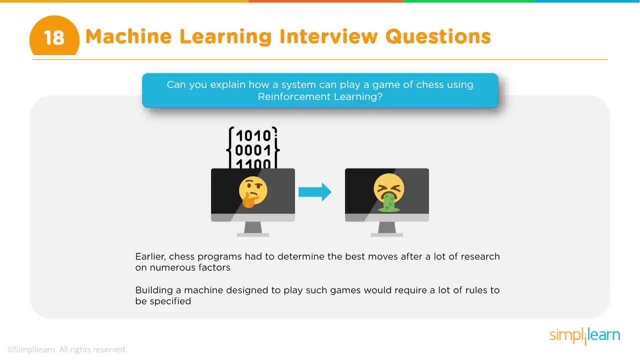 the final goal, let's say to maximize the score, or to minimize the number of lives and so on, or minimize the debts, for example, it is rewarded, And every time it takes a step which goes against that goal contrary or in the reverse. 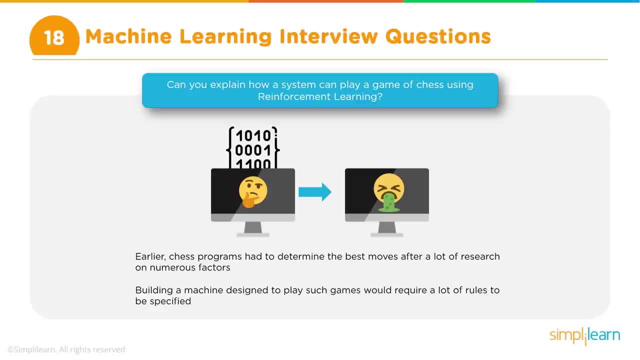 direction, it is penalized. Okay, So it is like a carrot and stick system. Now, how do you use this to create a game of chess? So, to create a system to play a game of chess. Now, the way this works is- and this could probably go back to this AlphaGo example- 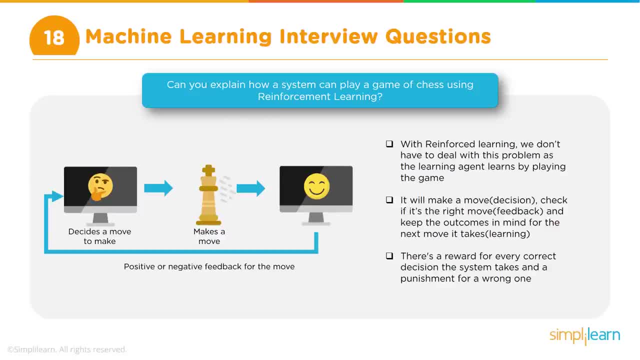 where AlphaGo defeated a human champion. So the way it works is in reinforcement learning the system is allowed. For example, in this case we are talking about chess, So we allow the system to first of all watch playing a game of chess. 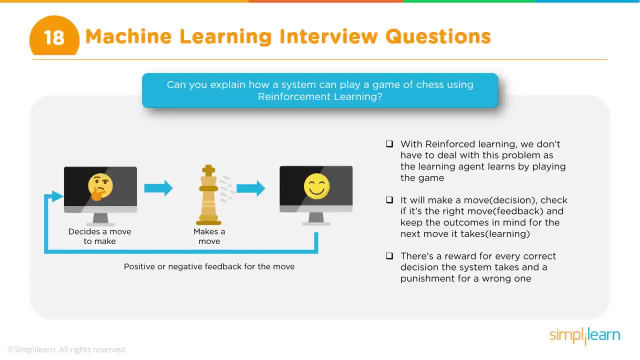 So it could be with a human being or it could be the system itself. There are computer games of chess, right, So Either this new learning system has to watch that game or watch a human being play the game, because this is reinforcement. learning is pretty much all visual. 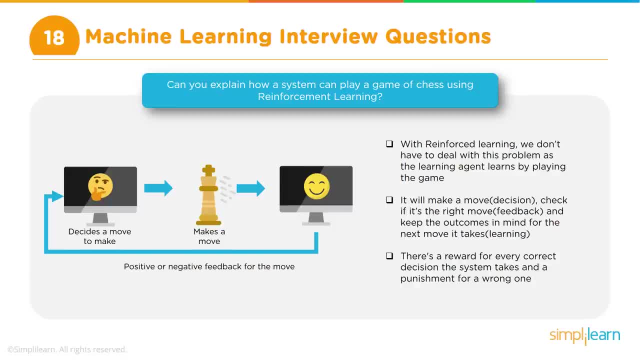 So when you're teaching the system to play a game, the system will not actually go behind the scenes to understand the logic of your software, of this game or anything like that. It is just visually watching the screen and then it learns. Okay, So reinforcement learning to a large extent works on that. 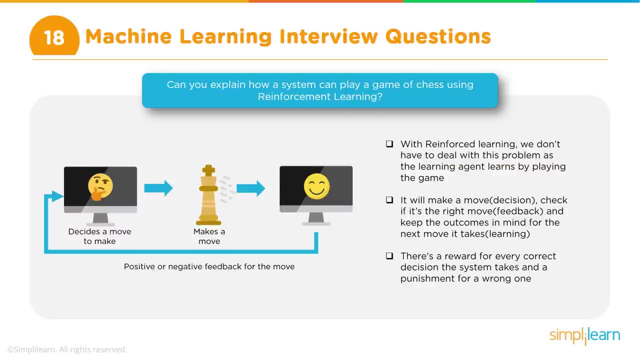 So you need to create a mechanism whereby your model will be able to watch somebody playing the game, and then you allow the system also to start playing the game. So it pretty much starts from scratch, Okay, And as it moves forward, it's right at the beginning. 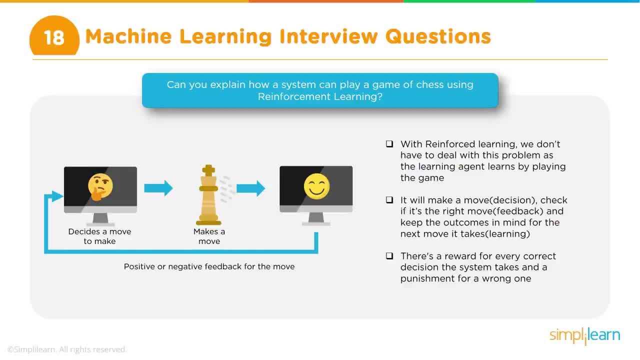 The system really knows nothing about the game of chess. Okay, So initially it is a clean slate. It just starts by observing how you're playing, So it will make some random moves and keep losing badly, But then what happens is over a period of time. 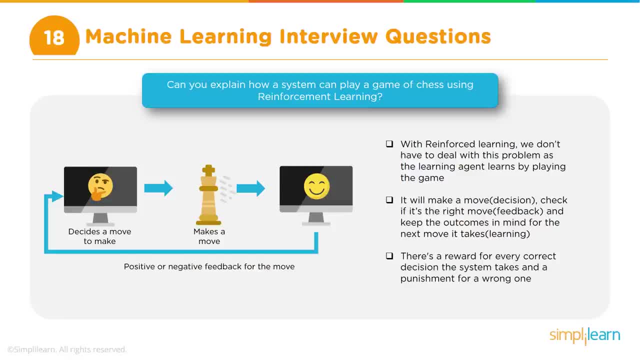 So you need to now allow the system or you need to play with the system, not just one, two, three, four or five times, but hundreds of times, thousands of times, maybe even hundreds of thousands of times, And that's exactly how AlphaGo has done. 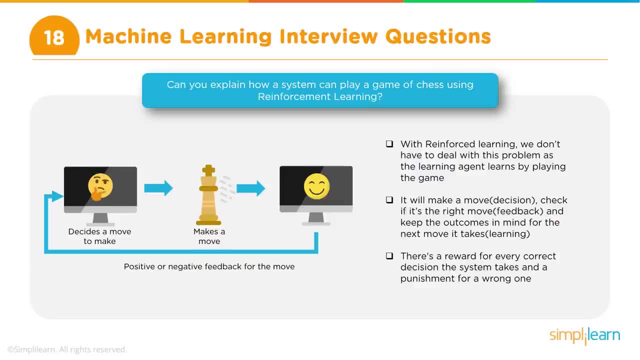 It played millions of games between itself and the system, right. So for the game of chess also, you need to do something like that. You need to allow the system to play chess and then learn on its own over a period of repetition. So I think you can probably explain it to this much, to this extent, and it should be. 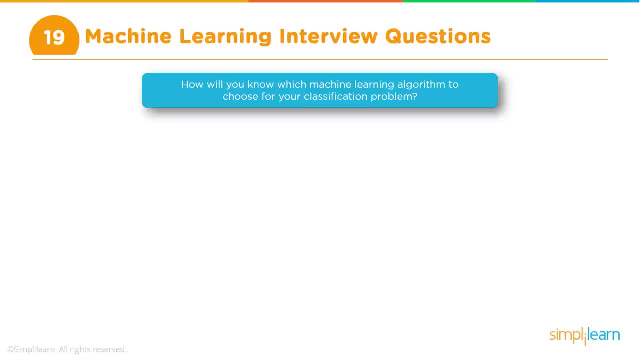 sufficient. Now this is another question which is again somewhat similar, but here the size is not coming into picture. So the question is: how will you know which machine learning algorithm to choose for your classification problem? Now, this is not only classification problem. 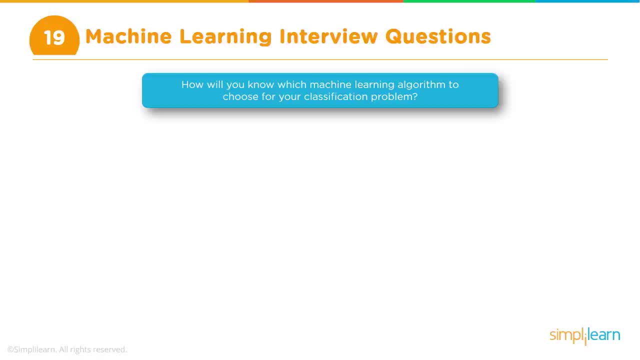 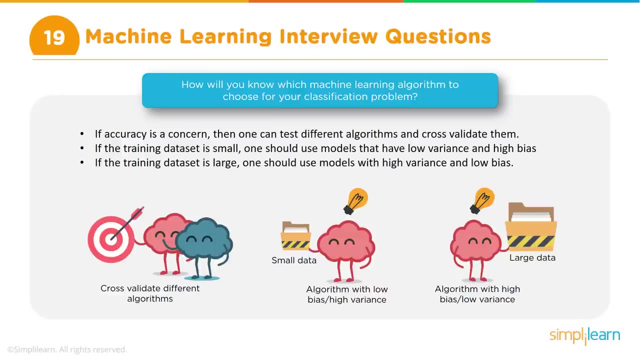 It could be a regression problem. I would like to generalize. Generalize this question. So if somebody asks you: how will you choose, How will you know which algorithm to use, The simple answer is: there is no way you can decide exactly, saying that this is the algorithm. 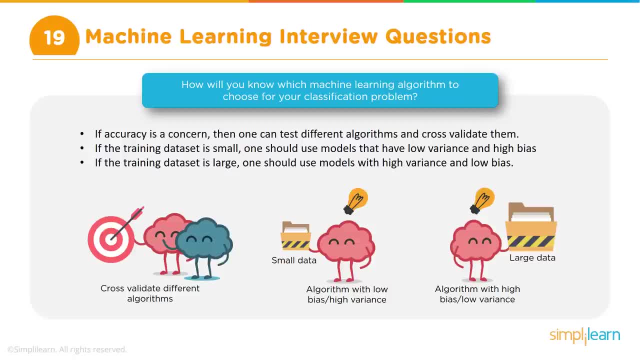 I'm going to use in a variety of situations. There are some guidelines like, for example: you will obviously, depending on the problem, you can say whether it is a classification problem or a regression problem And then, in that sense, you are kind of restricting yourself to if it is a classification problem. 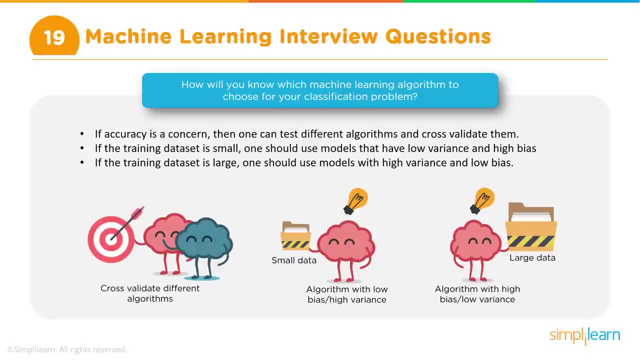 there are. You can only apply a classification algorithm right To that extent. you can probably, let's say, limit the number of algorithms. But now, within the classification algorithms, you have decision trees, you have SVM, you have logistic regression. 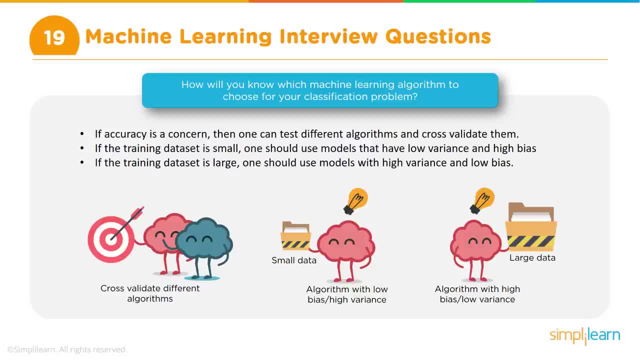 Is it possible to outright say yes for this particular problem, since you have explained this now, this is the exact algorithm that you can use. That is not possible. Okay, So we have to try out a bunch of algorithms, See which one gives us the best. 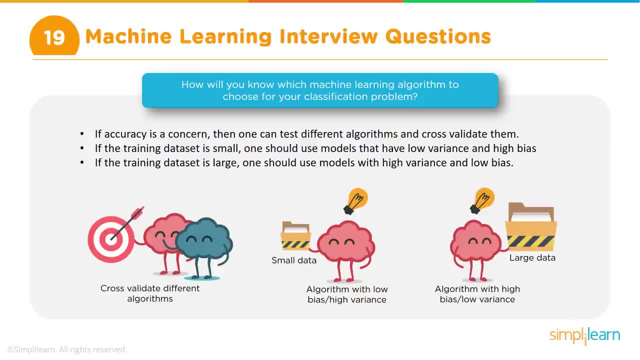 Performance and best accuracy and then decide to go with that particular algorithm. So in machine learning a lot of it happens through trial and error. There is no real possibility that anybody can, just by looking at the problem or understanding the problem, tell you that okay, in this particular situation this is exactly the 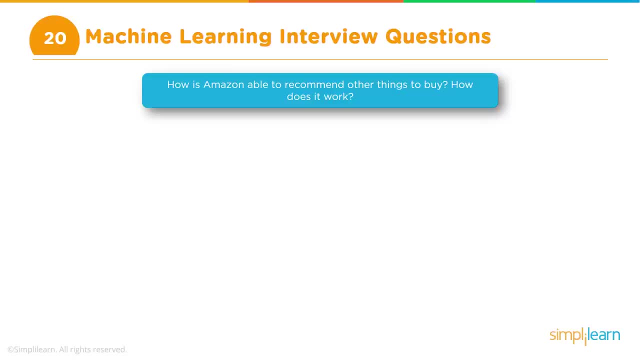 algorithm that you should use, Then the questions may be around application of machine learning, And this question is specifically around how Amazon is able to recommend other things to buy. So this is around recommendation engine. How does it work? How does the recommendation engine work? 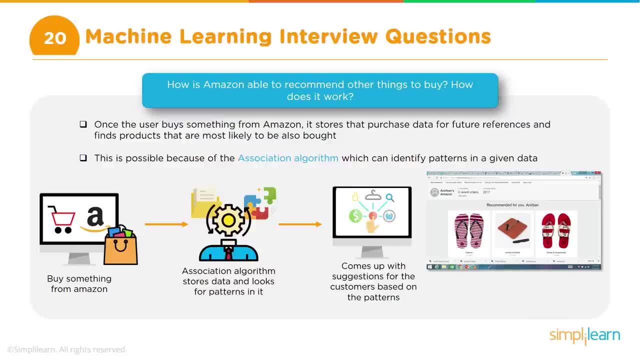 So this is basically the question is all about. So the recommendation engine again works based on various inputs that are provided. Obviously, something like you know, Amazon, a website or e-commerce site like Amazon collects a lot of data around the customer behavior: who is purchasing what, and if somebody is. 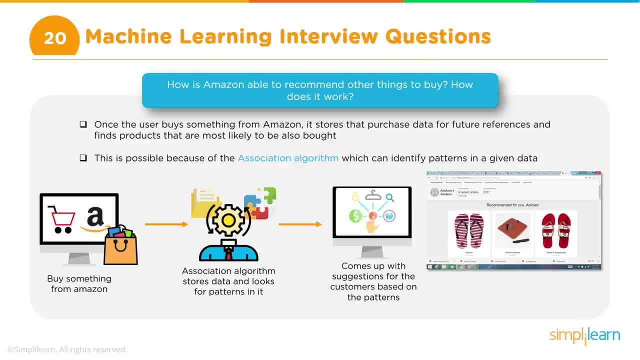 buying a particular thing, they're also buying something else. So This kind of association, right. So this is the unsupervised learning we talked about. They use this to associate and link or relate items, And that is one part of it. 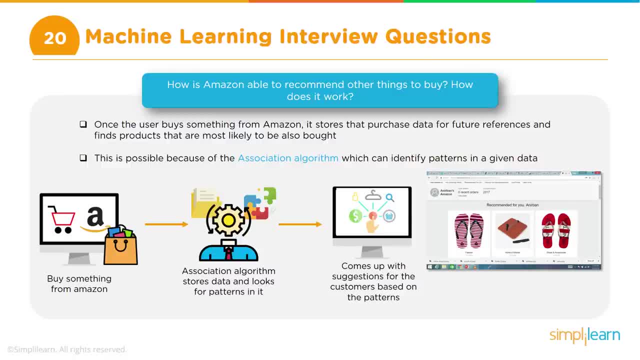 So they kind of build association between items, saying that somebody buying this is also buying this. That is one part of it. Then they also profile the users right Based on their age, their gender, their geographic location. they will do some profiling. 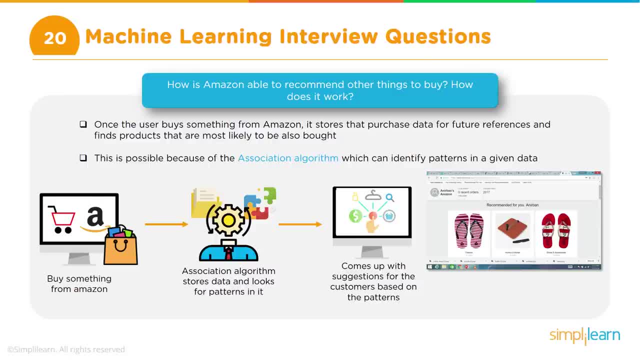 And then when somebody is logging in and when somebody is Shopping, kind of the mapping of these two things are done. They try to identify. obviously, if you have logged in, then they know who you are and your information is available, Like, for example, your age, maybe your gender, and where you're located, what you purchased. 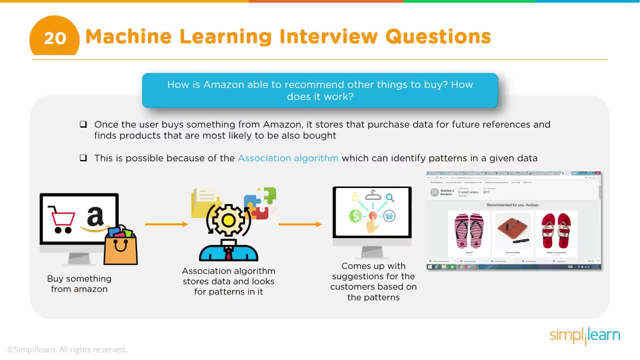 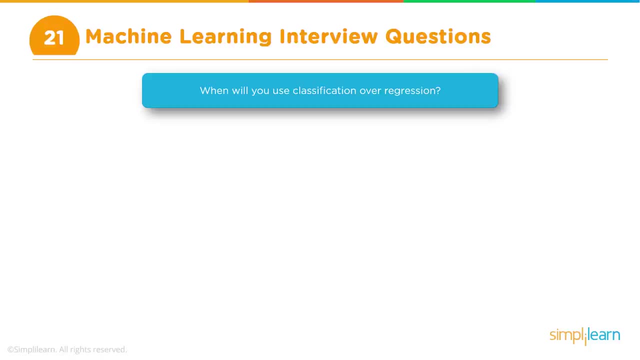 earlier, right? So all this is taken and the recommendation engine basically uses all this information and comes up with recommendations for a particular user. So that is how the recommendation engine works, All right. Then the question can be something very basic Like: when will you go for classification versus regression, right? 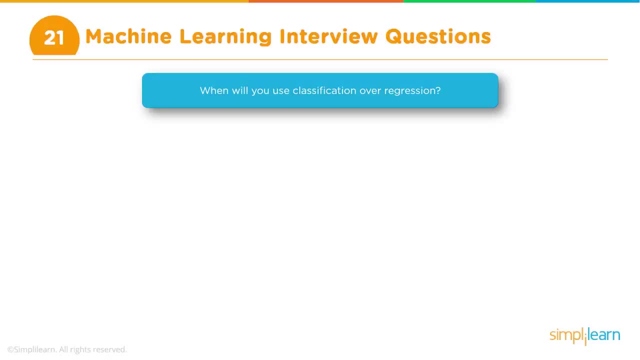 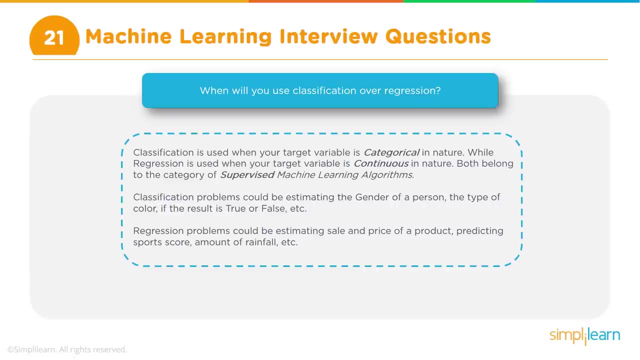 When do you do classification instead of regression, Or when do you use classification instead of regression? Now, Yes, sir. So this is basically going back to the understanding of the basics of classification and regression. So classification is used when you have to identify or categorize things into discrete. 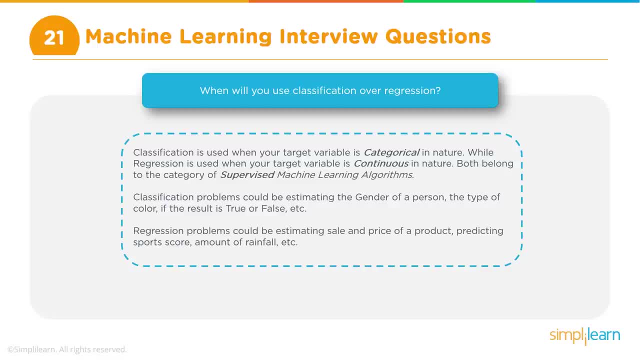 classes. So the best way to respond to this Question is to take up some examples and use it. Otherwise it can become a little tricky. The question may sound very simple, but explaining it can sometimes be very tricky. In case of regression we use, of course there will be some keywords that they will 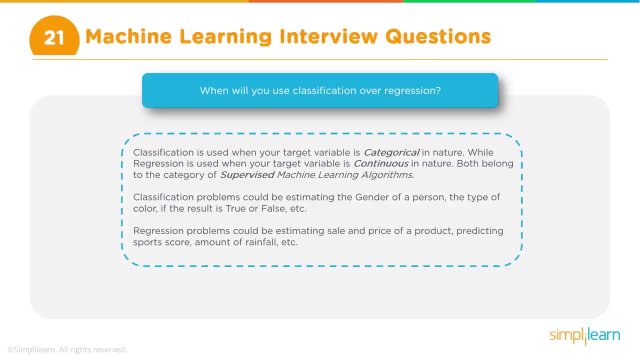 be looking for. So it's just you need to make sure you use those keywords. One is the discrete values, Another is the continuous values. So for regression, if you're trying to find some continuous values, you use regression, Whereas if you're trying to find some discrete values, you use classification and then you 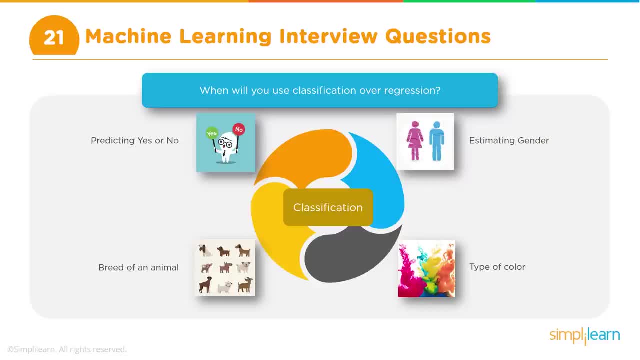 need to illustrate what are some of the examples. So classification is like, let's say, there are images and you need to put them into classes like cat, dog, elephant, tiger, something like that. So that is a classification problem. Or it can be that is a multi-class classification problem. 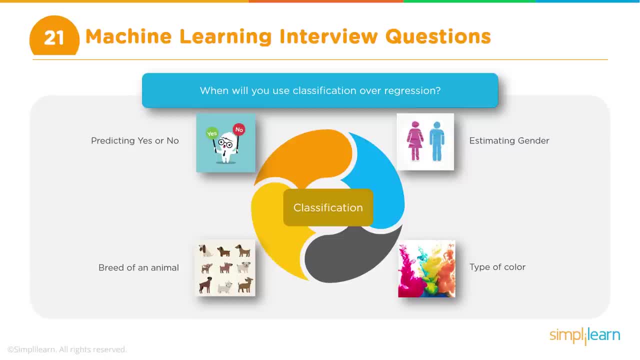 It could be binary classification problem, Like for example, whether a customer will buy or he will not buy. That is a classification, binary classification. It can be in the weather forecast Forecast area. Now weather forecast is again combination of regression and classification because on 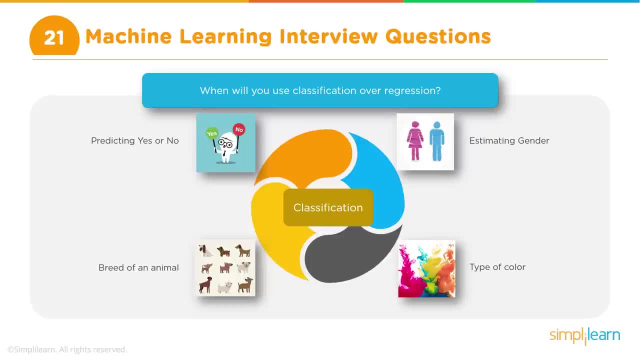 the one hand, you want to predict whether it's going to rain or not. That's a classification problem. That's a binary classification, right? Whether it's going to rain or not rain. However, you also have to predict what is going to be the temperature tomorrow, right? 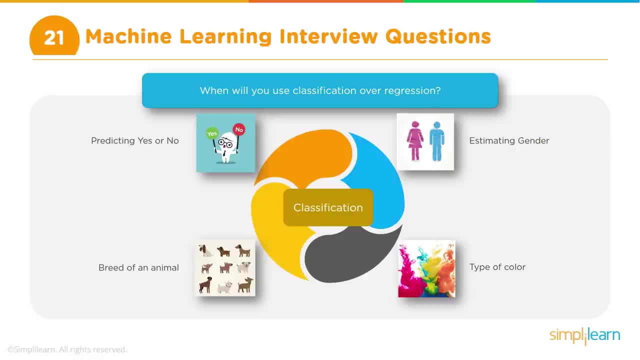 Now, temperature is a continuous value. You can't answer the temperature in a yes or no kind of a response, right? So what will be the temperature tomorrow? So you need to give a number which can be like 20 degrees, 30 degrees or whatever, right? 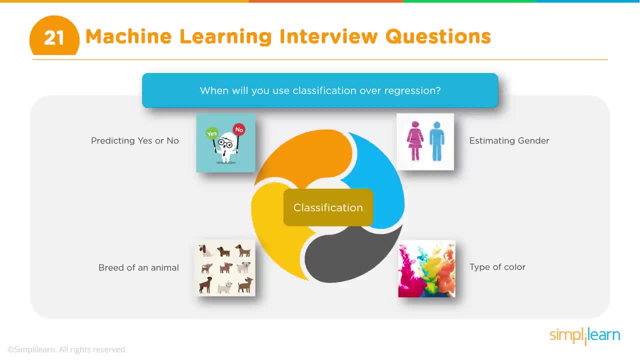 So that is where you use regression. One more example is stock price prediction, So that is where, again, you will use regression. So these are the various examples. So you need to illustrate with examples and make sure you include those keywords like discrete and continuous. 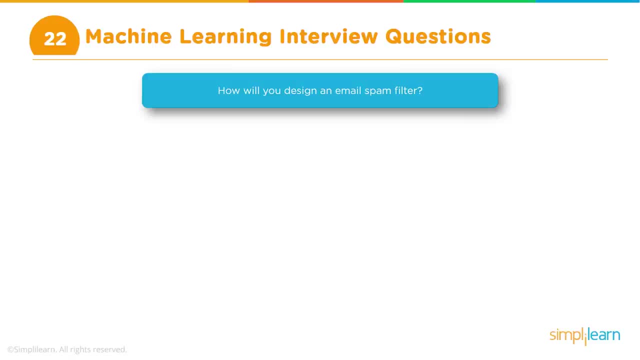 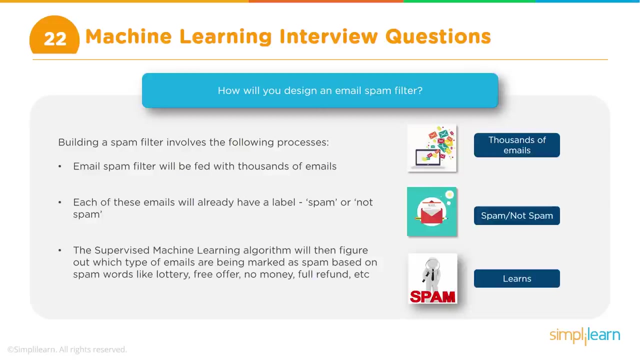 So the next question is more about a little bit of a design related question to understand your concepts and things like that. So it is: how will you design a spam filter? So how do you basically design Or develop a spam filter? So I think the main thing here is he's looking at probably understanding your concepts in 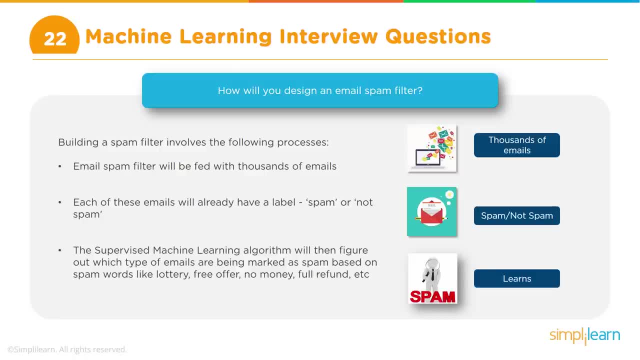 terms of what is the algorithm you will use or what is your understanding about difference between classification and regression and things like that. right, And the process, of course, the methodology and the process. So the best way to go about responding to this is we say that, okay, this is a classification. 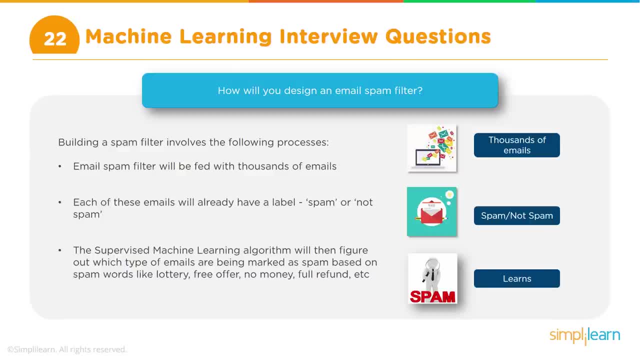 problem, because we want to find out whether an email is a spam or not Spam so that we can apply the filter accordingly. So first thing is to identify what type of a problem it is. So we have identified that it is a classification. Then the second step may be to find out what kind of algorithm to use. 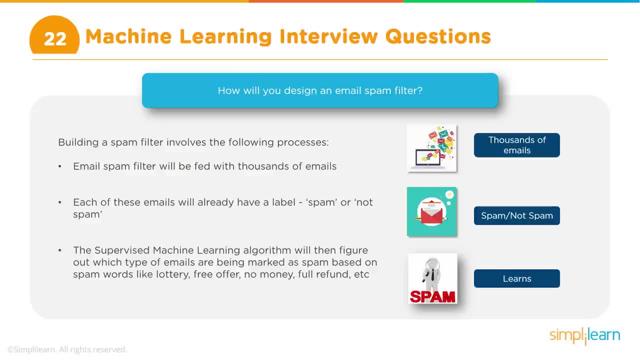 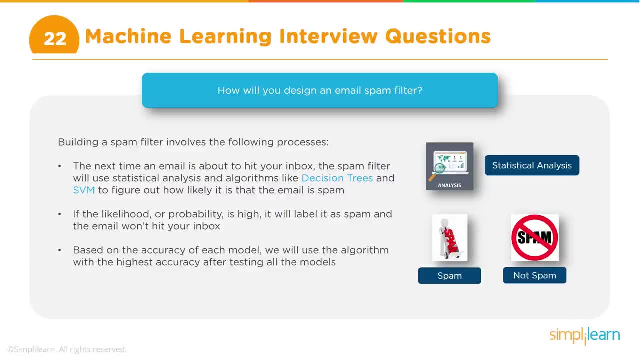 Now, since this is a binary classification problem, logistic regression is a very common, very common algorithm, But however right as I said earlier also, we can never say that okay, for this particular problem, this is exactly the algorithm that we can use. 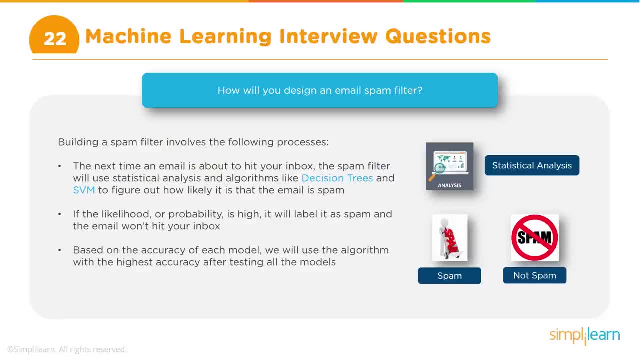 So we can also probably try Decision trees or even support vector machines, for example SVM. So we will kind of list down a few of these algorithms and we will say, okay, we want to, we would like to try out these algorithms. 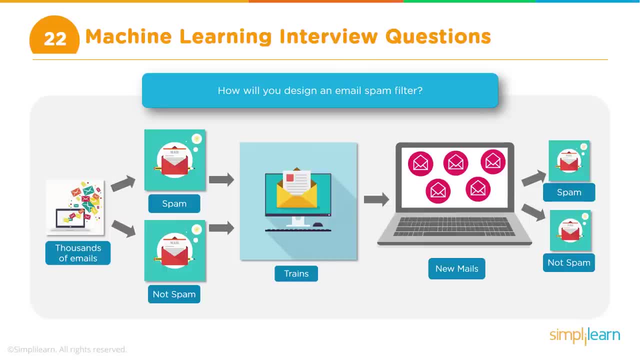 And then we go about taking your historical data, which is the labeled data which are marked, So you will have a bunch of emails- and then you split that into training and test data sets. You use your training data set to train your model, that or your algorithm. 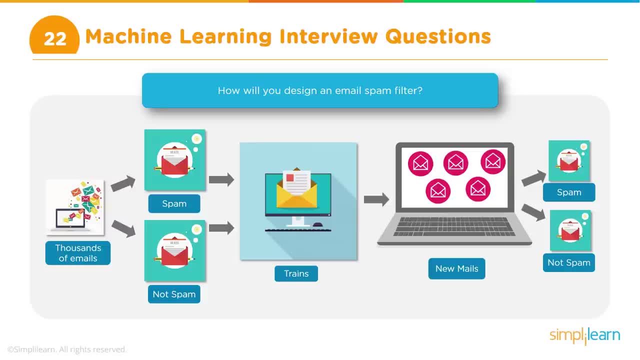 That you have used rather the model actually. So and you actually will have three models. Let's say, you are trying to test out three algorithms, So you will obviously have three models. So you need to try all three models and test them out as well. 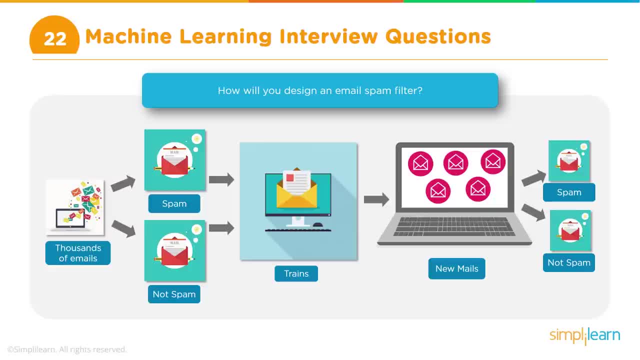 See which one gives the best accuracy, And then you decide that you will go with that model. Okay, So training and tests will be done, and then you zero in on one particular model And then you say, okay, this is the model we'll use. 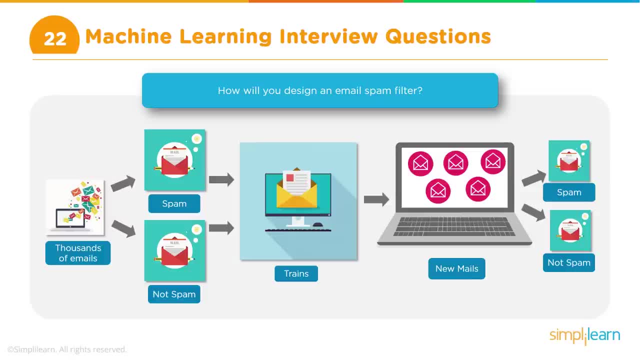 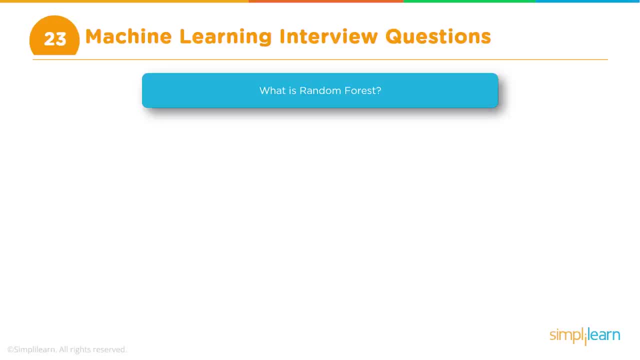 We will use and then go ahead and implement that Or put that in production. So that is the way you design a spam field. The next question is about random forest. What is random forest? So this is a very straightforward question. However, the response: you need to be again a little careful. while we all know what is, 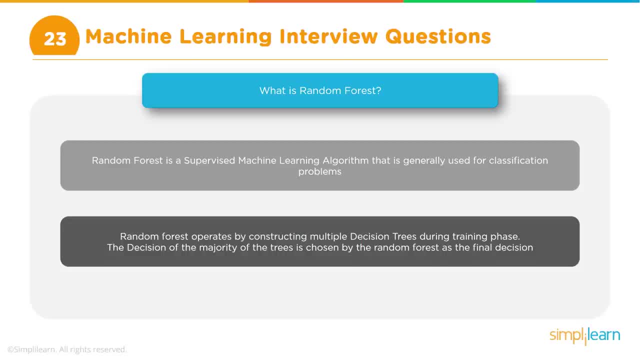 random forest. explaining this can sometimes be tricky. So one thing is random forest is kind of, in one way it is an extension of decision trees, because it is basically nothing but you have multiple decision trees And trees will basically you will use for doing if it is classification, mostly it. 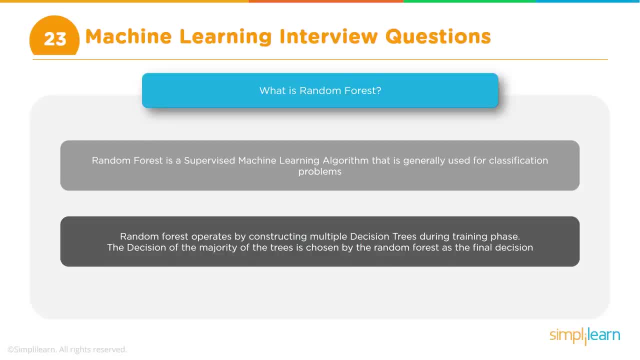 is classification. you will use the trees for classification and then you use voting for finding that the final class. So that is the underlines. but how will you explain this? How will you respond to this? So, first thing, obviously we will say that random forest is one of the algorithms and 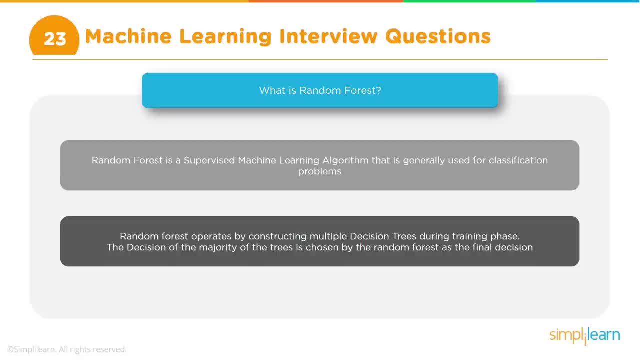 the more important thing that you need to- probably the interviewer is is waiting to hear- is ensemble learner, right? So this is one type of ensemble. Now, what is ensemble learner? Ensemble learner is like a combination of algorithms, So it is a learner which consists of more than one algorithm, or more than one maybe. 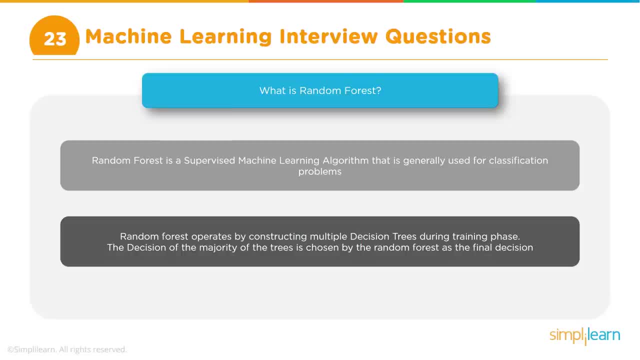 models. Okay, So in case of random forest, algorithm is the same, but instead of using one instance of it, we use multiple instances of it, and we use So in a way that is, a random forest is an ensemble learner. There are other types of ensemble learners where we have, like we use different algorithms. 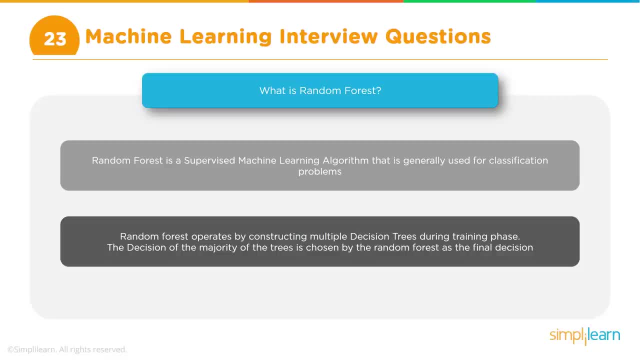 itself. So you have one, maybe logistic regression and a decision tree combined together, and so on and so forth. or there are other ways, like, for example, splitting the data in a certain way, and so on. So that's all about ensemble. 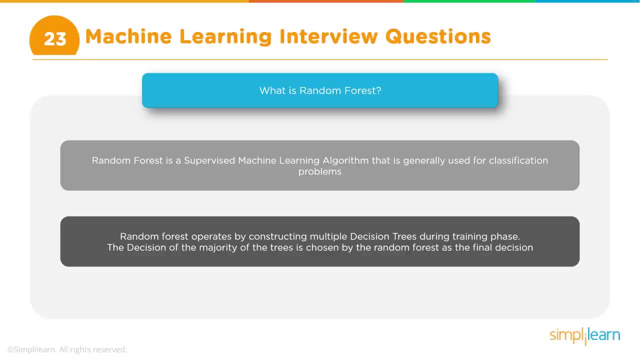 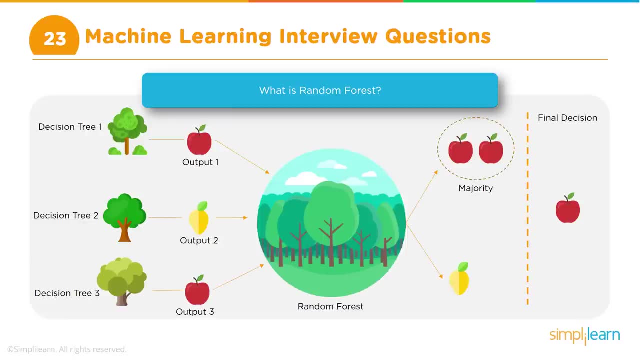 We will not go into that, but random forest itself. I think the interviewer will be happy to hear this word: ensemble learner. And so then you go and explain how the random forest works. So if the random forest is used for classification, then we use what is known as a voting mechanism. 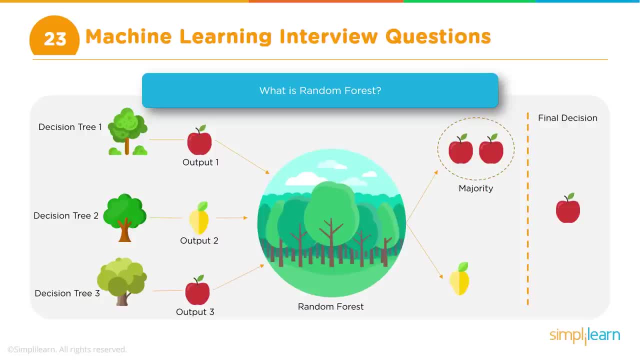 So basically, how does it work? Let's say your random forest Consists of hundred trees and each observation you pass through this forest and each observation. let's say it is a classification problem, binary classification, zero or one, and you have hundred trees. 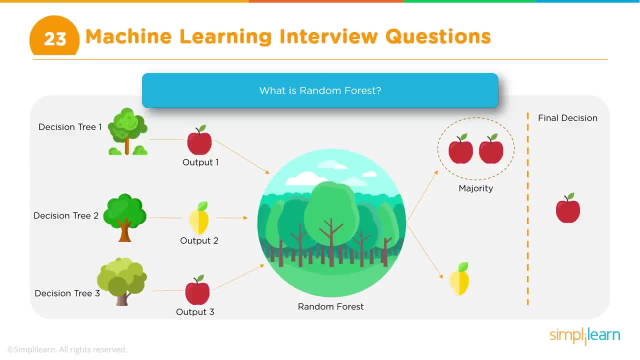 Now, if 90 trees say that it is a zero and 10 of the trees say it is a one, you take the majority, You may take a vote And since 90 of them are saying zero, you classify this as zero. 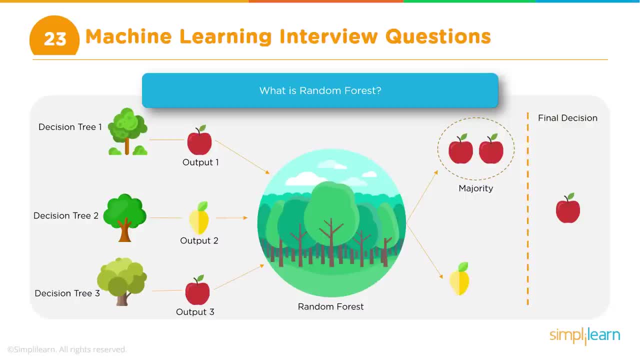 Then you take the next observation and so on. So that is the way a random forest works for classification. If it is a regression problem, it's somewhat similar, but only thing is, instead of vote, what we will do is in regression, Remember what happens. 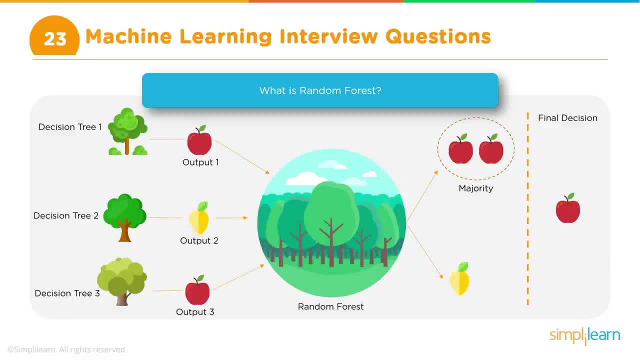 You actually calculate a value right. So, for example, you're using regression to predict the temperature and you have hundred trees and each tree obviously will probably predict a different value of the temperature. They may be close to each other, but they may not be exactly the same value. 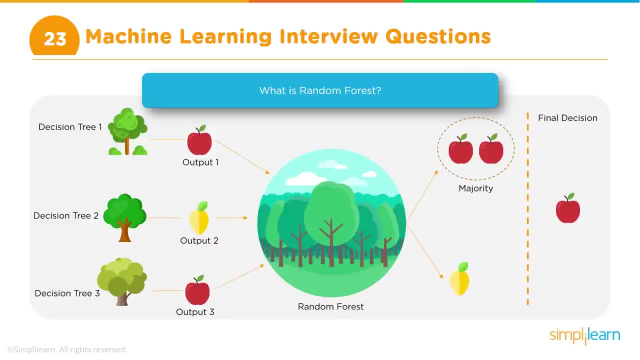 So these hundred trees? So how do you now find the actual value, The output For the entire forest right? So you have outputs of individual trees which are a part of this forest, but then you need to find the final output of the forest itself. 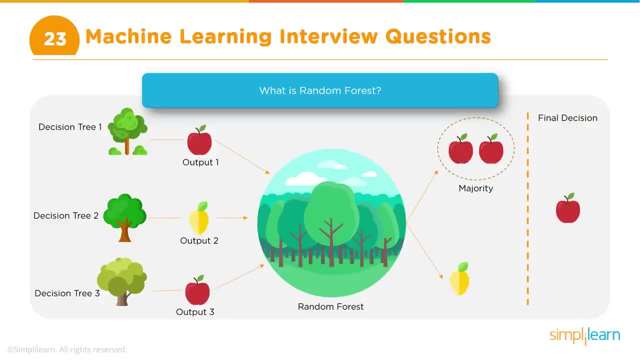 So how do you do that? So in case of regression, you take like an average or the mean of all the hundred trees, right? So this is also a way of reducing the error. So maybe if you have only one tree and if that one tree makes a error, it is basically. 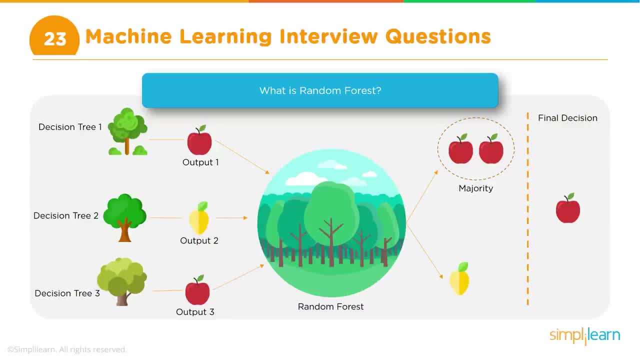 a hundred percent wrong or a hundred percent right, right, But if you have, on the other hand, if you have a bunch of trees, you are basically basically mitigating that error, reducing that error. Okay, So that is the way random forest works. 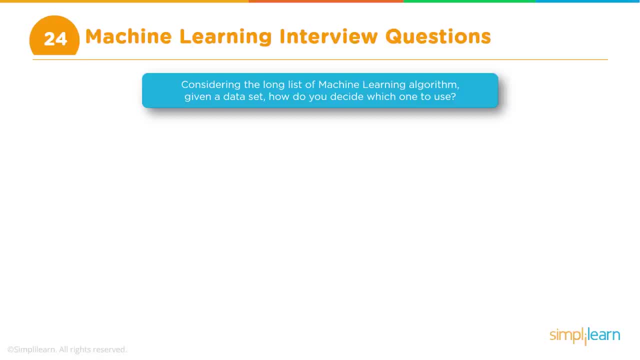 So the next question is: considering the long list of machine learning algorithms, How will you decide on which one to use? So once again here, there is no way to outright say that this is the algorithm that we will use for a given data set. 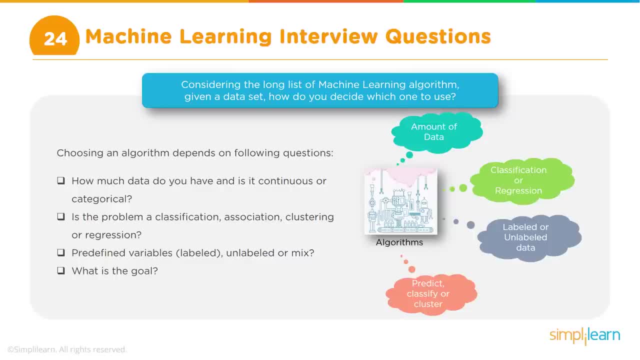 This is a very good question, but then the response has to be like again: there will not be a one size fits all, So we need to. First of all, you can probably shorten the list in terms of by saying, okay, whether 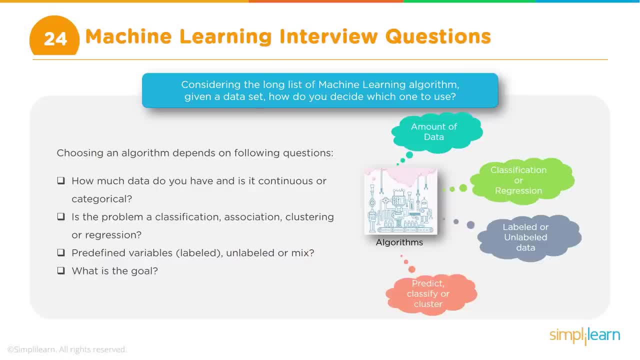 it is a classification problem or it is a regression problem. To that extent you can probably shorten the list, because you don't have to use all of them. If it is a classification problem, you only can pick from the classification algorithms, right? 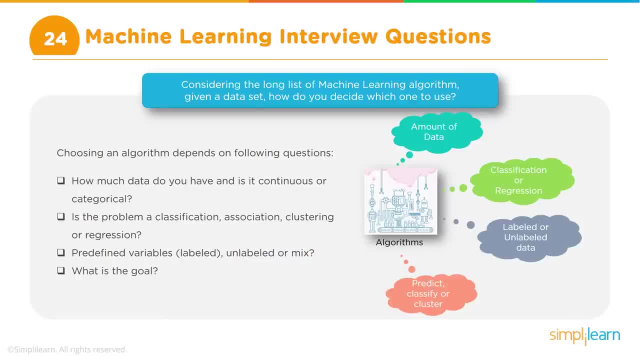 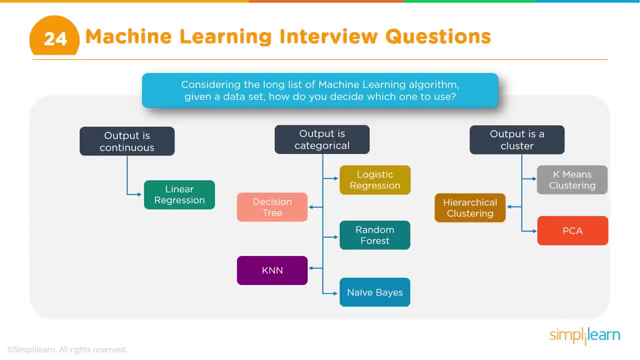 So, for example, if it's a classification, you cannot use linear regression algorithm, or if it is a regression problem, you cannot use SVM. or maybe no, you can use SVM, but maybe a logistic regression right. So to that extent you can probably shorten the list, but still you will not be able. 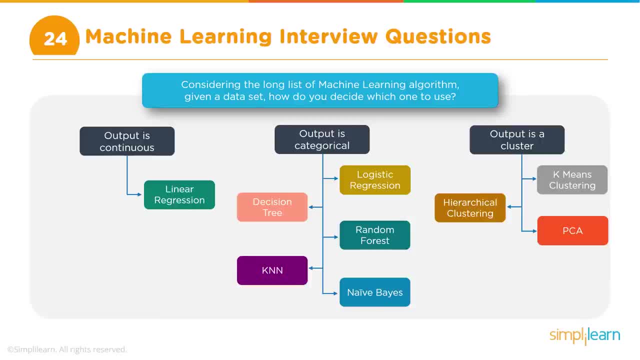 to a hundred percent, decide on saying that this is the exact algorithm that I'm going to use. So the way to go about is you choose a few algorithms based on what the problem is. You try out your data, you train some models of these algorithms, check which one gives. 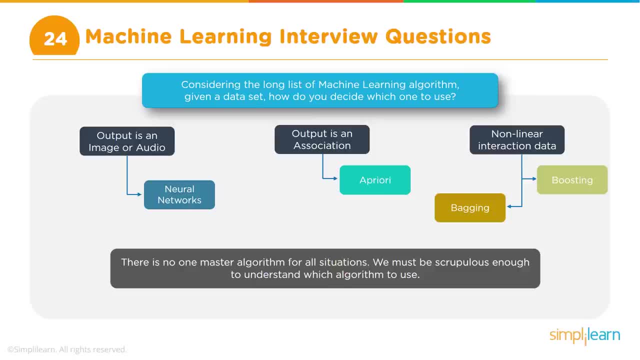 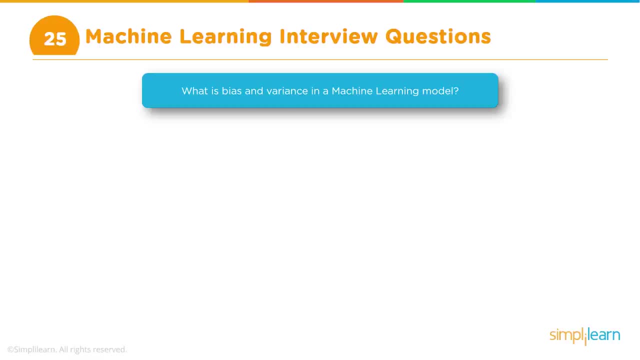 you the lowest error or the highest accuracy And based on that you choose that particular algorithm. Okay, All right. Then There can be questions around bias and variance. So the question can be: what is bias and variance in machine learning? 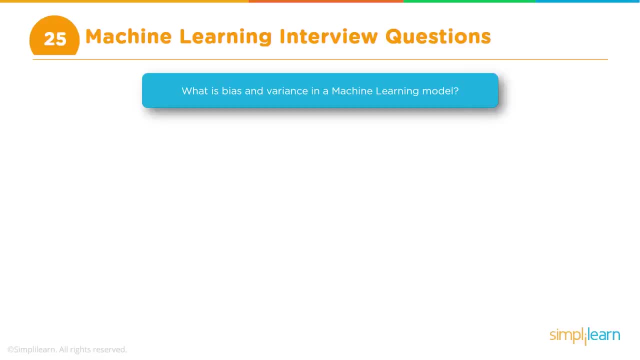 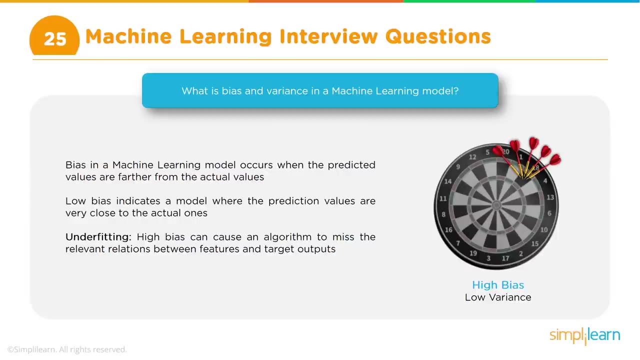 So you just need to give out a definition for each of these. For example, a bias. in machine learning, it occurs when the predicted values are far away from the actual value. So that is a bias, Okay. And whereas they are all, all the values are probably they are far off, but they are very. 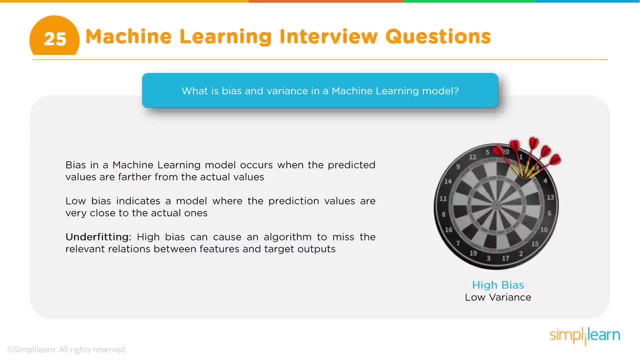 near to each other, though The predicted values are close to each other, right, While they are far off from the actual value, But they are close to each other. You see the difference. So that is bias, And then the other part is your variance. 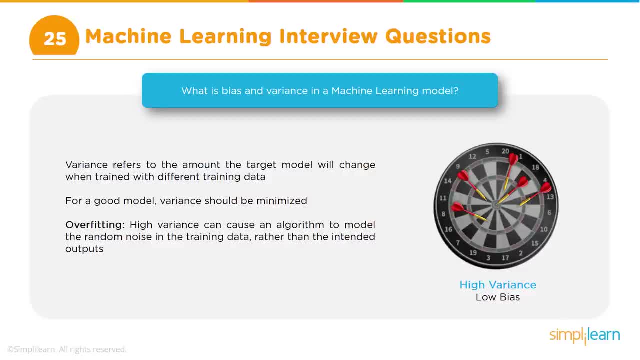 Now, variance is when the predicted values are all over the place, right. So the variance is high. That means it may be close to the target, but it is kind of very scattered. So the point: the predicted values are not close to each other, right. 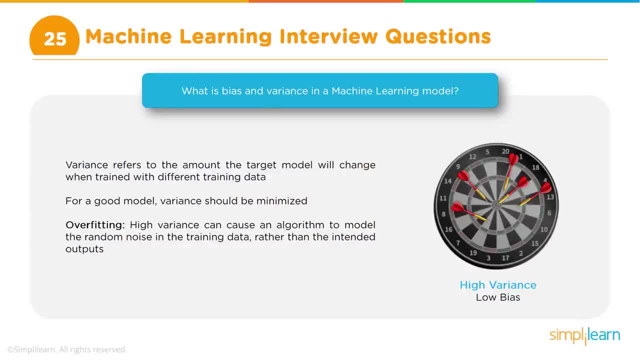 In case of bias, the predicted values are close to each other, but they are not close to the target. but here they may be close to the target, but they may not be close to each other, So they are a little bit more scattered. 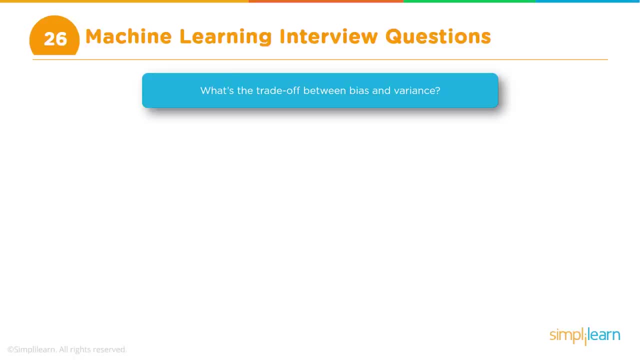 So that is what in case of variance? Okay, Then the next question is about, again related to bias and variance. What is the trade off between bias and variance? Yes, I think this is a interesting question, because these two are heading in different directions. 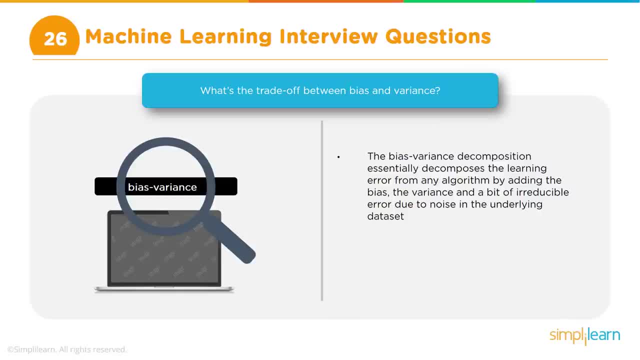 So, for example, if you try to minimize the bias, variance will keep going high, And if you try to minimize the variance, bias will keep going high and there is no way you can Minimize both of them. So you need to have a trade off saying that, okay, this is the level at which I will have. 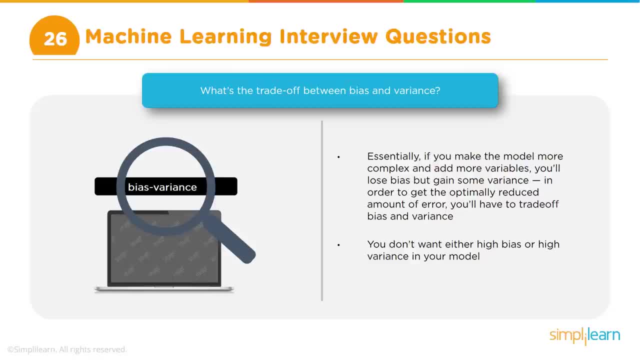 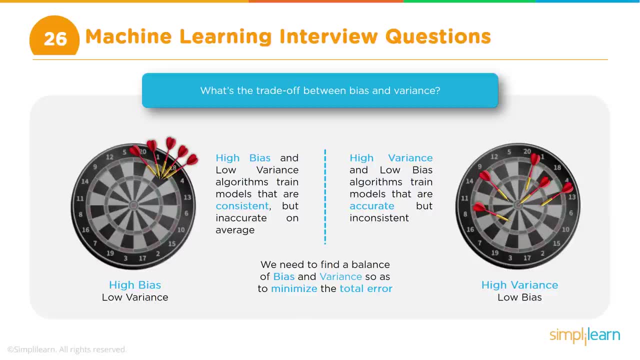 my bias and this is the level at which I will have variance. So the trade off is that, pretty much, that you decide what is the level you will tolerate for your bias and what is the level you will tolerate for variance, and a combination of these two, in such a way that your final results are not way off and having a trade off will. 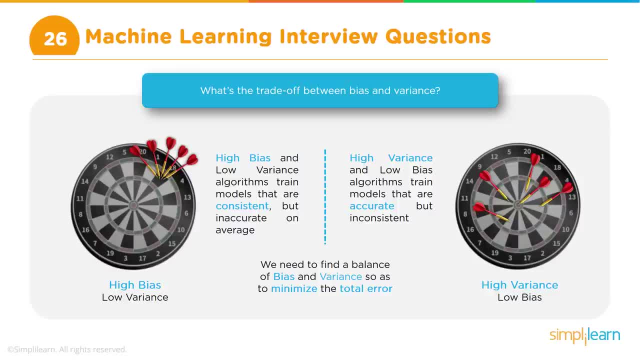 ensure that the results are consistent, right? So That is basically: the output is consistent, and which means that they are close to each other and they are also accurate, but that means they are as close to the target as possible, right? So if either of these is high, then one of them will go off the track. 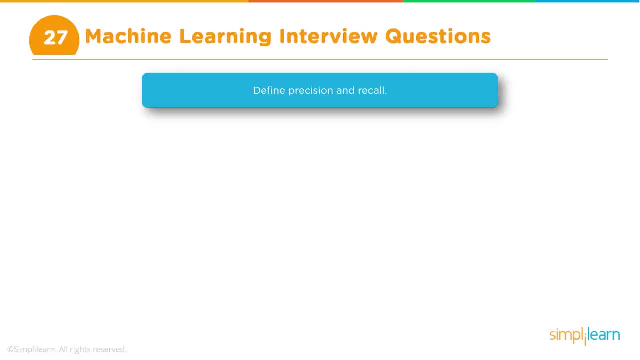 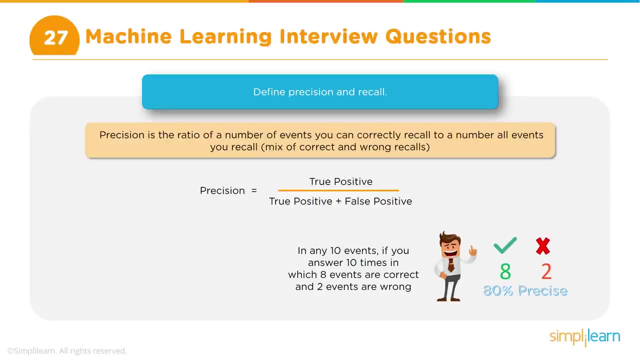 Define precision and recall Now again here I think it would be best to draw a diagram and take a confusion matrix. and it is very simple. The definition is like a formula: Yeah, Your precision is true positive by true positive plus false positive. 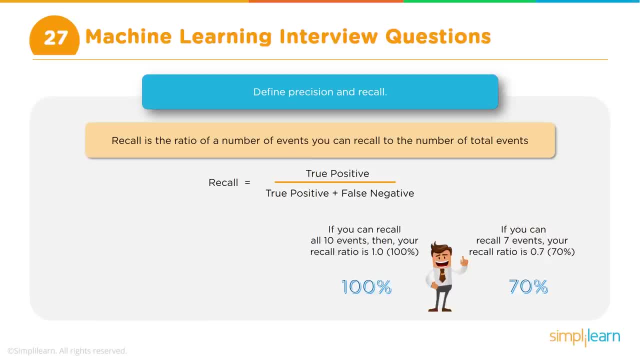 And your recall is true positive by true positive plus false negative. Okay, So that's, you can just show it in a mathematical way. That's pretty much. you know that can be shown. That's the easiest way to define. So the next question can be about decision tree. 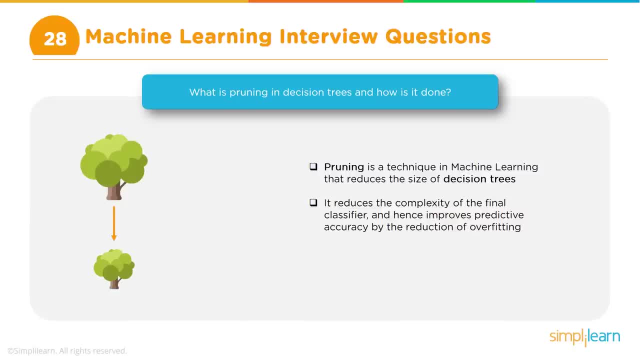 What is decision tree pruning and why is it So? basically, decision trees are really Simple to implement and understand, but one of the drawbacks of decision trees is that it can become highly complicated as it grows right, And the rules and conditions can become very complicated. 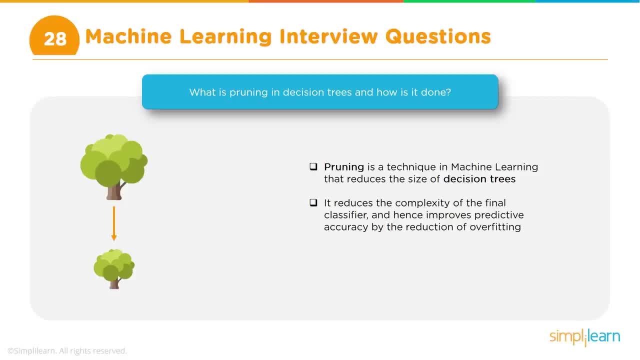 And this can also lead to overfitting, which is basically that during training you will get a hundred percent accuracy, but when you're doing testing you'll get a lot of errors. So that is the reason pruning needs to be done. 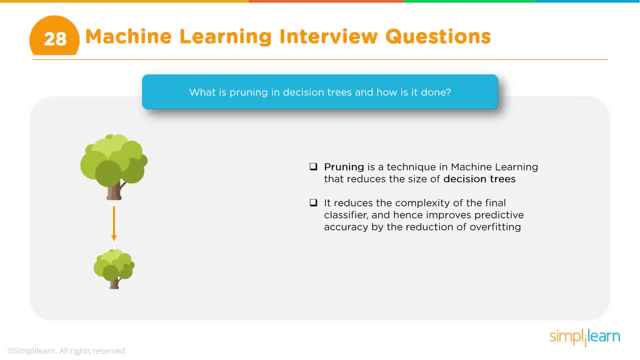 So the purpose or the reason for doing, Uh decision tree pruning is to reduce overfitting or to cut down on overfitting. And what is decision tree pruning? It is basically that you reduce the number of branches because, uh, as you may be aware, 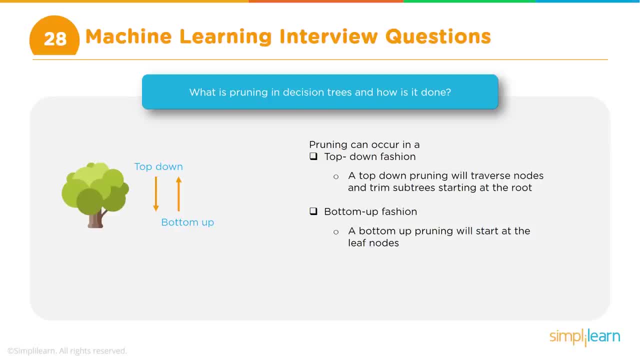 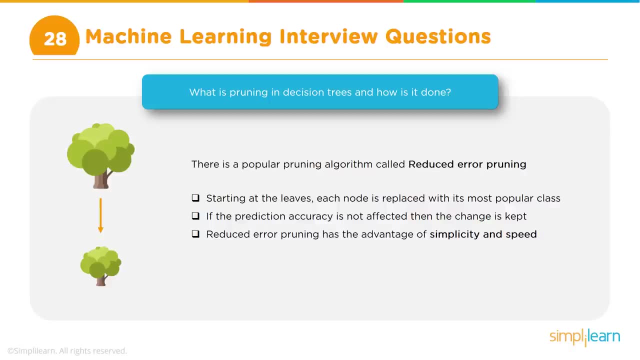 a tree consists of the root node, and then there are several internal nodes, and then you have the leaf nodes. Now, if there are too many of these internal nodes, that is when you face the problem of overfitting, and pruning is the process of reducing those internal nodes. 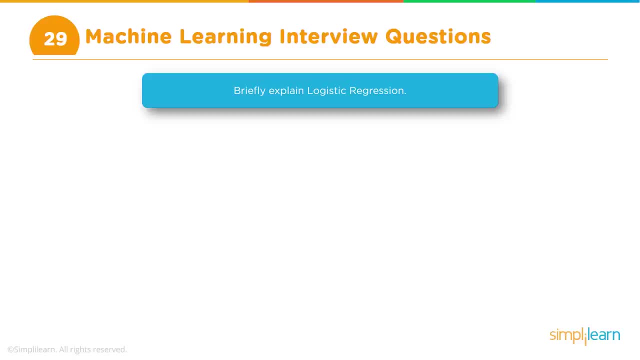 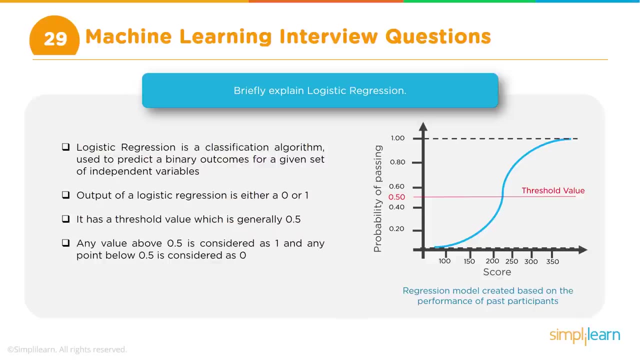 Okay, All right. So the next question can be: what is logistic regression? So, basically, logistic regression is one of the techniques used for performing classification, especially binary classification. Now there is something special about logistic regression, and there are a couple. 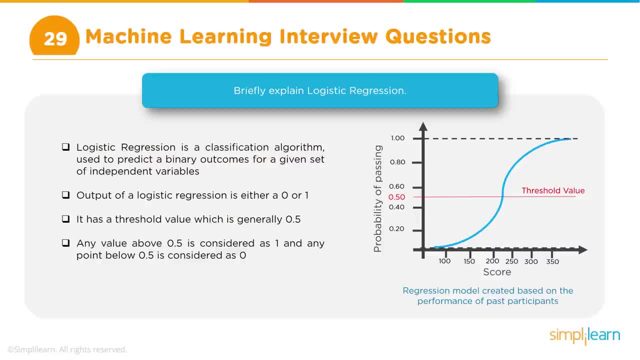 of things you need to be careful about. First of all, the name is a little confusing. It is called logistic regression but it is used for classification, So this can be sometimes confusing. So you need to probably clarify that to the interviewer, if it's really you know. 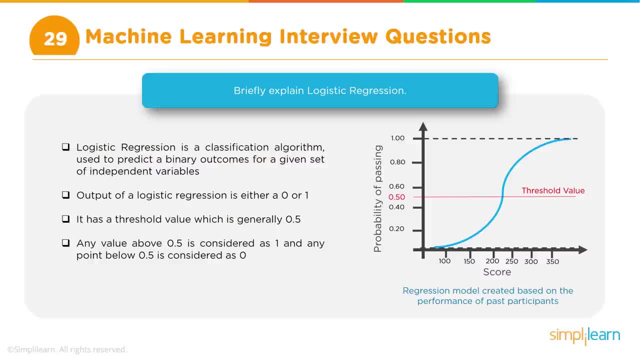 if it is required, And they can also ask this like a trick question, right? So that is one part. Second thing is the term logistic has nothing to do with the usual logistics that we talk about, but it is derived from log, So that the mathematical derivation was log and therefore 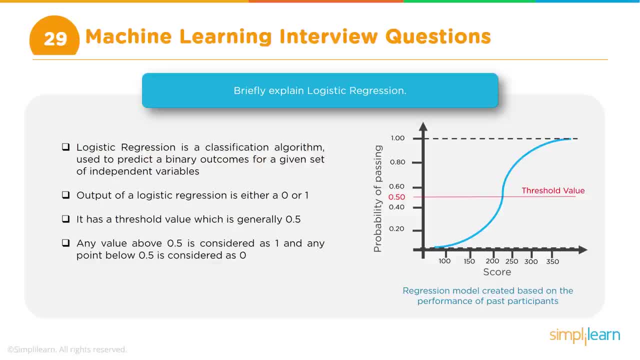 the name logistic regression. So what is logistic regression and how is it used? So logistic regression is used for binary classification and the output of a logistic regression is either a 0 or a 1, and it varies. So it's basically: it calculates a probability between 0 and 1,. 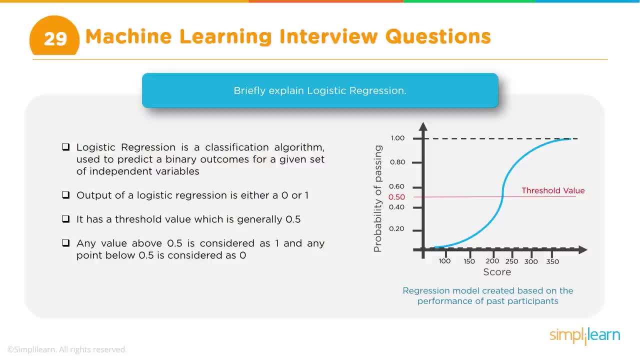 and we can set a threshold that can vary. Typically it is 0.5.. So any value above 0.5 is considered as 1, and if the probability is below 0.5, it is considered as 1.. So if the 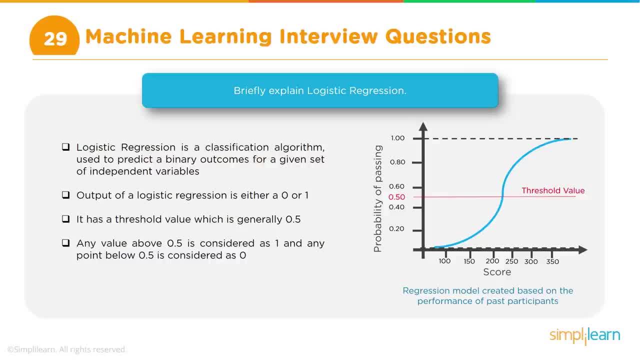 probability is below 0.5, it is considered as 0. So that is the way we calculate the probability, or the system calculates the probability and, based on the threshold, it sets a value of 0 or 1, which is like a binary classification- 0 or 1.. Okay, then we have a question around. 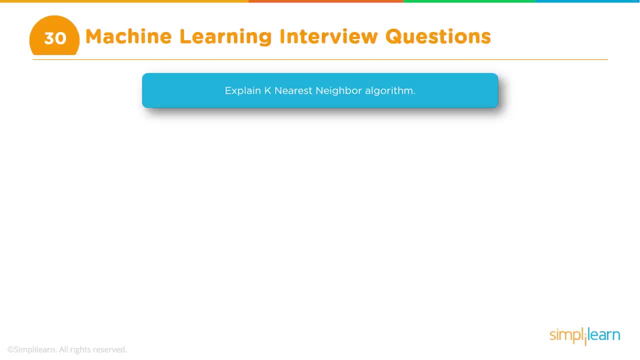 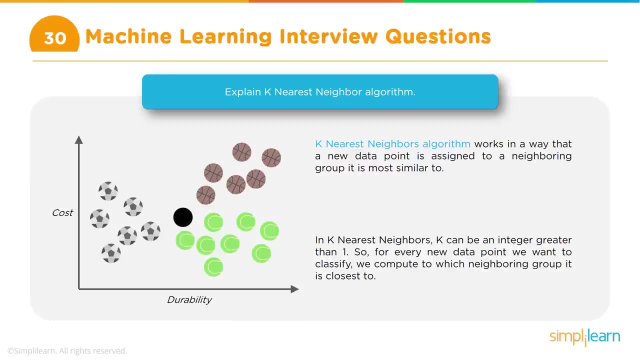 k-nearest neighbor algorithm. So explain k-nearest neighbor algorithm. So, first of all, what is a k-nearest neighbor algorithm? This is a classification algorithm. So that is the first thing we need to mention, And we also need to mention that. 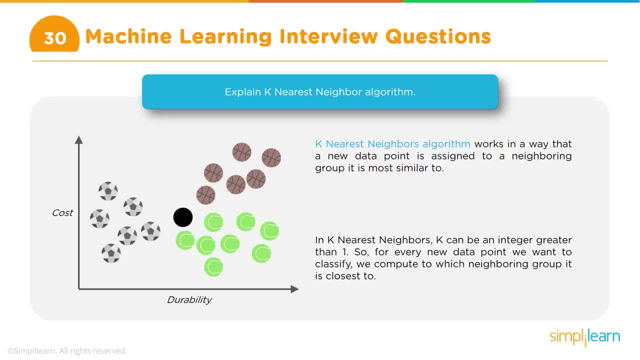 the k is a number, it is an integer and this is variable and we can define what the value of k should be. It can be 2,, 3,, 5,, 7, and usually it is an odd number. So that is something we need to. 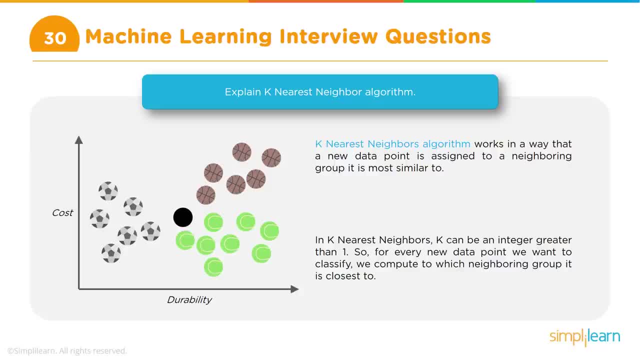 mention. Technically it can be even number also, but then typically it would be odd number and we will see why that is Okay. so, based on that, we need to classify objects. Okay, we need to classify objects. So, again, it will be very helpful to draw a. 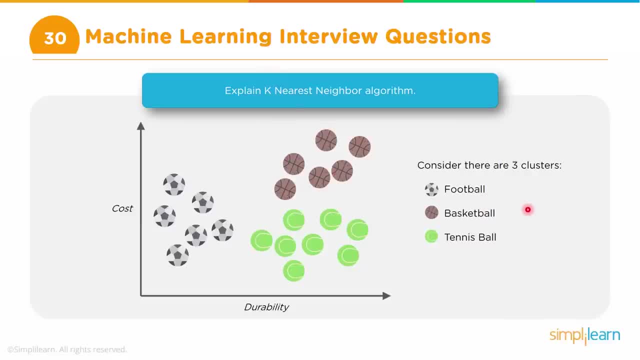 diagram. You know if you are explaining, I think that will be the best way. So draw some diagram like this: And let's say we have three clusters or three classes existing And now you want to find for a new item that has come. you want to find out which class this belongs to, right? So 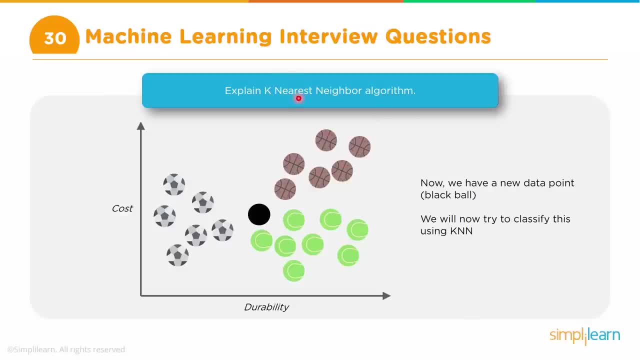 you go about, as the name suggests, you go about finding the nearest neighbors right, The points which are closest to this, And how many of them you will find. That is what is defined by k. Now, let's say, our initial value of k was: 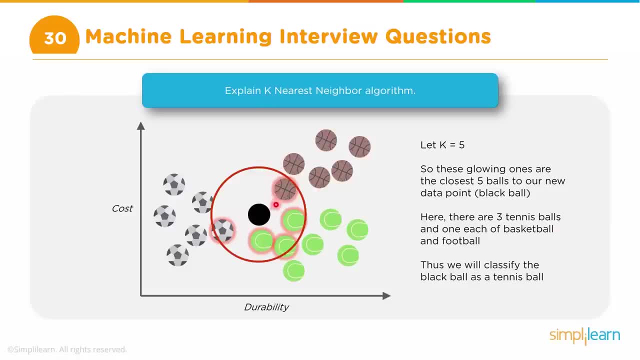 5. So you will find the k, the five nearest data points. So in this case, as it is illustrated, these are the five nearest data points, But then all five do not belong to the same class or cluster, So there are one belonging to this, cluster 1, the second one belonging to this: 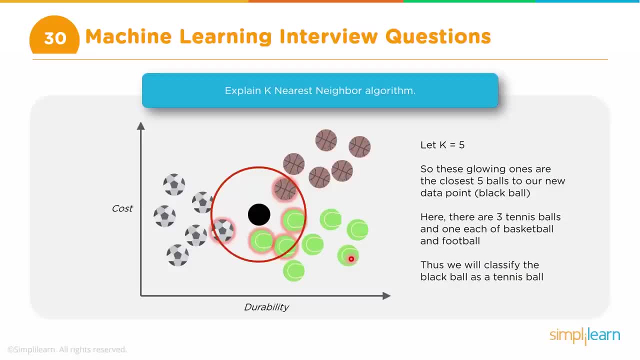 cluster 2,, three of them belonging to this third cluster. Okay, so how do you decide? That's exactly the reason we should, as much as possible, try to assign an odd number so that it doesn't go to the same cluster. So in this case, you see that the majority, actually, if there are, 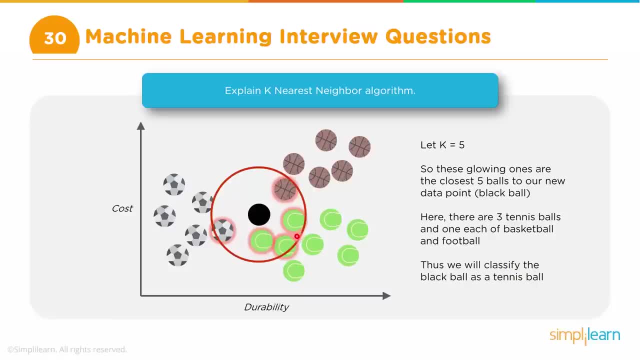 multiple classes, then you go with the majority. So, since three of these items belong to this class, we assign, which is basically the, in this case the green, or the tennis, or the third cluster, as I was talking about, right, So we assign it to this third class. So in this case it is. 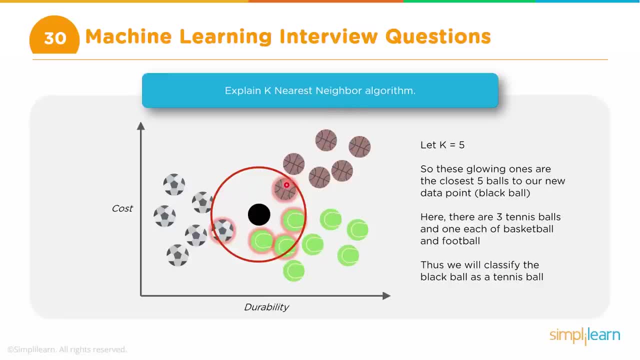 that's how it is decided. Okay, so k nearest neighbors. the first thing is to identify the number of neighbors that belong to this cluster. So in this case, we assign the number of neighbors that belong to this cluster. So, in this case, we assign the number of neighbors that belong to this. 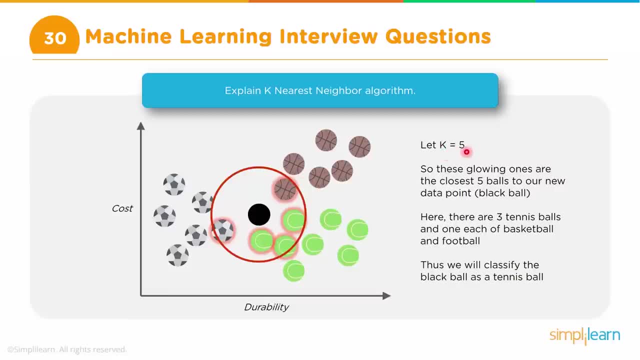 cluster. So in this case we assign the number of neighbors that are mentioned as k. So in this case it is: k is equal to five. So we find the five nearest points and then find out out of these five which class has the maximum number in that And then the new data point is assigned to that. 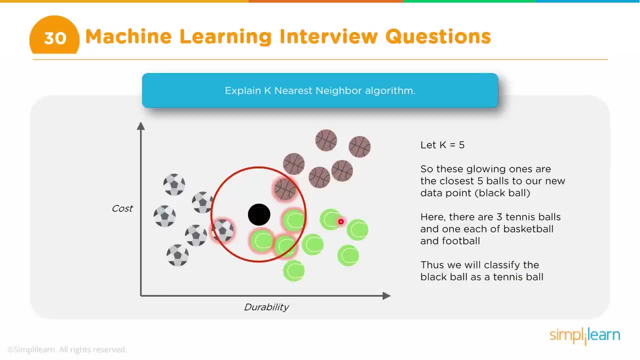 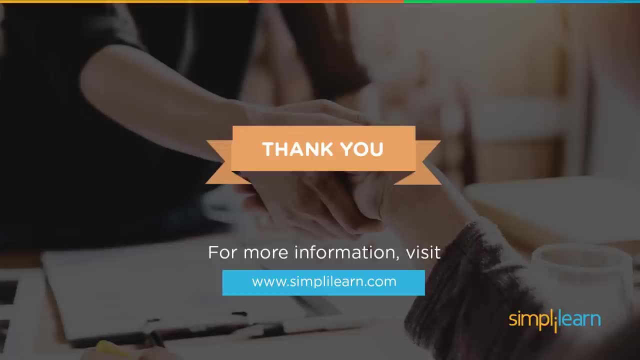 class. So that's pretty much how k nearest neighbors work. All right, So that brings us to the end of this module. I hope you enjoyed this interview questions and hope you will be able to crack your next interview if any of these questions come up.